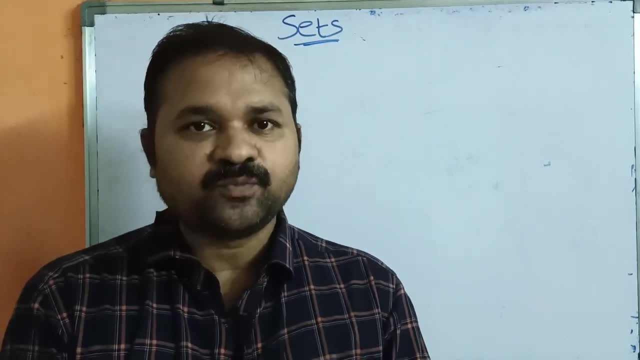 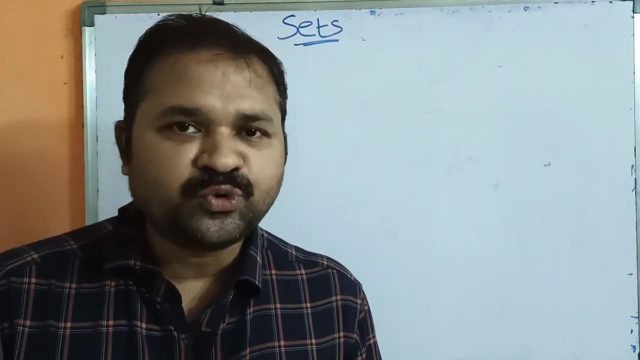 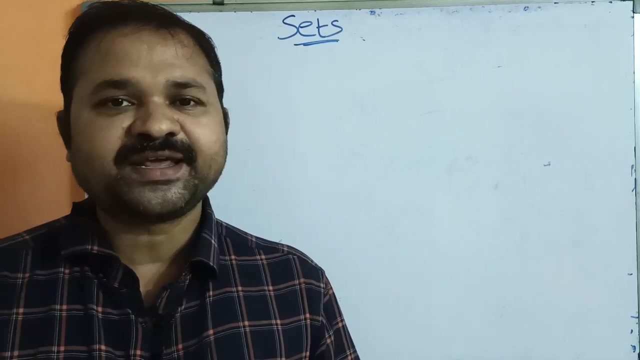 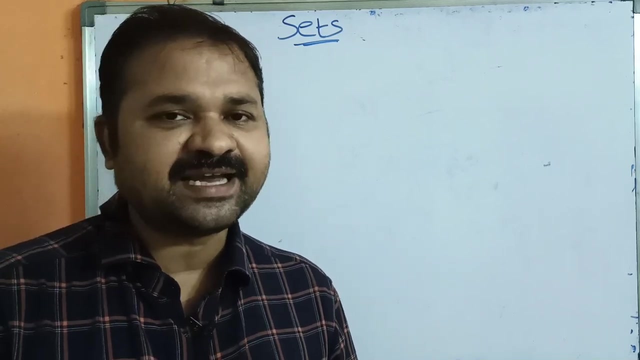 In this video, we are going to discuss about sets such as what is a set and how to denote a member or element. next, what is finite set? next, what is infinite set? what is single turn set, followed by set representation or set notations. We can represent set in two. 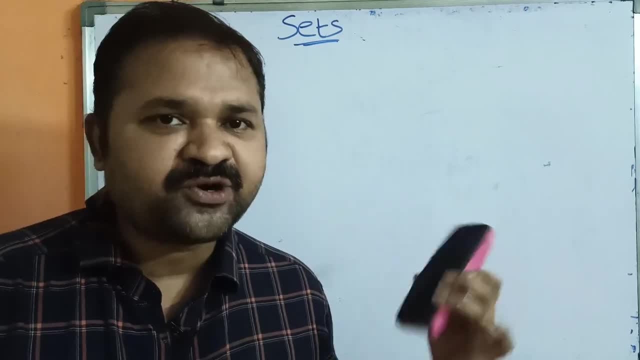 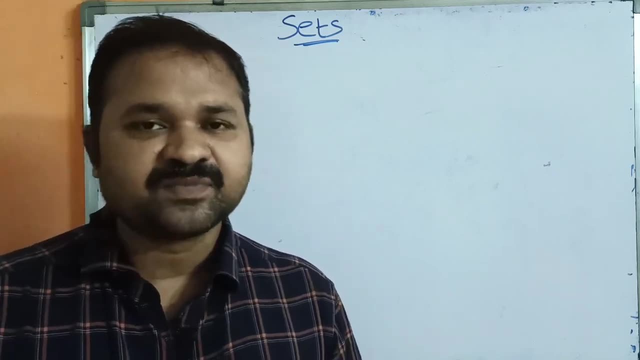 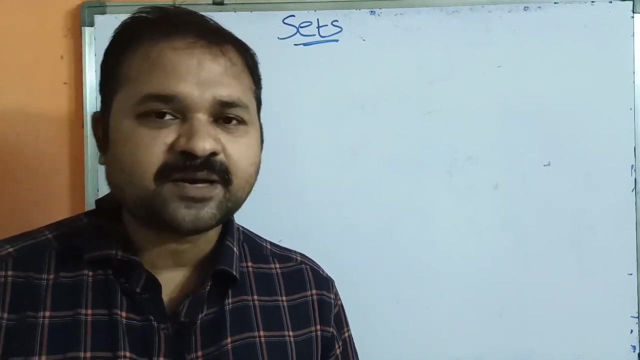 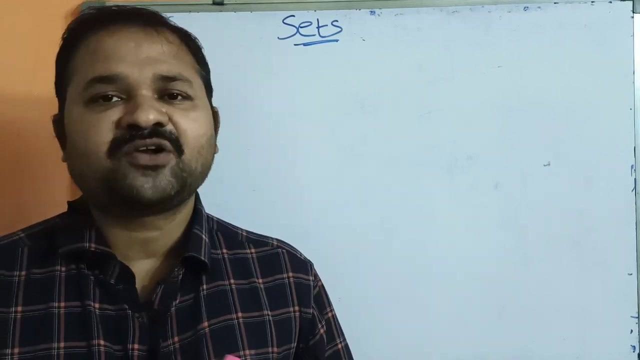 ways. First way is roster notation. second way is set builder notation, followed by various terminologies on the set, such as cardinality of the set, subset, equality of two sets, proper subset, universal set, next followed by null set or empty set, followed by operations. 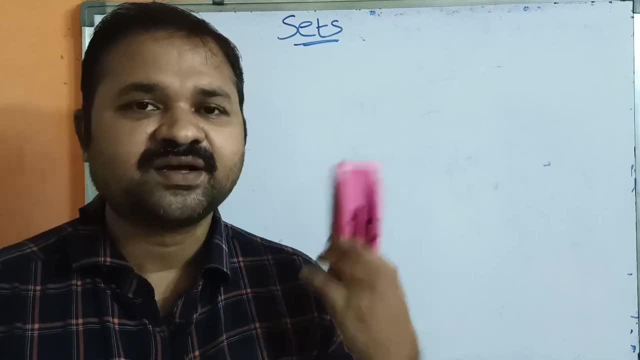 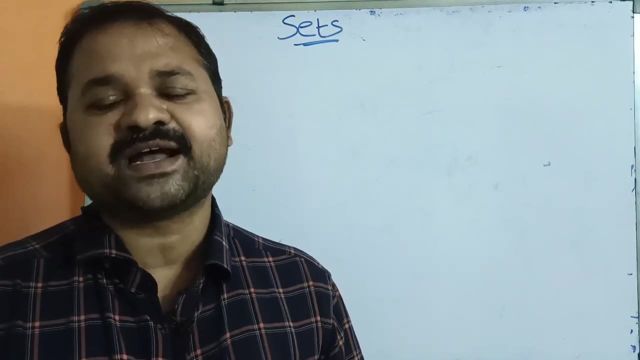 on the set, such as intersection, disjoint, universal set, finite set, finite set, finite union. next, difference, complement, symmetric difference, Cartesian product. Let us discuss all the topics on the sets in this video. First, let us see what is a set. Let us see: 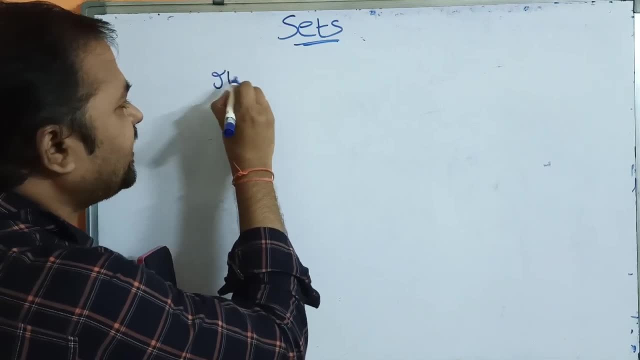 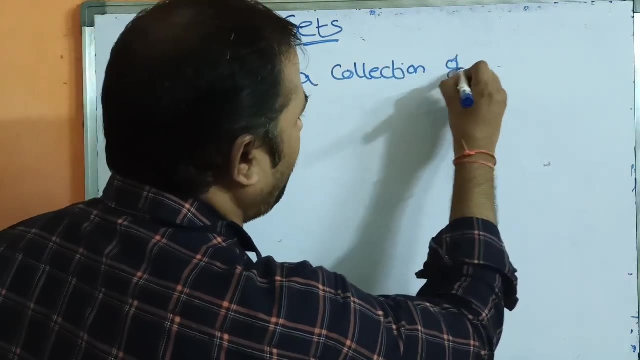 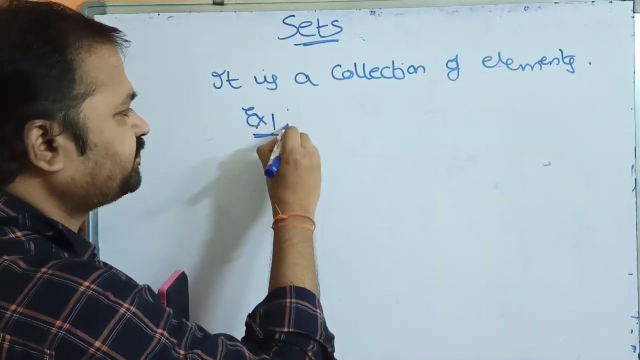 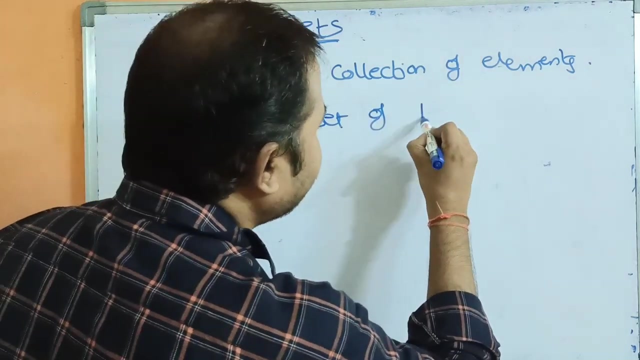 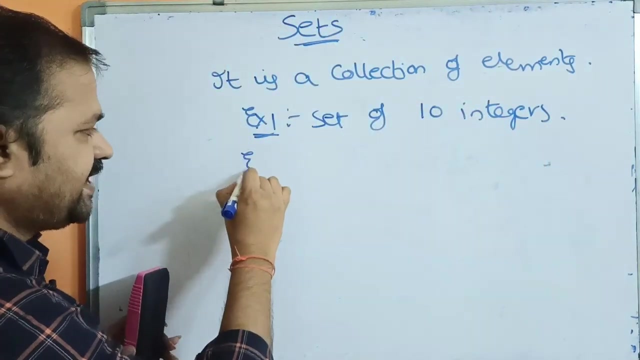 the definition for the set: Set means it is a collection of elements. So the definition for the set is: set is a collection of elements. Now let us take the example of the set. Let us take the example of the set: A set of 10 integers. So this is a set. So this set contains 10 integers. Example 2.. 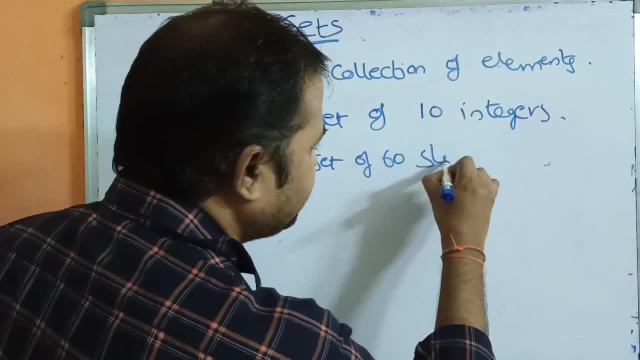 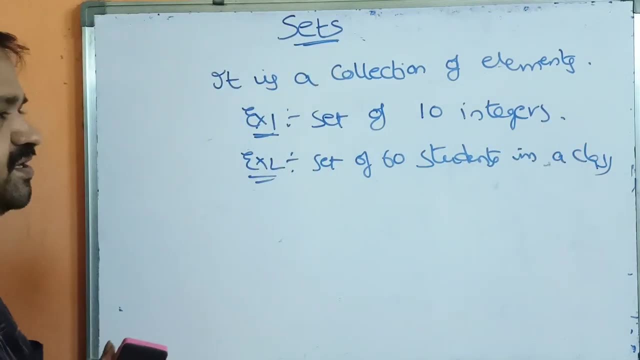 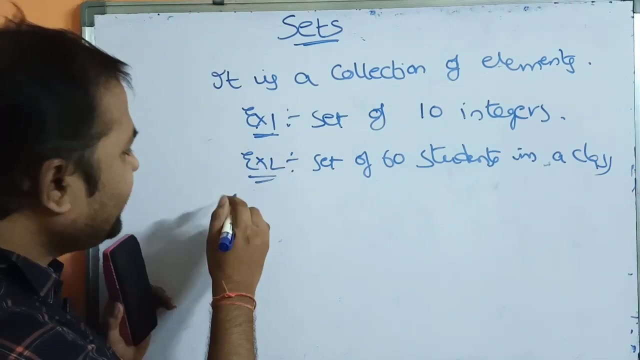 Set of 60 students in a class. So this is a set. This set contains totally 6 student information. So this is about what is a set And some examples For the set. Now let us see what is the element: How we can represent member or element of. 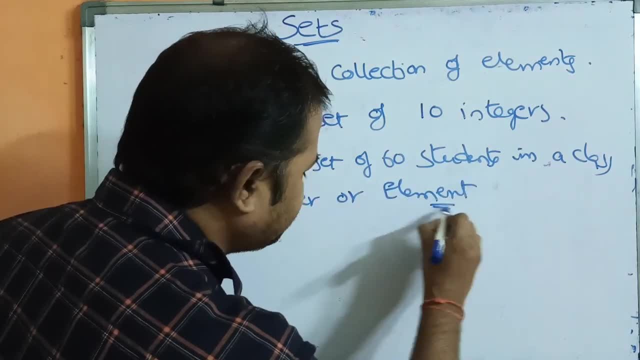 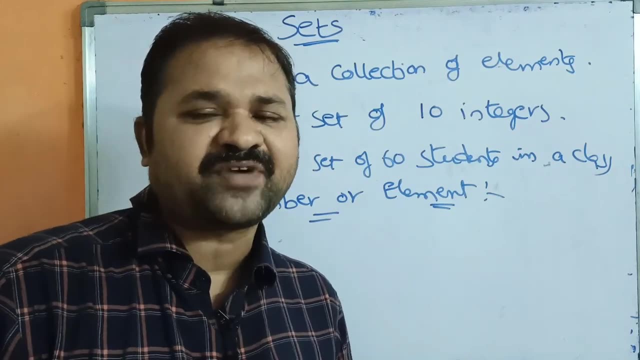 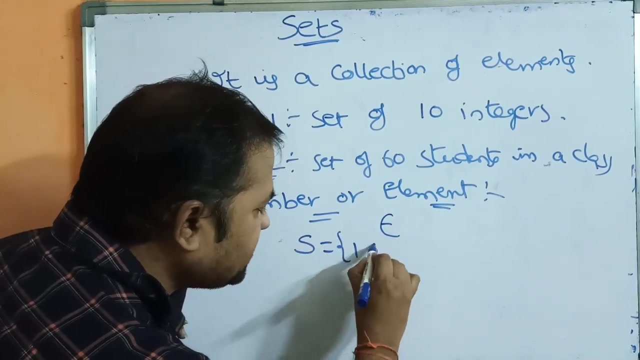 a set, Member or element of a set. Here we can represent a member or element with the help of epsilon symbol, So this symbol is called as epsilon symbol. Let we have a set called as. s is equal to 1 comma 2 comma 3.. 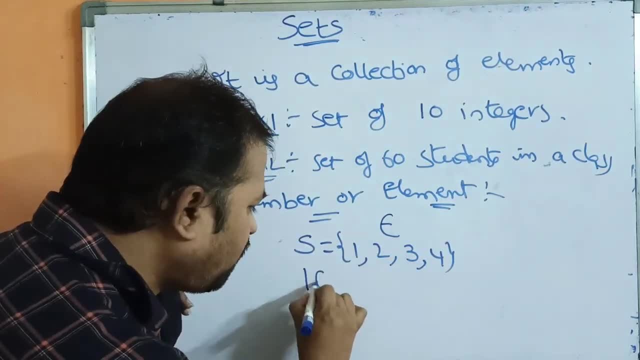 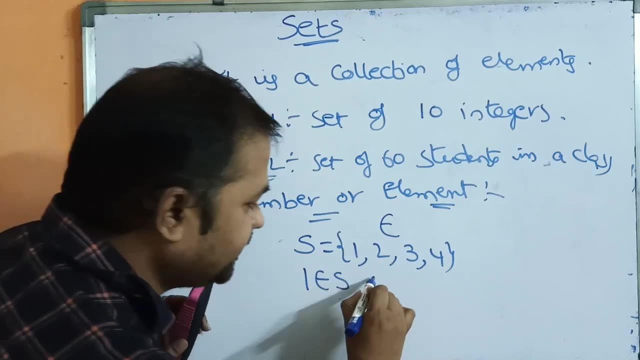 Members of the set are 1,, 2,, 3, 4.. So we can say that 1 belongs to s. That means 1 is a member of the set. That is, 1 is an element of the set. Likewise, we can say that 2 belongs. 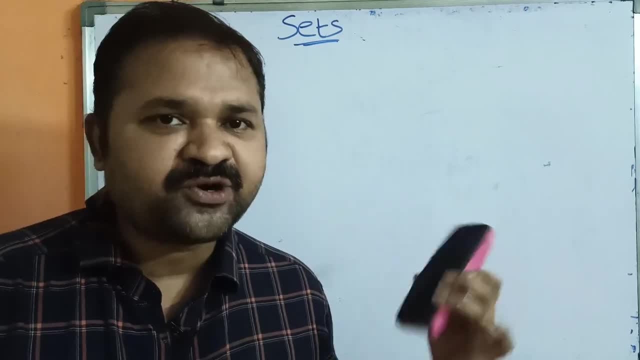 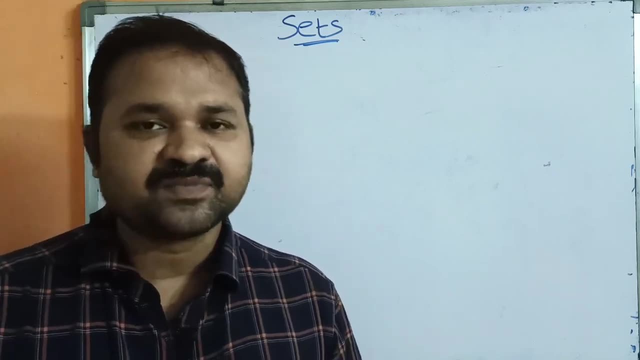 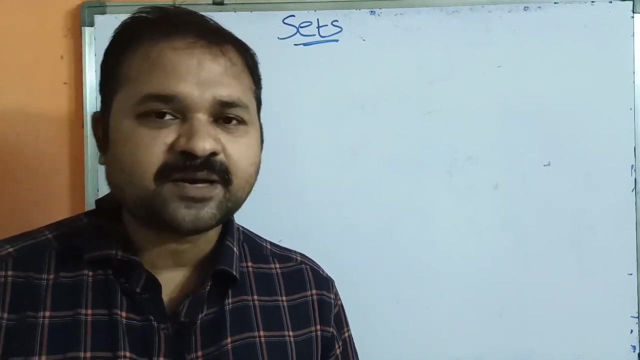 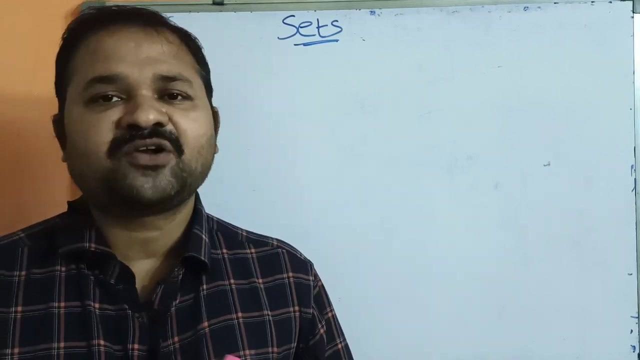 ways. First way is roster notation. second way is set builder notation, followed by various terminologies on the set, such as cardinality of the set, subset, equality of two sets, proper subset, universal set, next followed by null set or empty set, followed by operations. 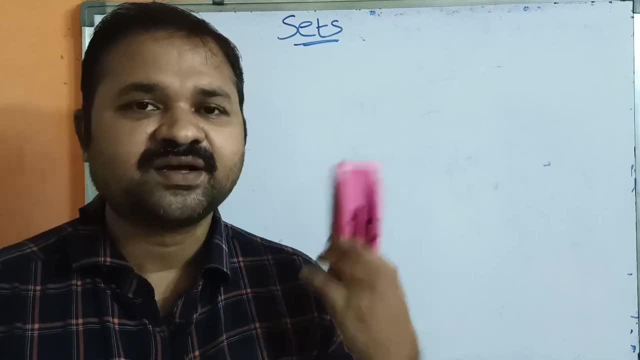 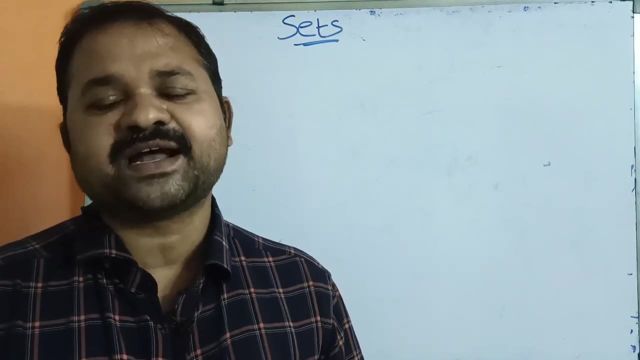 on the set, such as intersection, disjoint, universal set, finite set, finite set, finite union. next, difference, complement, symmetric difference, Cartesian product. Let us discuss all the topics on the sets in this video. First, let us see what is a set. Let us see: 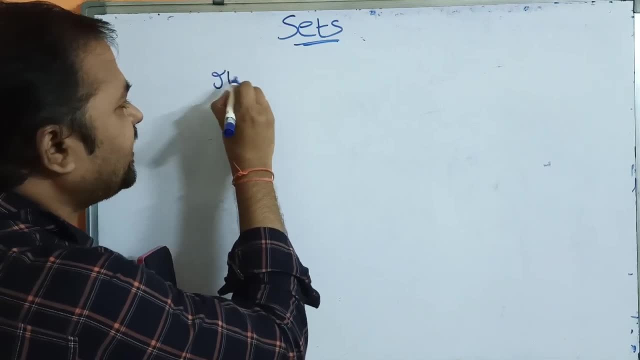 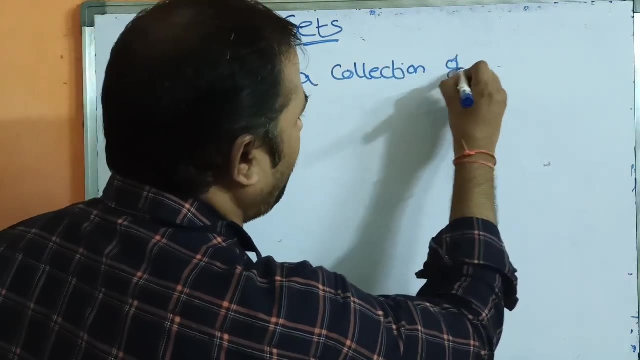 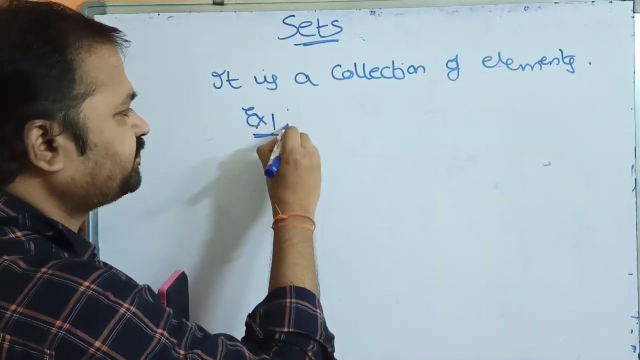 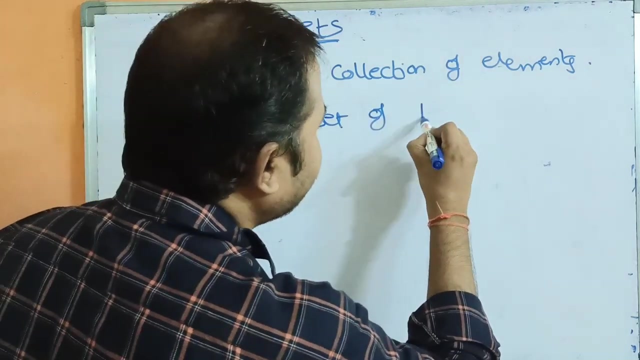 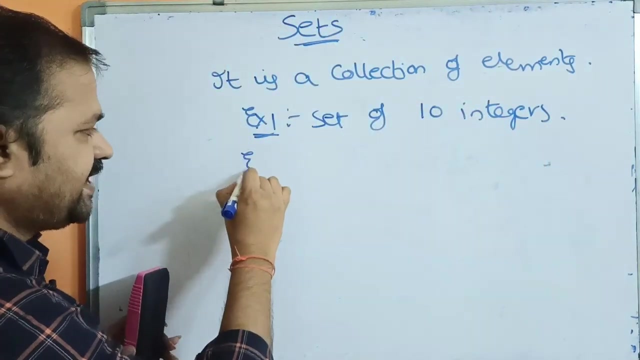 the definition for the set: Set means it is a collection of elements. So the definition for the set is: set is a collection of elements. Now let us take the example of the set. Let us take the example of the set: A set of 10 integers. So this is a set. So this set contains 10 integers. Example 2.. 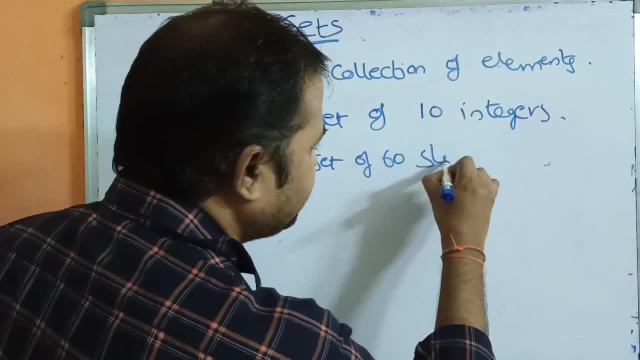 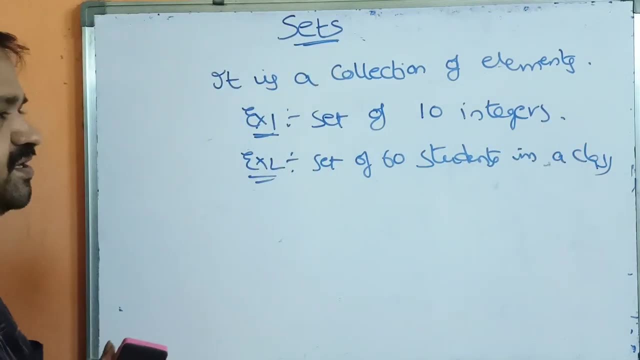 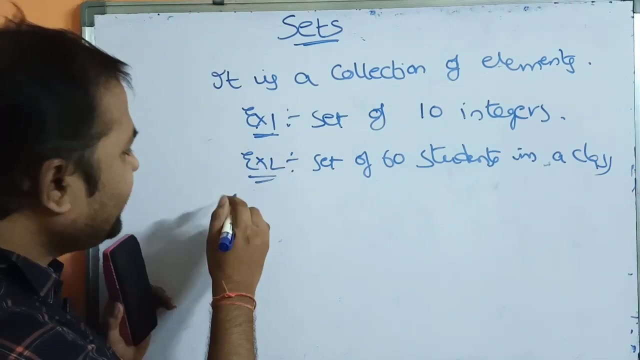 Set of 60 students in a class. So this is a set. This set contains totally 6 student information. So this is about what is a set And some examples For the set. Now let us see what is the element: How we can represent member or element of. 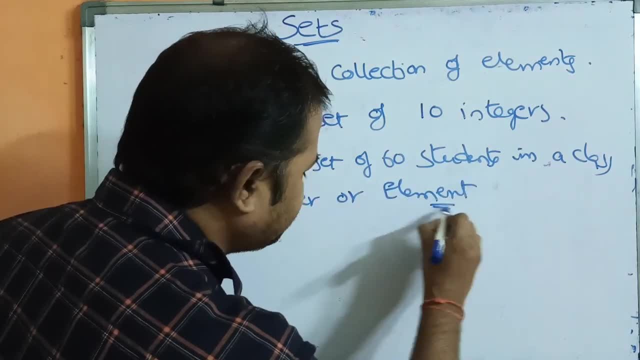 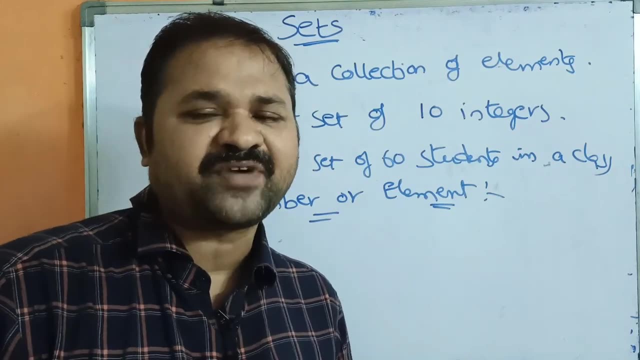 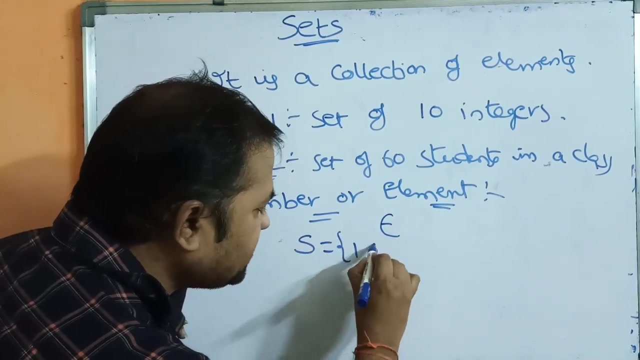 a set, Member or element of a set. Here we can represent a member or element with the help of epsilon symbol, So this symbol is called as epsilon symbol. Let we have a set called as. s is equal to 1 comma 2 comma 3.. 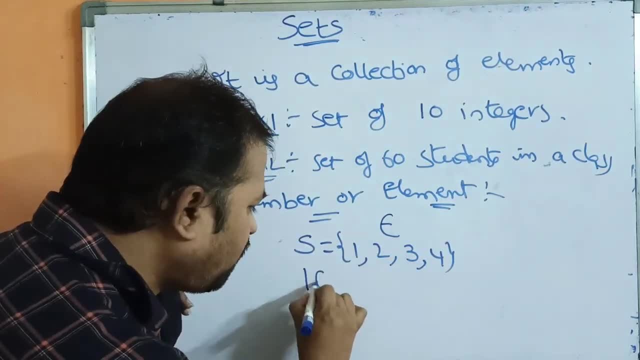 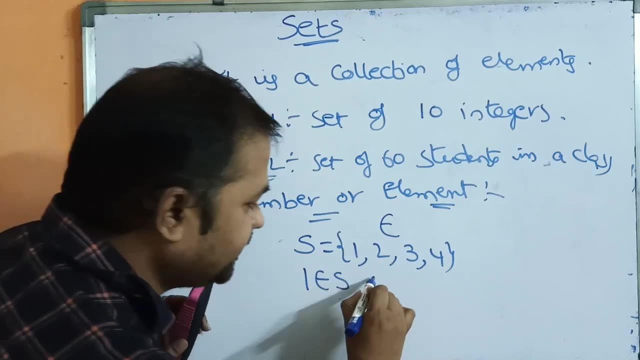 Members of the set are 1,, 2,, 3, 4.. So we can say that 1 belongs to s. That means 1 is a member of the set. That is, 1 is an element of the set. Likewise, we can say that 2 belongs. 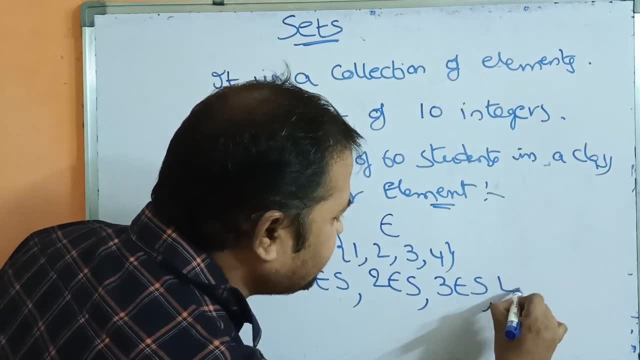 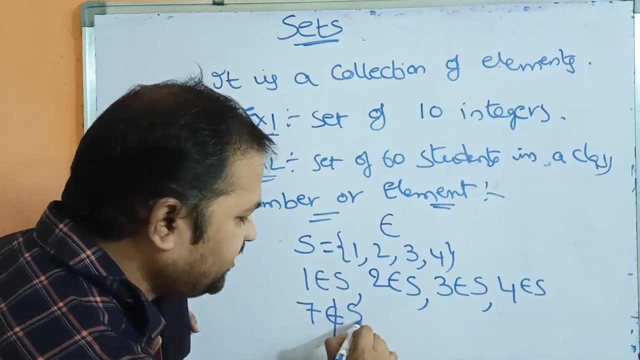 to s. 2 is a member of the set. 3 is a member of the set. 4 is a member of the set. Let us take 7.. 7 is not a member of the set. Then we use this symbol: Doesn't belongs to Some. 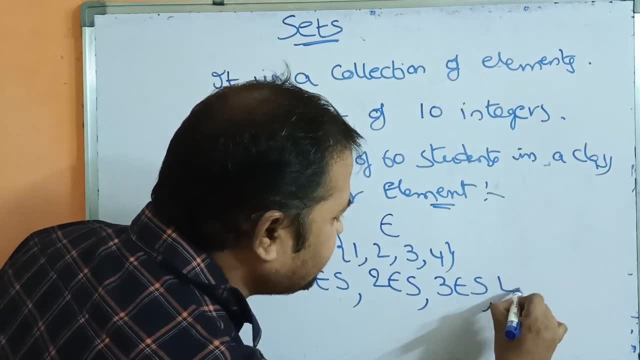 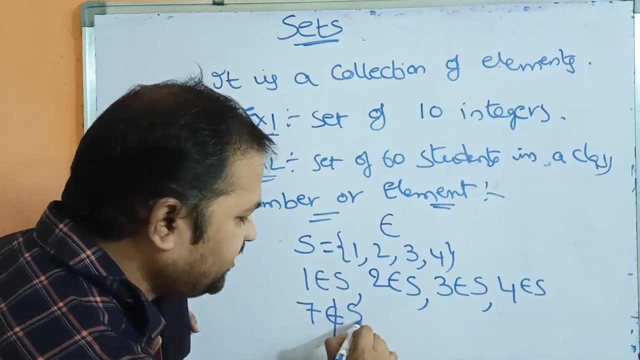 to s. 2 is a member of the set. 3 is a member of the set. 4 is a member of the set. Let us take 7.. 7 is not a member of the set. Then we use this symbol: Doesn't belongs to Some. 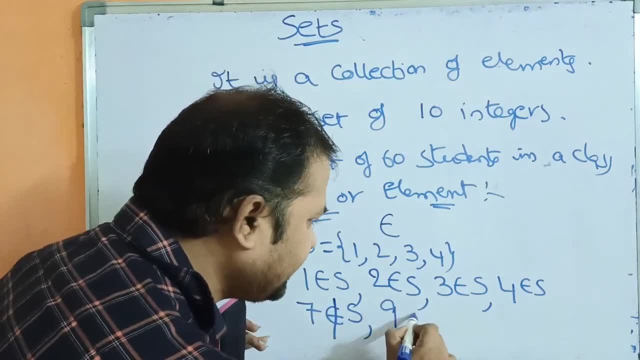 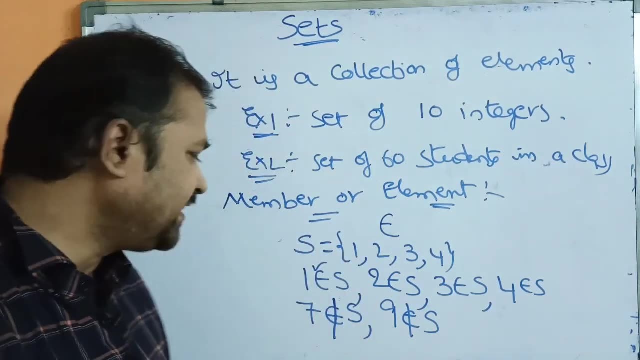 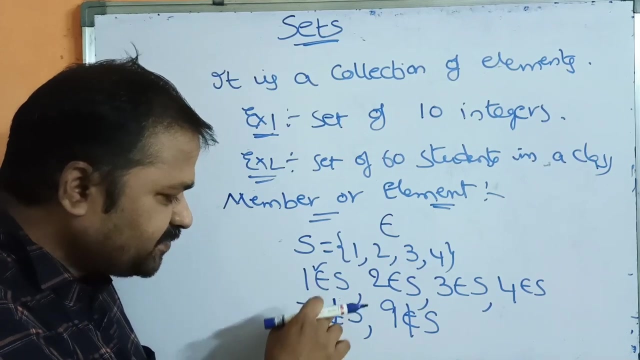 epsilon and some a line like this: Ok, Let us take 9.. So 9 is a member of the set. So 9 doesn't belong to set, Ok, So here epsilon symbol is used to denote that it is a member of the set. The element is a member of the set, Whereas this doesn't belongs to, Doesn't? 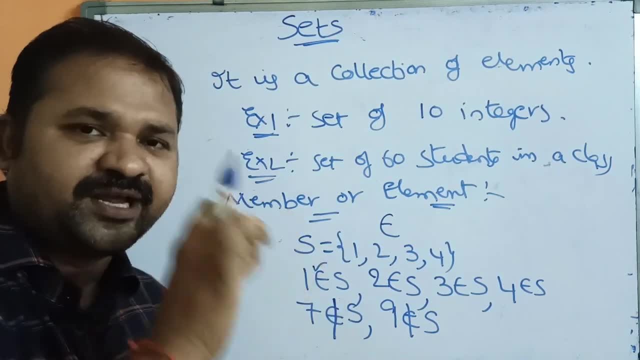 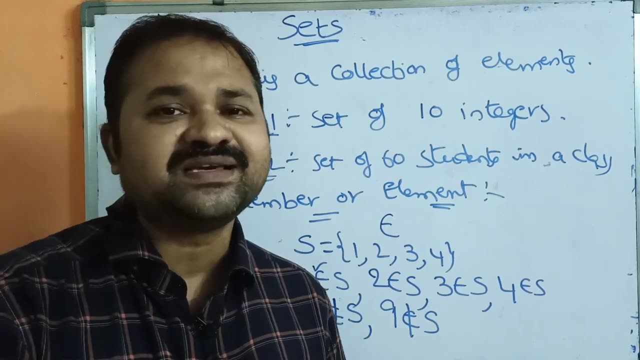 epsilon- Ok, Epsilon cross mark. This symbol is used to denote that that element is not a member of the set. Generally, we can denote set by using capital letters, So we can denote set with the help of capital letters, Such as capital A. 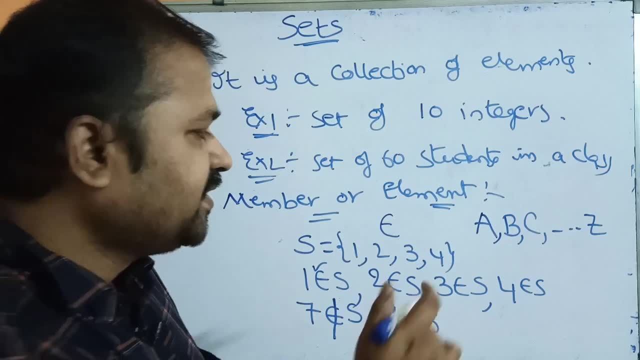 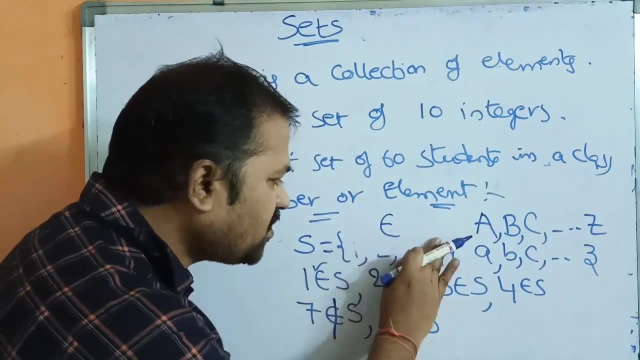 Capital B, Capital C, So on capital Z, Whereas we can use lower case letter in order to represent the elements of the set. So here, in place of 1,, 2,, 3, 4, we can write small, a small. 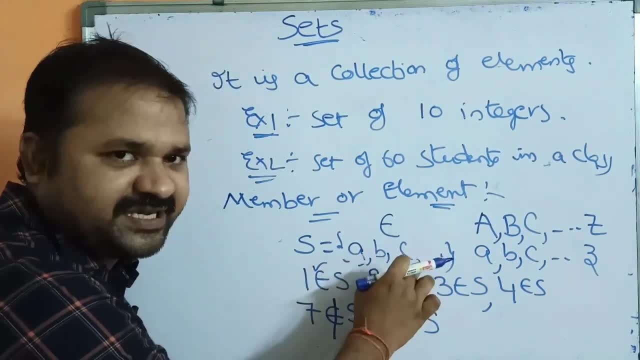 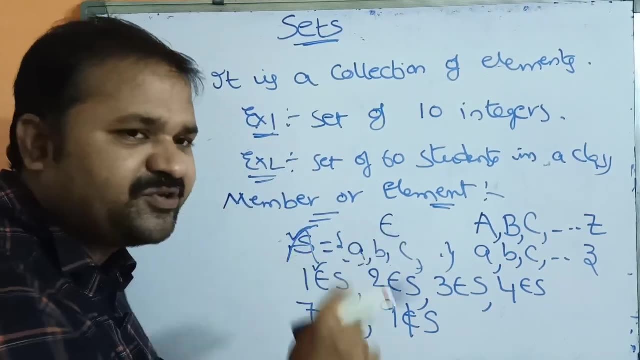 b, small c also. Ok, But we can't write capital letters here. Why? because we use capital letters for denoting a set. So capital S is equal to abc, Capital A is equal to abc, So likewise we can denote the set. Now let us see about what is finite set. 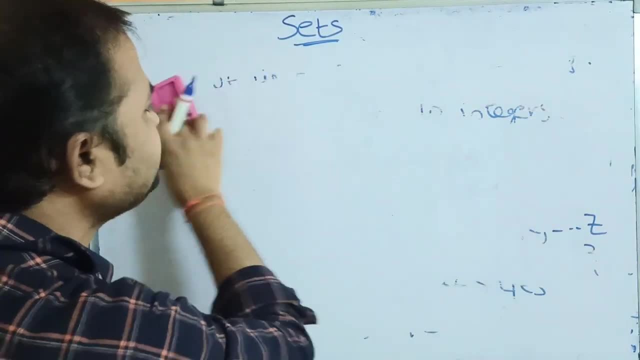 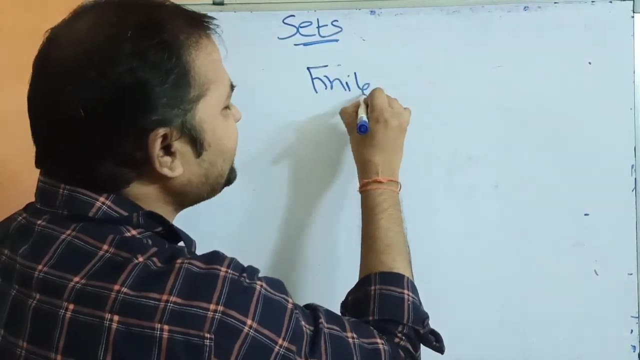 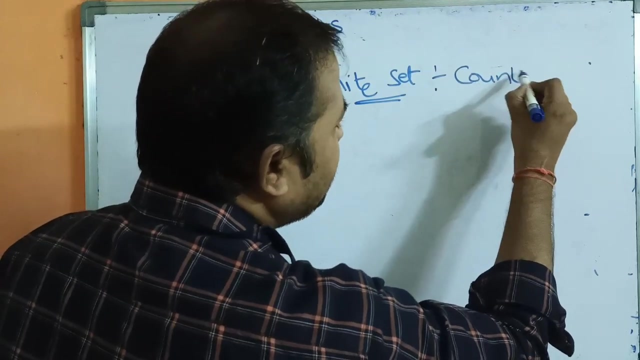 What is infinite set and what is singleton set? First let us see about what is finite set. The name itself specifies the meaning. So finite set means if the set contains a finite number of elements. So finite number of elements means if the set contains a countable. 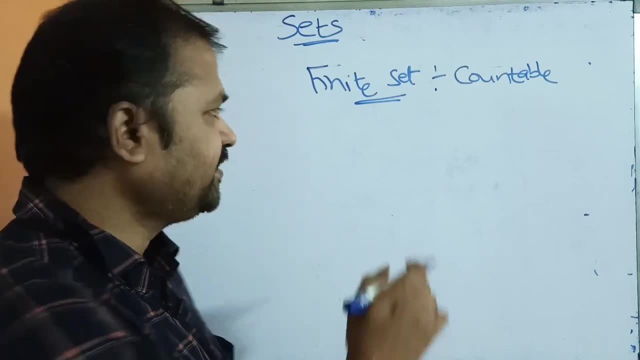 number of elements. Then it is called as finite set. Ok, So let we have a set like this, A set of odd numbers from 1 to 10.. So 1,, 3,, 5,, 7,, 9.. 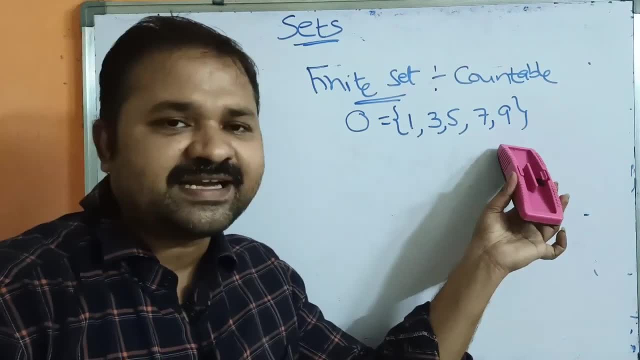 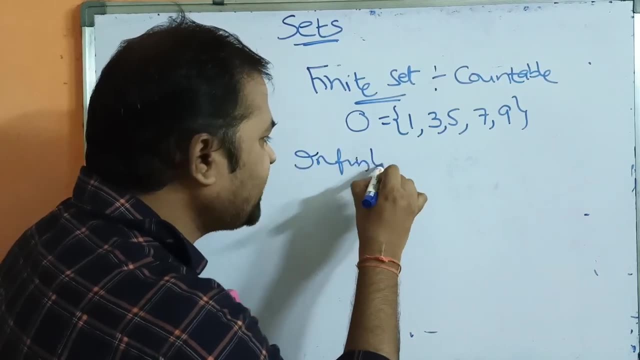 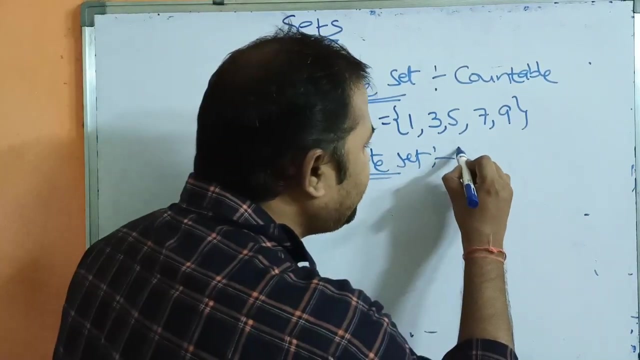 Ok, So this is nothing but a finite set. This set contains only 5 elements. Ok, Let us take a series like this Infinite set. Now let us see about infinite set. Infinite set means the set contains infinite number of elements. Infinite number of elements means the set. 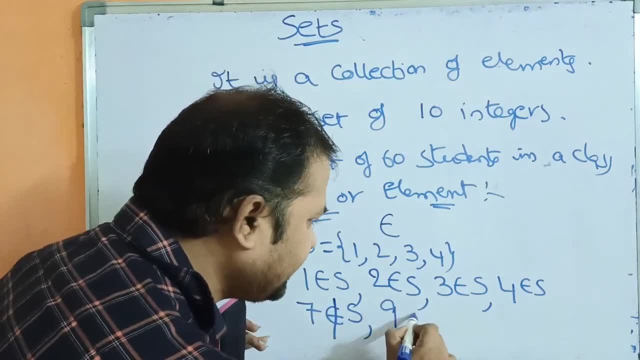 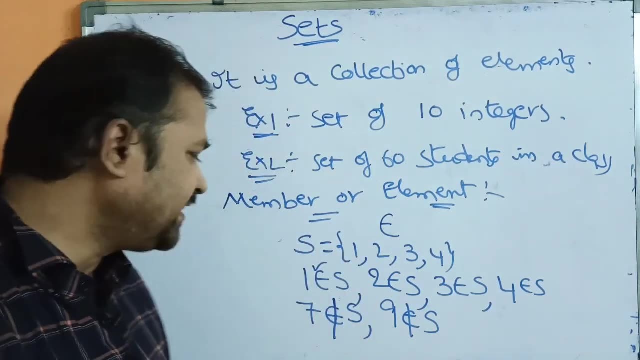 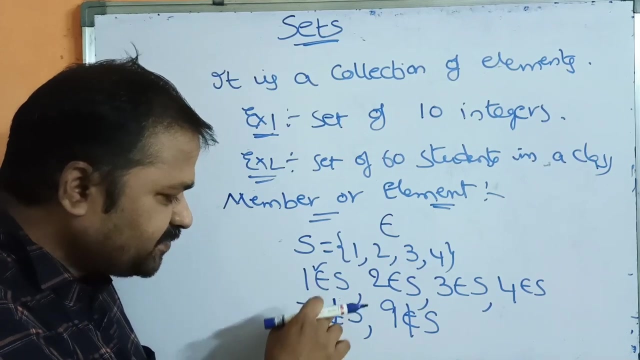 epsilon and some a line like this: Ok, Let us take 9.. So 9 is a member of the set. So 9 doesn't belong to set, Ok, So here epsilon symbol is used to denote that it is a member of the set. The element is a member of the set, Whereas this doesn't belongs to, Doesn't? 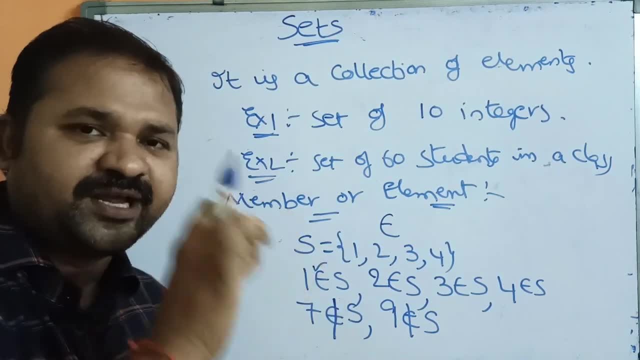 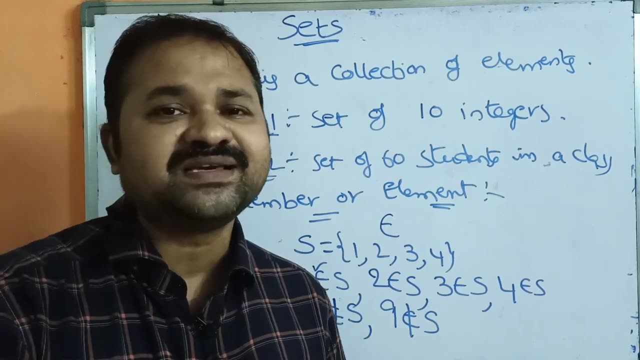 epsilon- Ok, Epsilon cross mark. This symbol is used to denote that that element is not a member of the set. Generally, we can denote set by using capital letters, So we can denote set with the help of capital letters, Such as capital A. 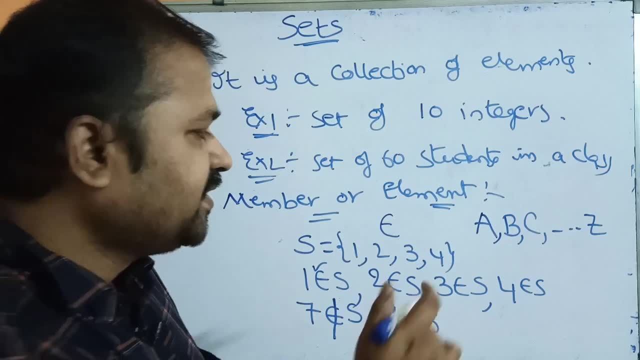 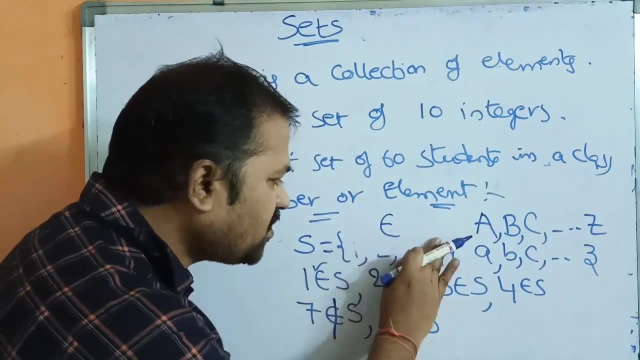 Capital B, Capital C, So on capital Z, Whereas we can use lower case letter in order to represent the elements of the set. So here, in place of 1,, 2,, 3, 4, we can write small, a small. 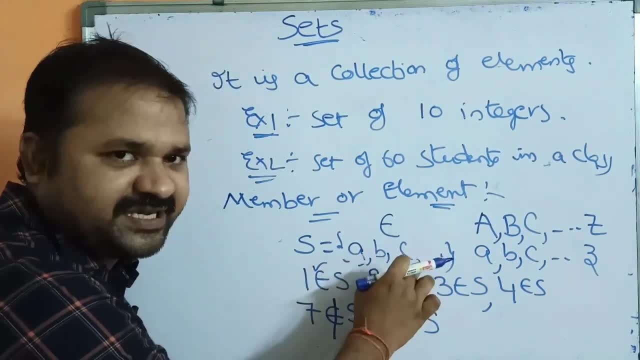 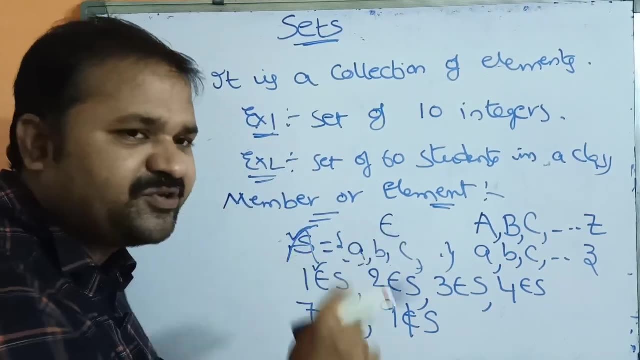 b, small c also. Ok, But we can't write capital letters here. Why? because we use capital letters for denoting a set. So capital S is equal to abc, Capital A is equal to abc, So likewise we can denote the set. Now let us see about what is finite set. 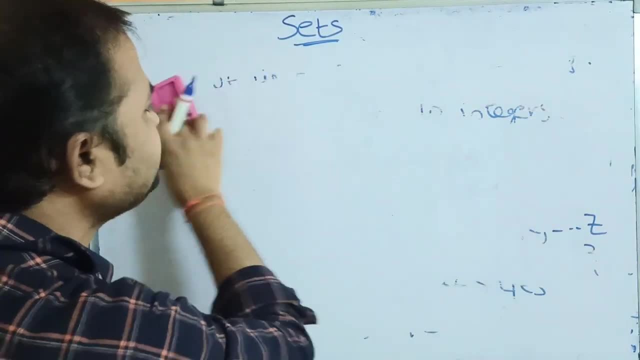 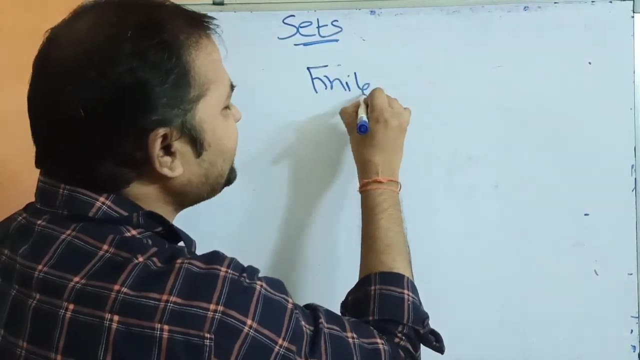 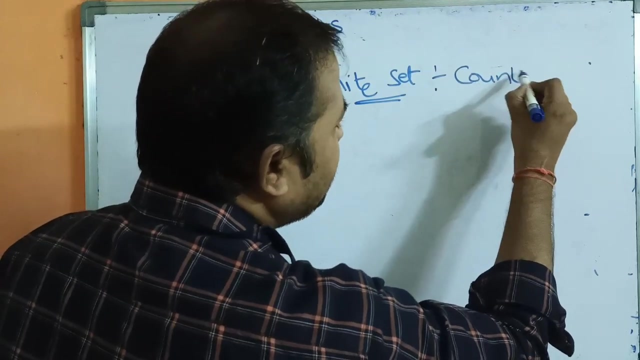 What is infinite set and what is singleton set? First let us see about what is finite set. The name itself specifies the meaning. So finite set means if the set contains a finite number of elements. So finite number of elements means if the set contains a countable. 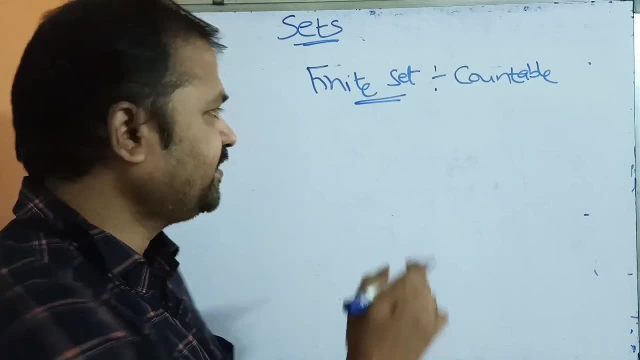 number of elements. Then it is called as finite set. Ok, So let we have a set like this, A set of odd numbers from 1 to 10.. So 1,, 3,, 5,, 7,, 9.. 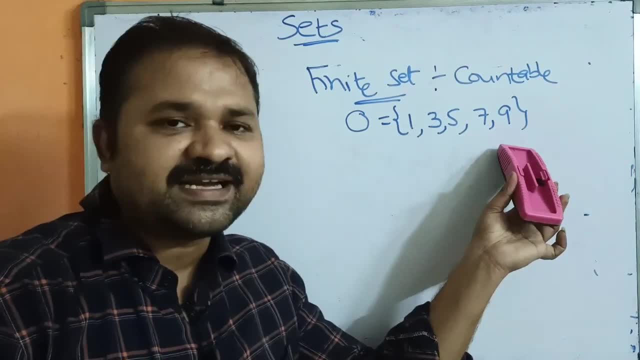 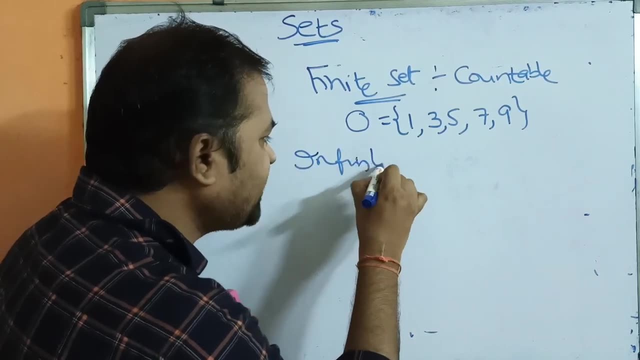 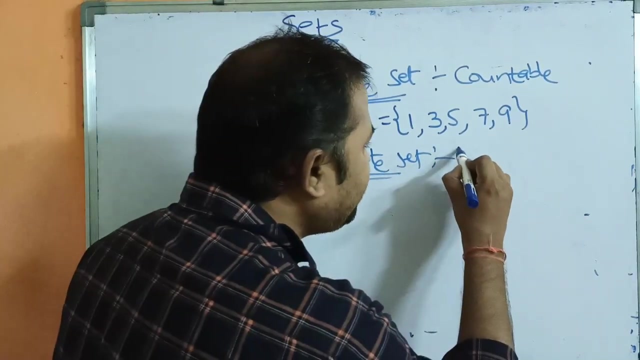 Ok, So this is nothing but a finite set. This set contains only 5 elements. Ok, Let us take a series like this Infinite set. Now let us see about infinite set. Infinite set means the set contains infinite number of elements. Infinite number of elements means the set. 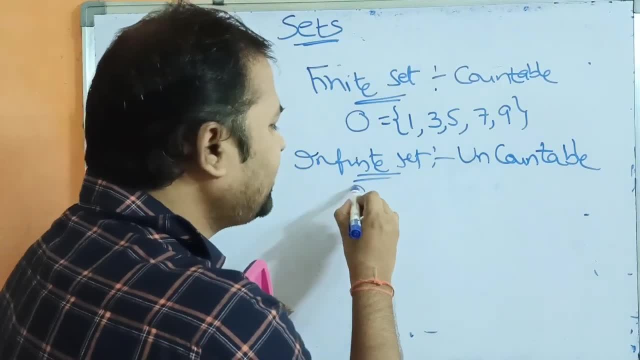 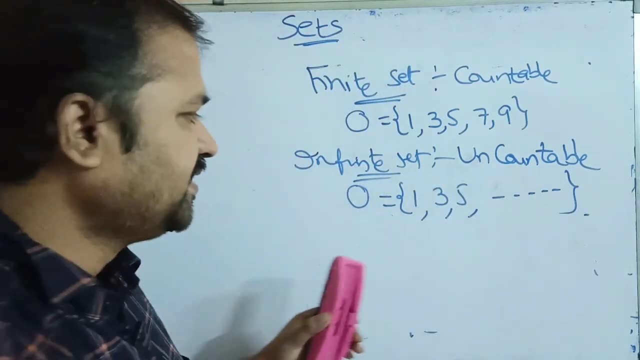 contains uncountable number of elements. So let we have a set like this: O is equal to 1 comma, 3 comma, 5 comma, so on Some series like this here we don't know what is the final term. we don't know the final term here. 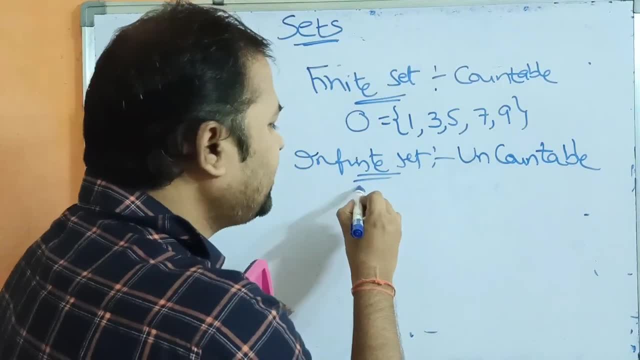 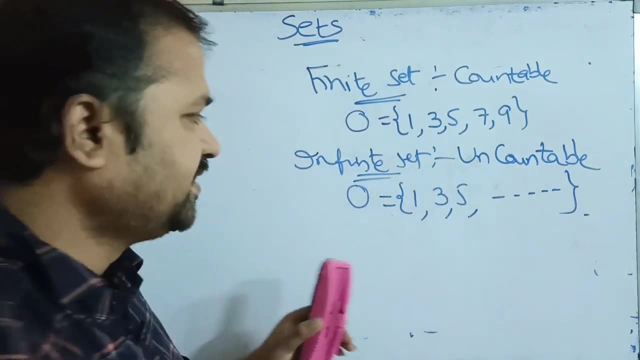 contains uncountable number of elements. So let we have a set like this: O is equal to 1,, 3,, 5, so on, Some series like this. So let us take a series like this: O is equal this Here. we don't know what is the final term. We don't know the final term here. So this is: 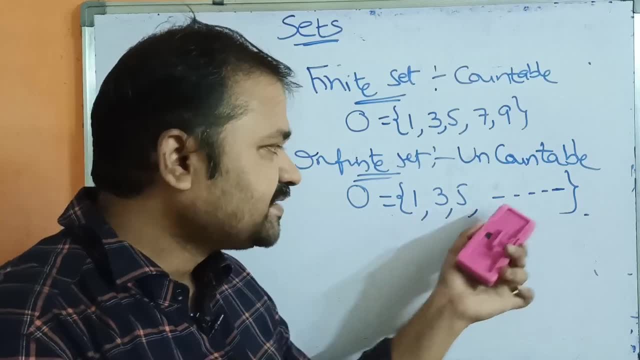 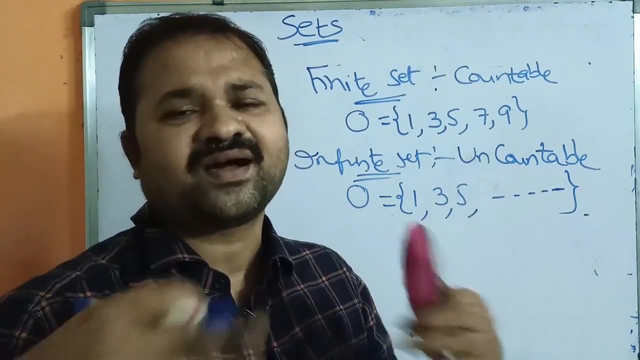 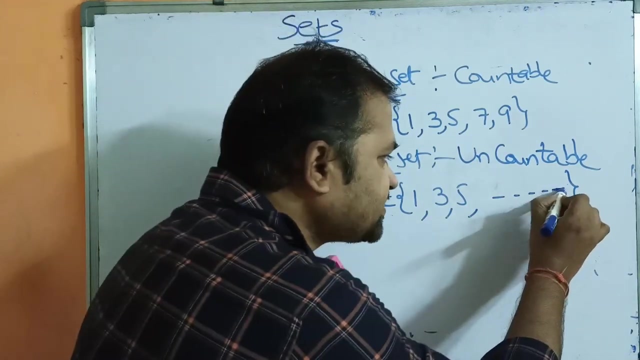 called as infinite set. Infinite set means the set contains infinite number of elements. Here we don't know what is the final term: 100 or 200, or 1 lakh or 2 lakh or 3 lakh? We don't know what is that number. So that's why this is called as infinite set. Infinite set means we don't know. 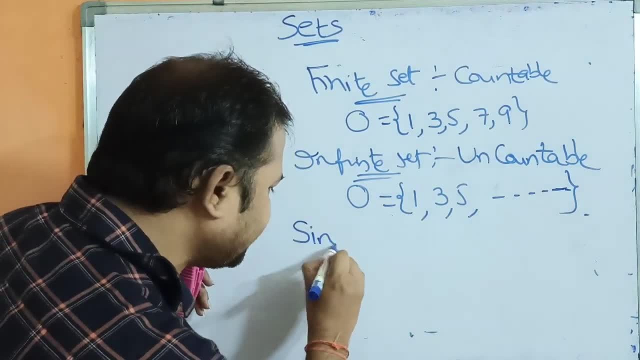 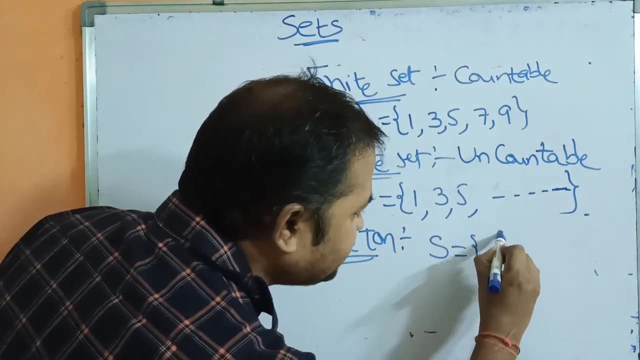 what is the final value? Now let us see about singleton set. Singleton- the name itself specifies the meaning. If the set contains only one element, then it is called as singleton set. If you consider this example here, the set contains only one element, So that's why this is called as. 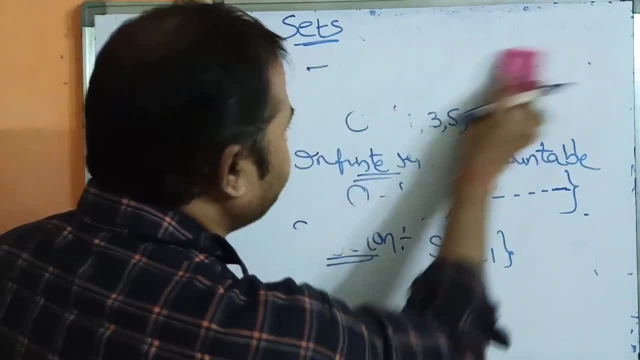 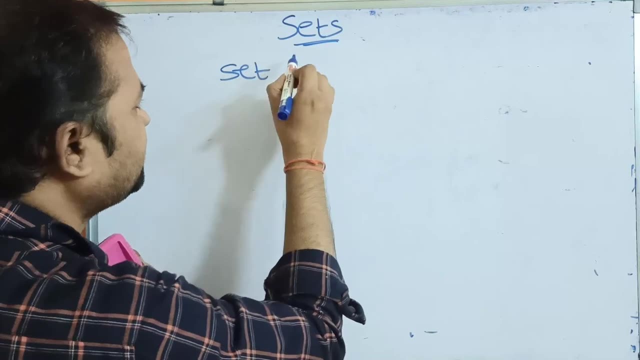 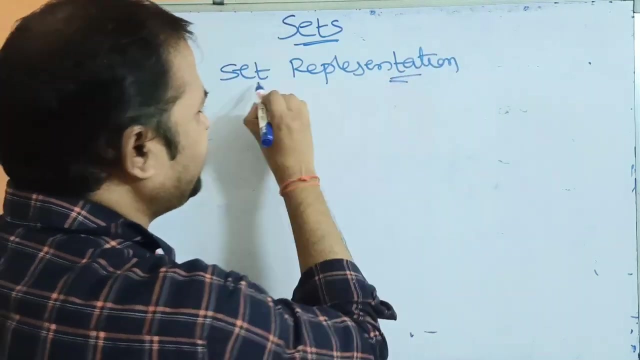 singleton set. Now let us see the next concept, That is, set representation. This is very, very important concept. So set representation, Set representation Or set notations, Set representation Representations Or set notations Or set notations. 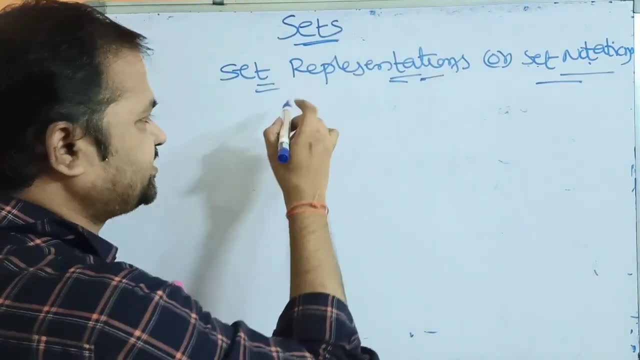 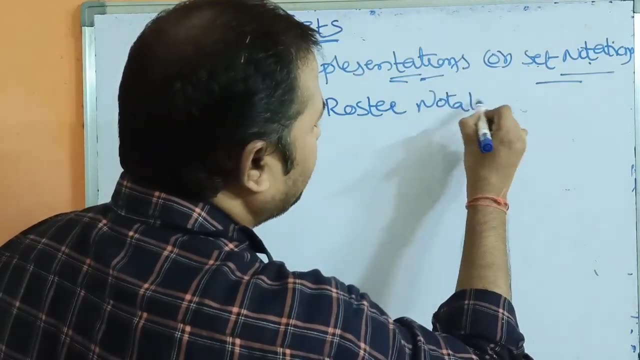 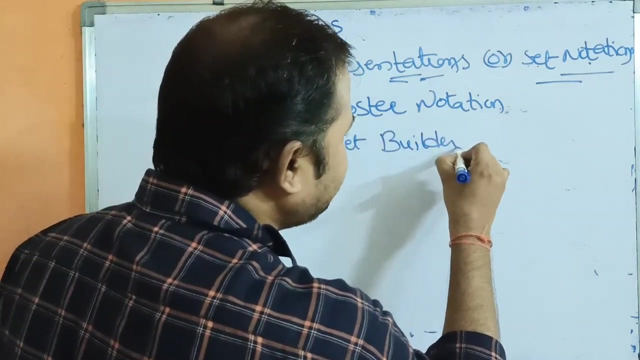 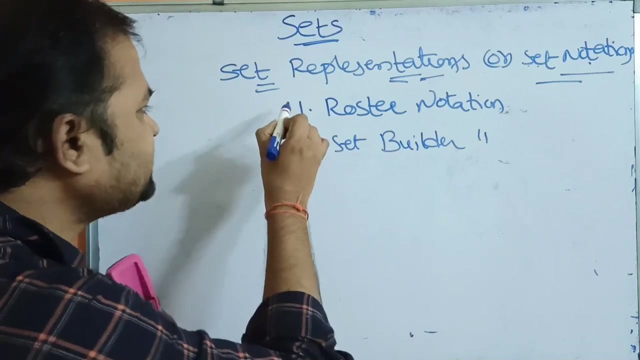 We can represent set in two notations. The first notation is: we can use roaster notation, Roaster notation. And the second approach is we can use set builder notation. So we can represent sets in two notations ways. first way is roaster notation, second way is set builder notation. first let us see about 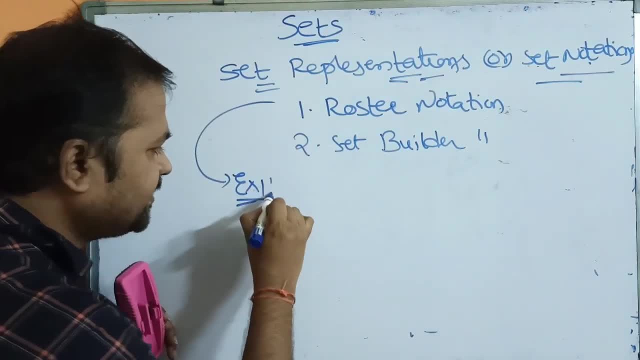 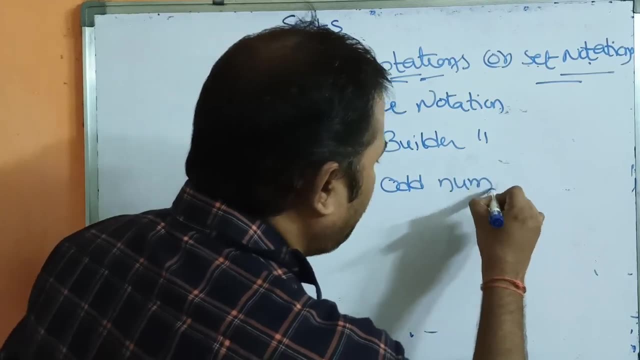 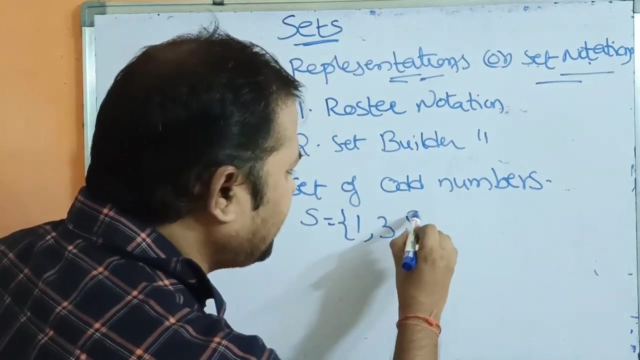 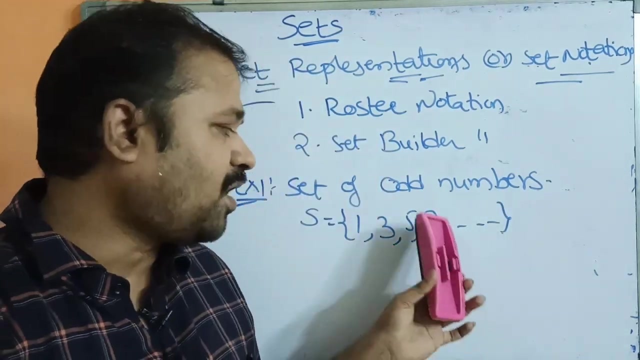 roaster notation. let us take an example, okay. set of set of odd numbers. set of odd numbers: okay, odd numbers. s is equal to, within the curly braces, one comma, three comma, five comma, seven, so on. okay, roaster notation means here the elements or the members of the set. 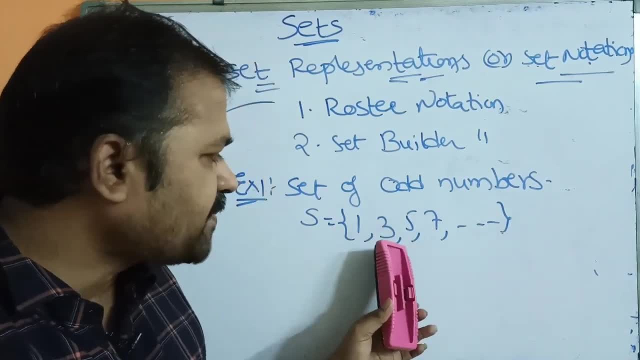 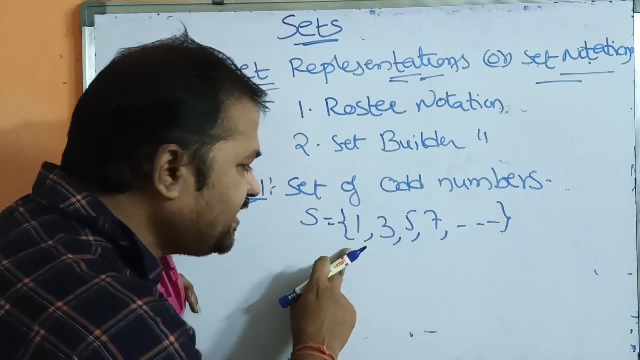 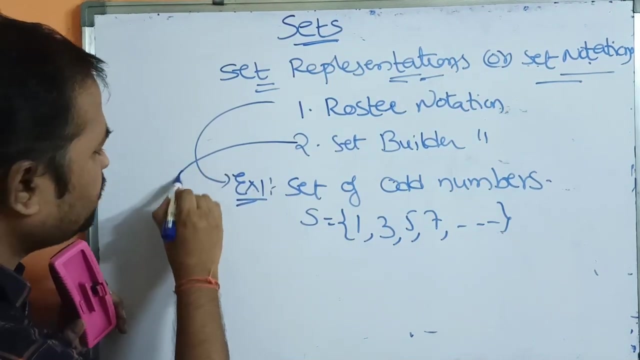 must be enclosed in curly braces and they are separated by comma symbol. okay, this is called as roaster notation. the elements must be enclosed in the curly braces and they are separated by comma symbol. now let us see the second approach. second approach: what is the second approach? 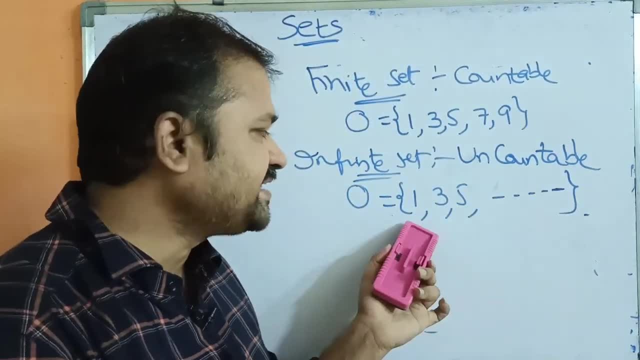 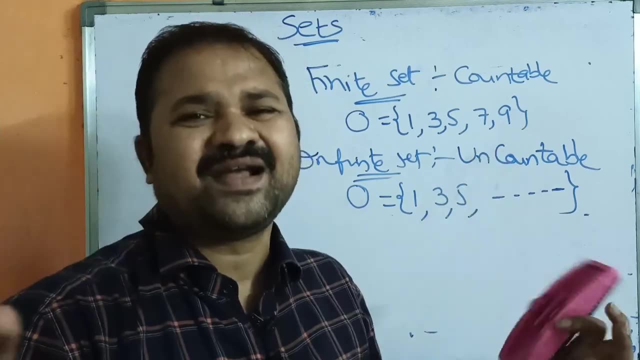 so this is called as infinite set. okay, infinite set means the set contains infinite number of elements. here we don't know what is the final term: 100 or 200 or 1 lakh, or 2 lakh or 3 lakh. we don't know what is that number. okay, so 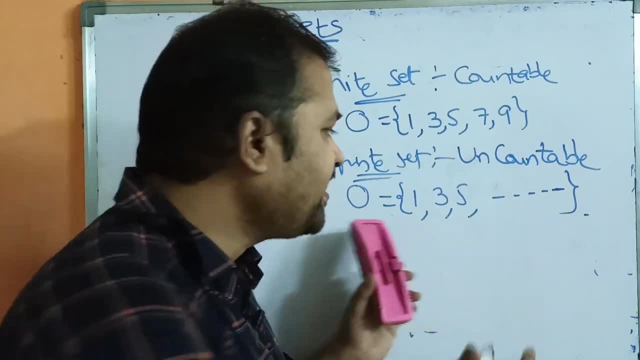 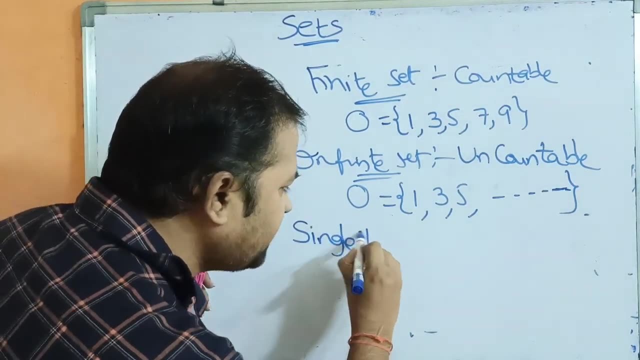 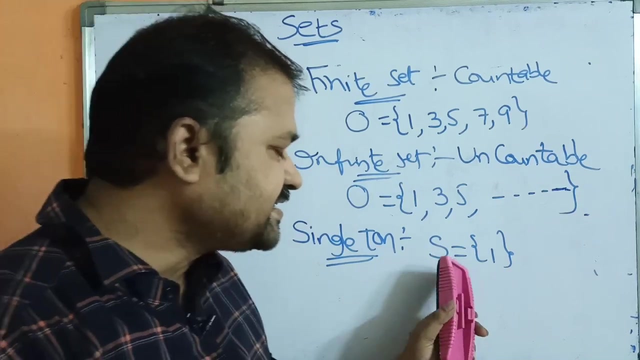 that's why this is called as infinite name, infinite set. infinite set means we don't know what is the final value. now let us see about singleton set. singleton- the name itself specifies the meaning. if the set contains only one element, then it is called a singleton set. if you consider this example here, the set. 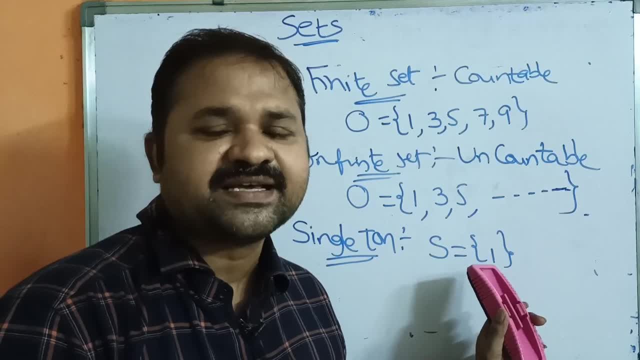 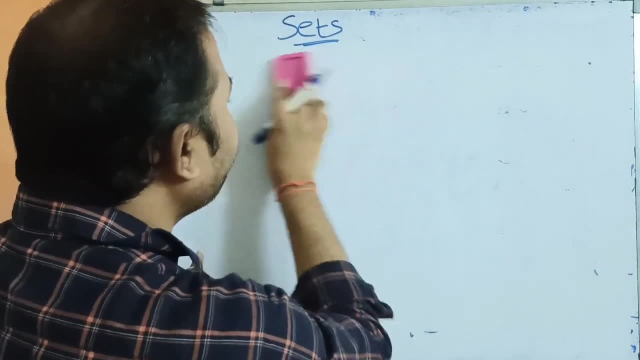 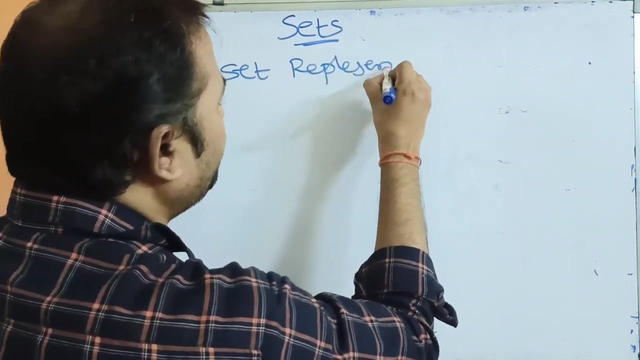 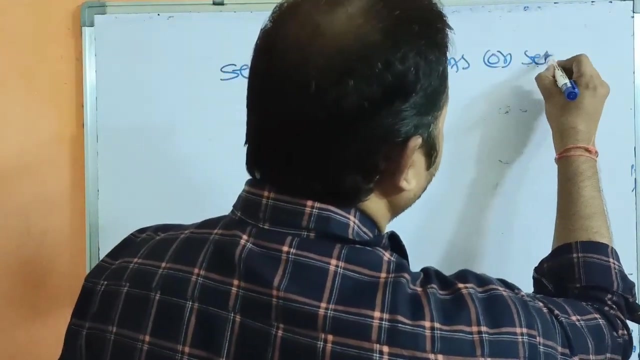 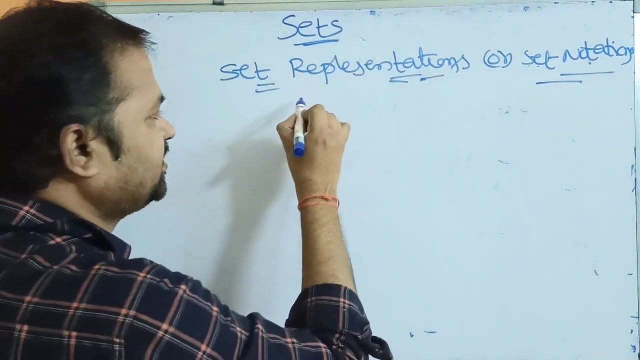 contains only one element, so that's why this is called as singleton set. now let us see the next concept, that is, set representation. this is very, very important concept. so set representation, set representation or set notations, set representation, representation are set notations, are set notations. we can represent set in two notations: the 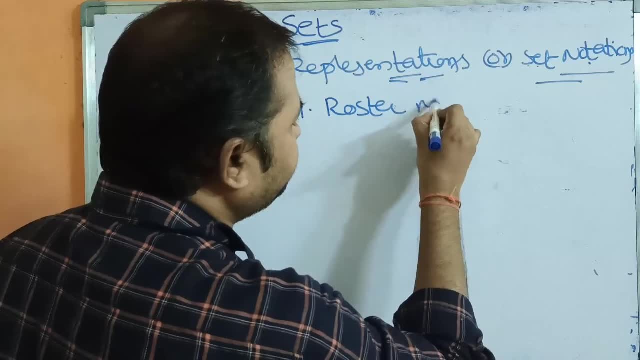 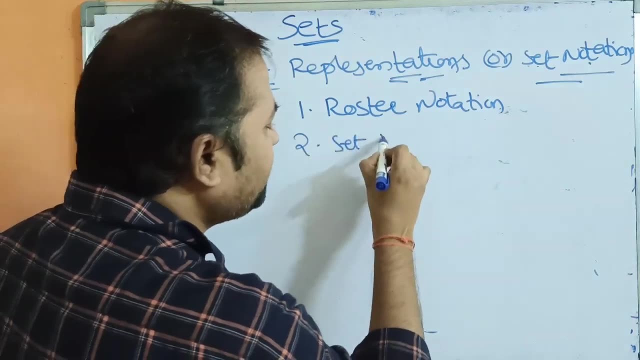 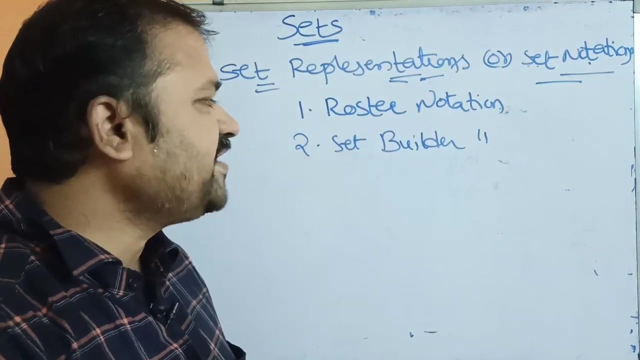 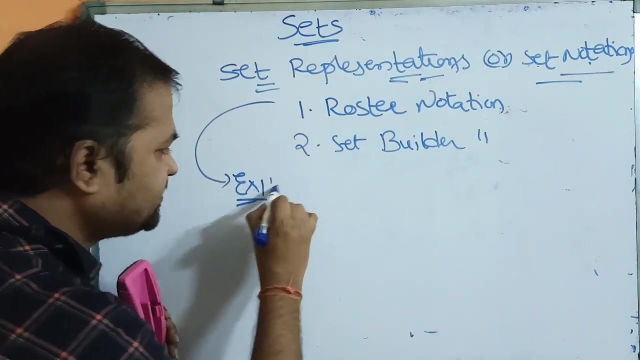 first notation is we can use roster notation, roster notation. and the second approach is we can use set builder notation. so we can represent sets in two ways. first way is roster notation, second way is set builder notation. first let us see about roseter notation. let us take an example. okay, set of set. 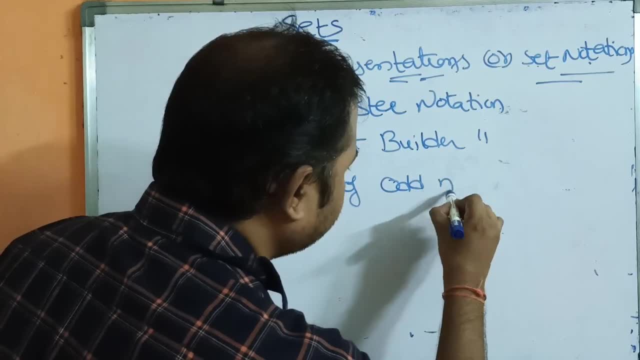 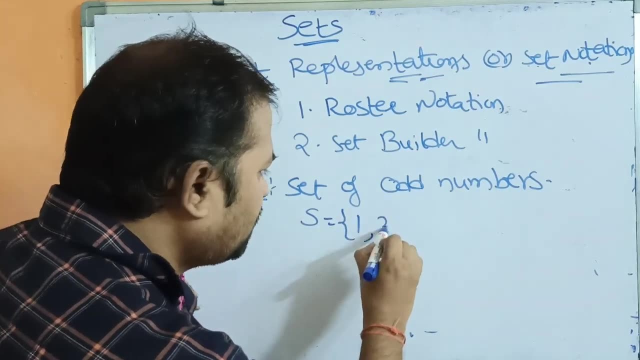 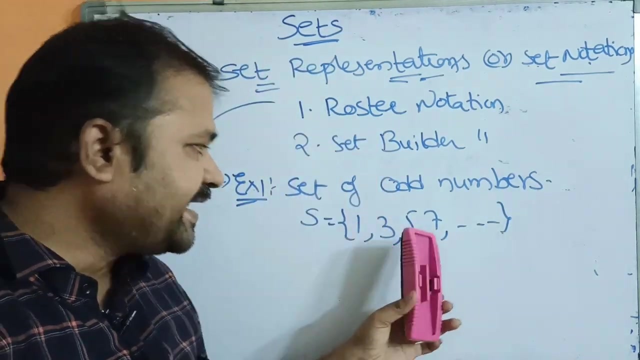 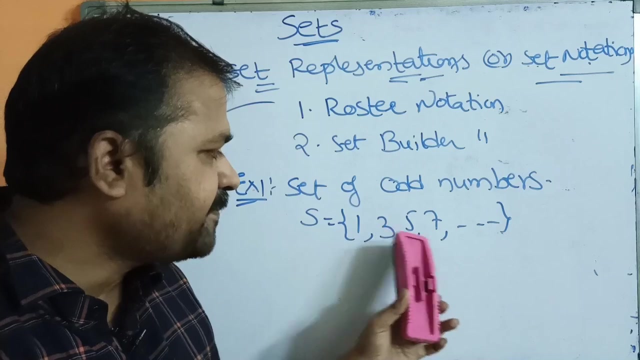 of odd numbers, set of odd numbers. okay, odd numbers. S is equal to, within the curly braces, 1 comma 3 comma 5 comma 7, so on. okay, Rosetta notation means here the elements are the members of the set must be enclosed in curly braces and they are separated by comma symbol. okay, this is called as roaster notation. 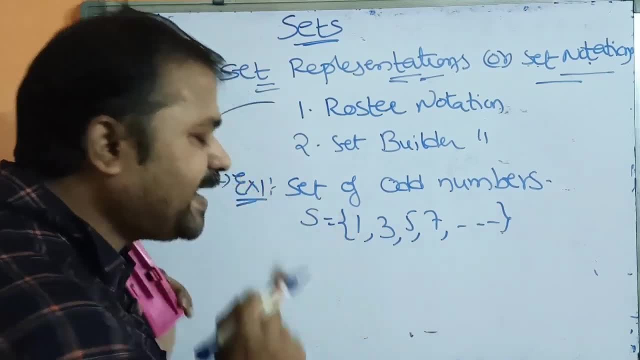 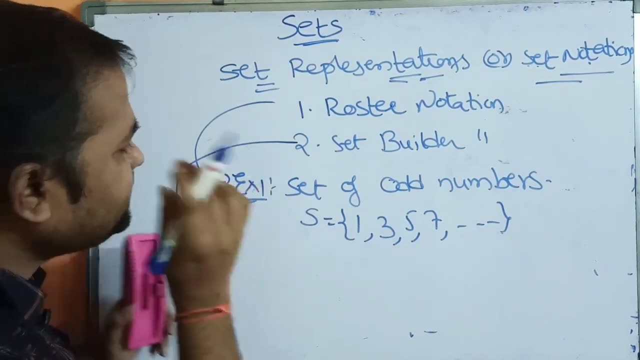 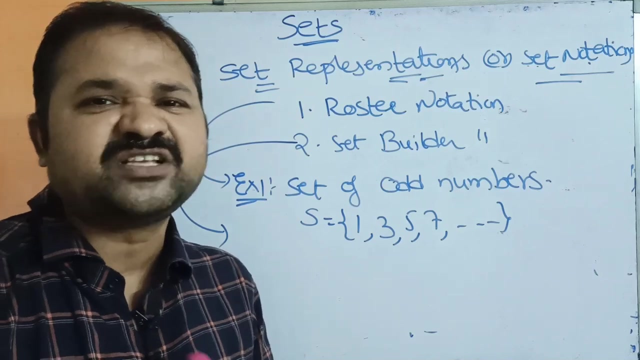 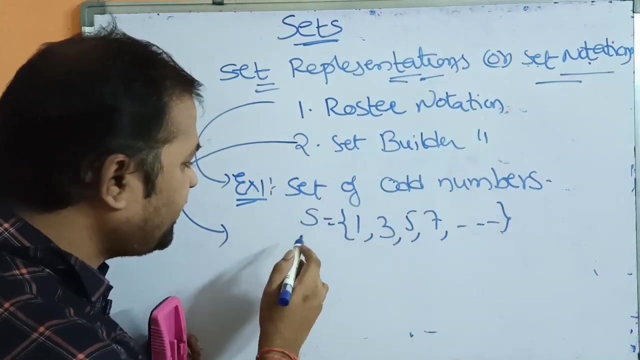 the elements must be enclosed in the curly braces and they are separated by comma symbol. now let us see the second approach. second approach: what is the second approach? set to builder notation. set to builder notation means here all the elements which possess the same property- okay- must be represented here. if you consider the same example, set of odd numbers. 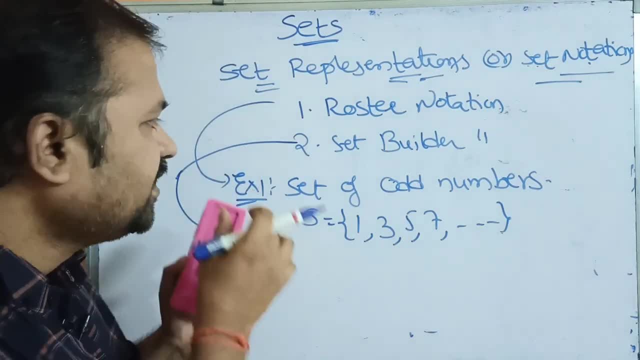 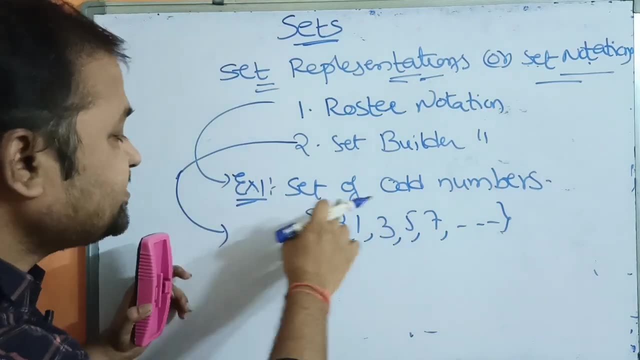 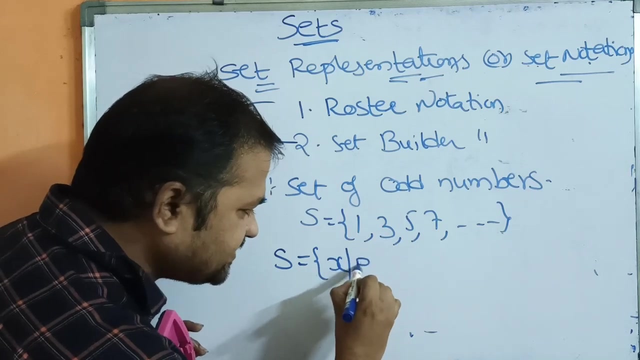 set to builder notation. set to builder notation means here all the elements which possess the same property. okay, must be represented here. if we consider the same example, set of odd numbers. so here we can represent as, like this: s is equal to x, such that p of x, p of x means what that property, here all the. 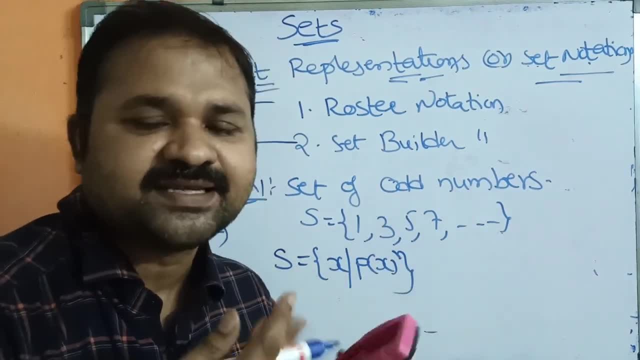 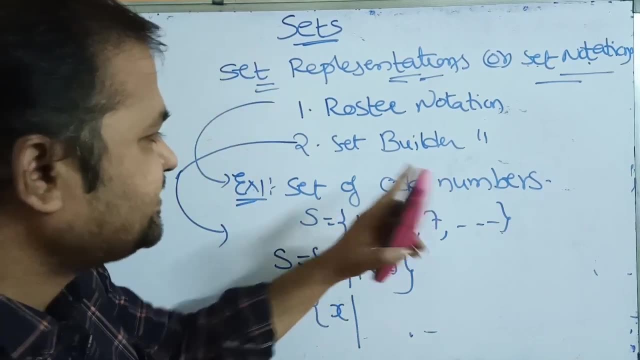 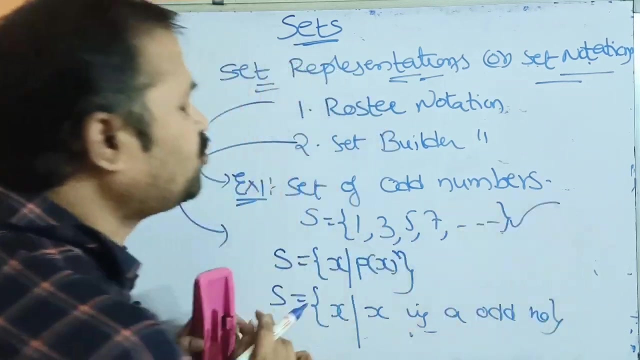 elements of the set must process, must possess the same property, must have the same property. so s is represented as: like this: x such that same example: x is a odd number, x is a odd number. okay, this representation is called as roaster notation, whereas this representation is called as what? 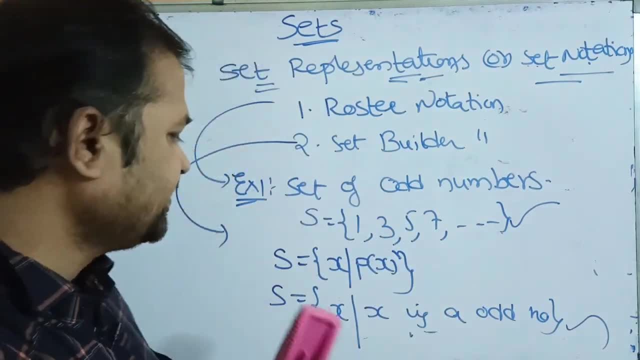 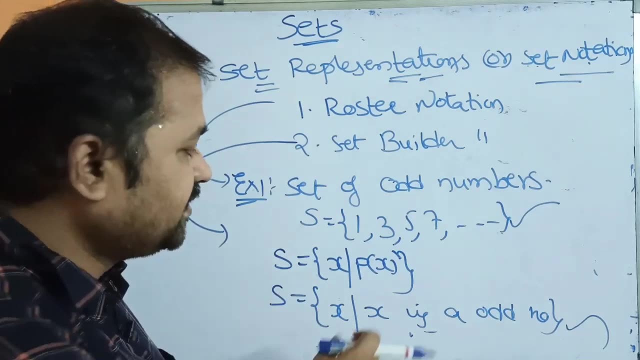 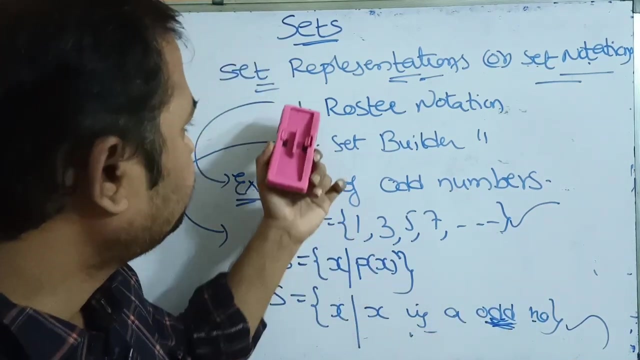 set builder notation. set builder notation: okay, set builder notation means we have to follow this index properties, so the elements which have the same property so must be placed here. so here, what is the elements property? common property is odd numbers. so we can represent the set in these two ways: first approach is roster notation and the second 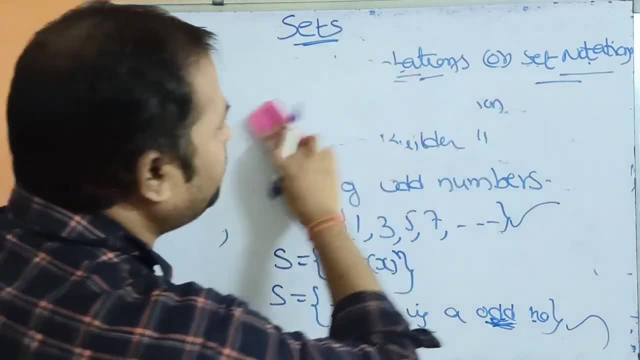 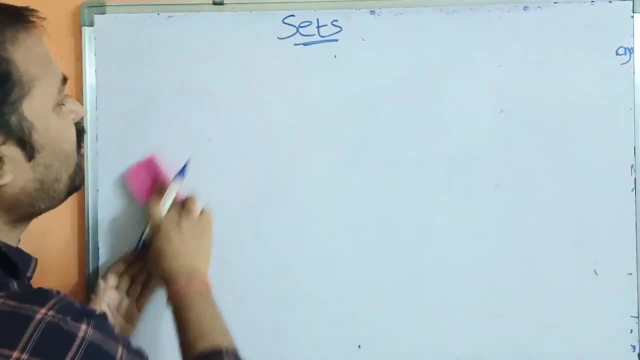 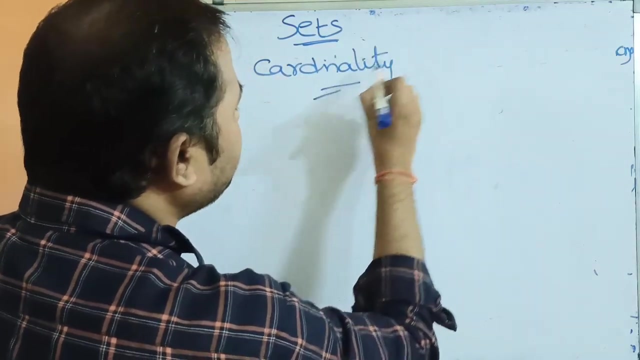 approach is what set to builder notation. now let us see about various terminologies on the set. the first terminology is cardinality of the set. what is cardinality? cardinality of the set, cardinality of a set. so cardinality means it specifies the number of elements which are present. 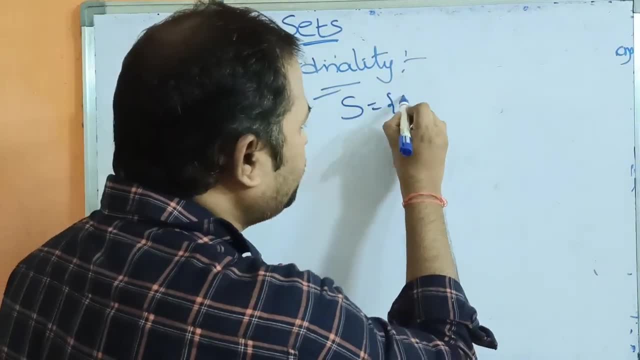 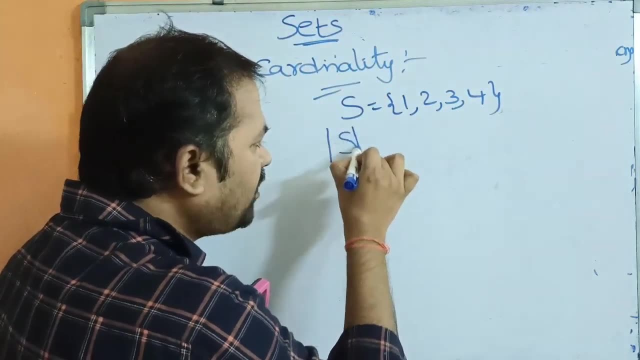 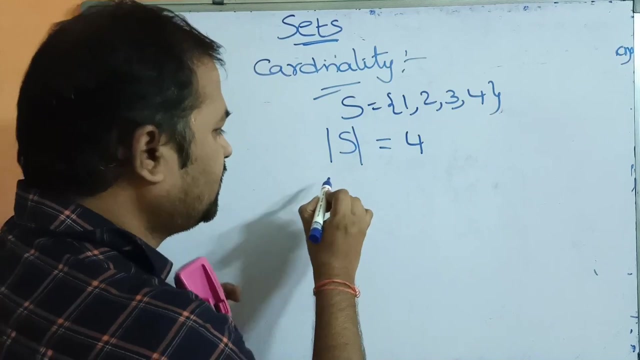 in the set. let we have a set like this: s is equal to 1 comma 2 comma, 3 comma 4. then cardinality of the set is represented with the help of mod s is equal to here. this set contains how many elements? 4 elements. so mod s is equal to 4. so let us take another example. we have one more set like this: s. 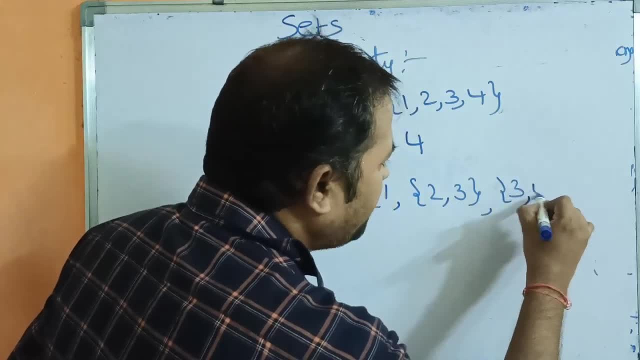 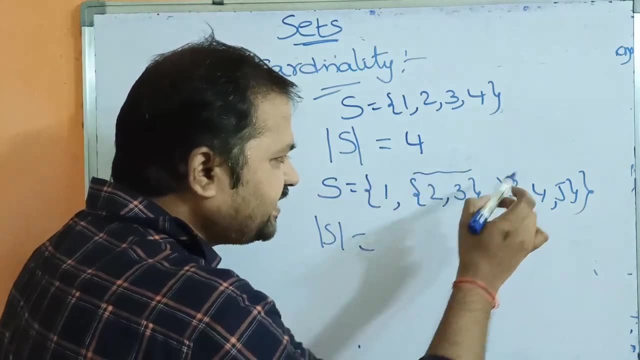 is equal to 1 comma, 2 comma 3, 3 comma, 4 comma 5 nested set. okay, now, what is mod s here? 1 means one element, whereas this 2 comma 3 is another element, whereas this 3 comma, 4 comma 5 is another. 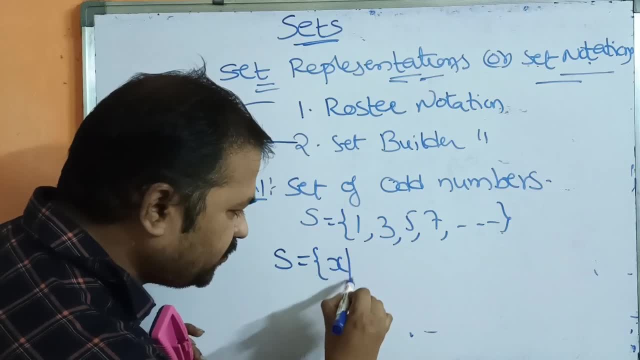 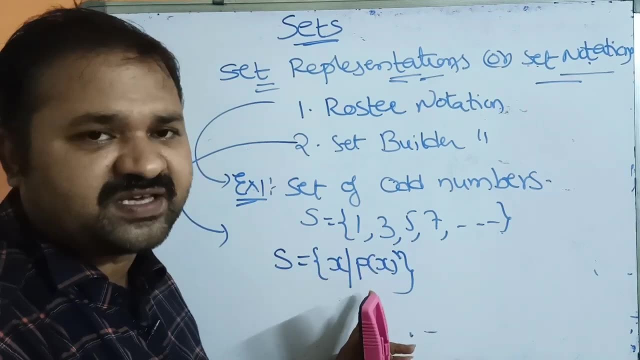 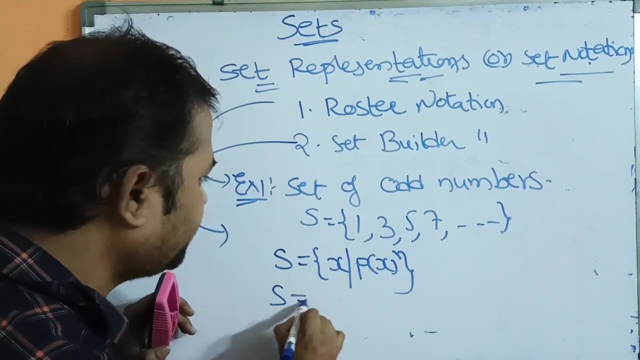 so here we can represent as like this: s is equal to x, such that p of x. p of x means what that property- here all the elements of the set must process- must possess the same property, must have the same property. so s is equal to. we can represent as like this: x such that same example: x is a odd. 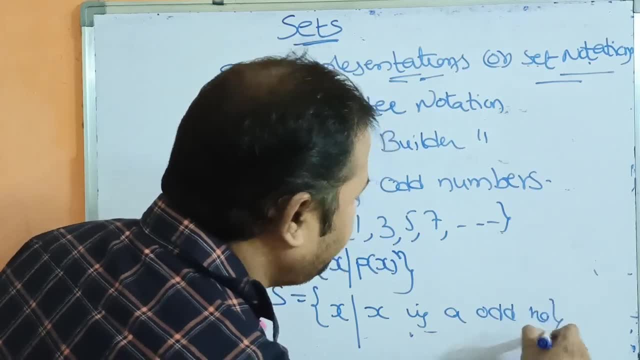 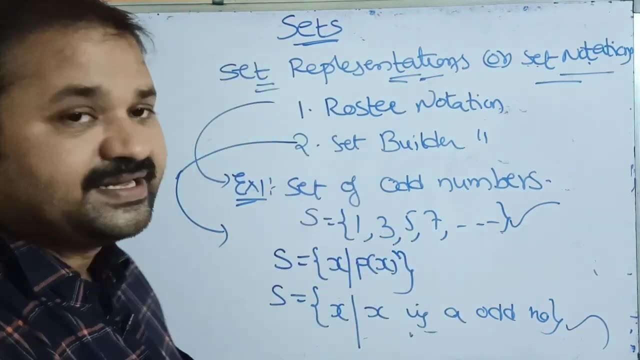 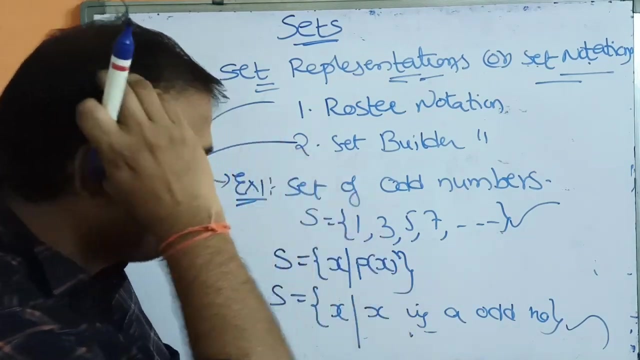 number x is a odd number. a odd number, okay. this representation is called as roster notation, whereas this representation is called as what set builder notation. set builder notation, okay. set builder notation means we have to follow this index properties, so the elements which have the same property so must be placed. 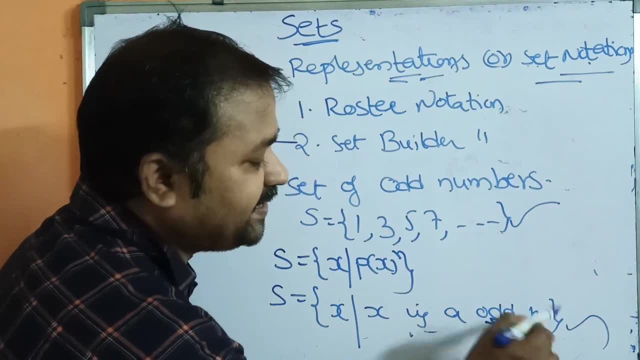 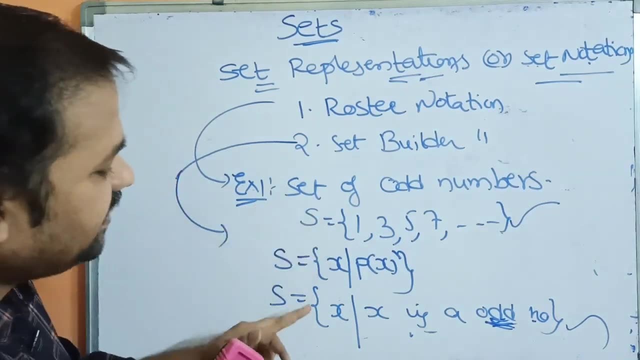 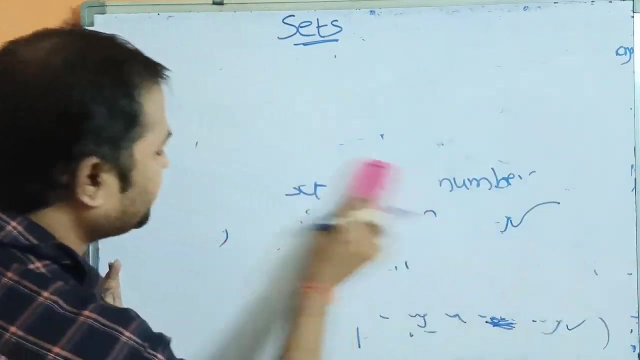 here. so here, what is the elements property? common property is odd numbers. so we can represent the set in these two ways. first approach is roster notation and the second approach is what set to builder notation. now let us see about various terminologies on the set. the first terminology is: 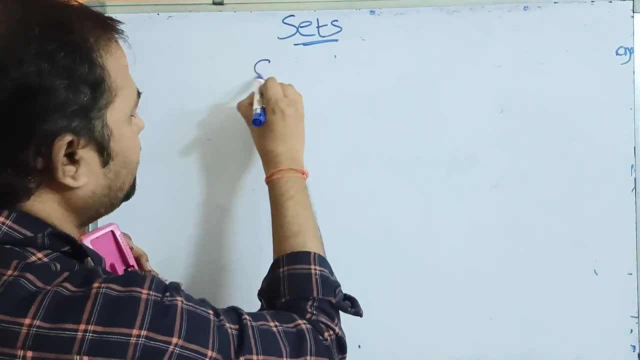 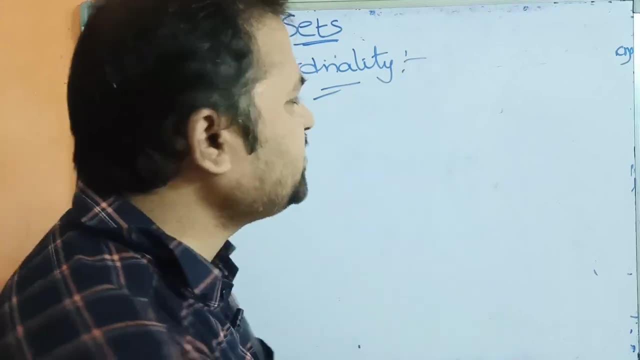 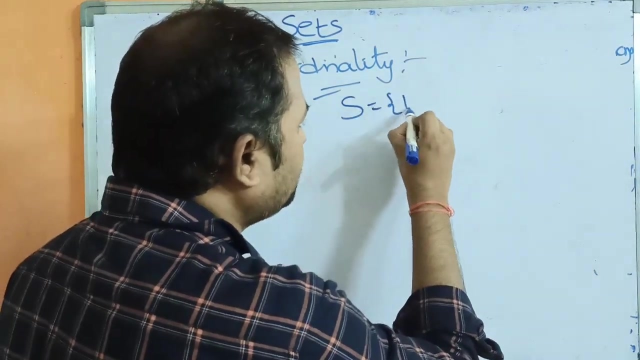 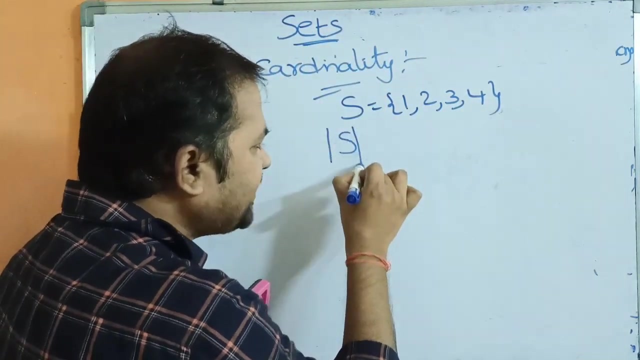 cardinality of the set. what is cardinality? cardinality of the set, cardinality of a set. so cardinality means it specifies the number of elements which are present in the set. let we have a set like this: s is equal to 1 comma, 2 comma, 3 comma, 4.. then cardinality of the set is represented with the help of mod s. 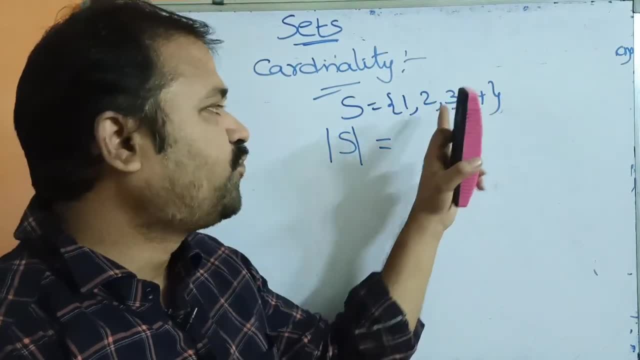 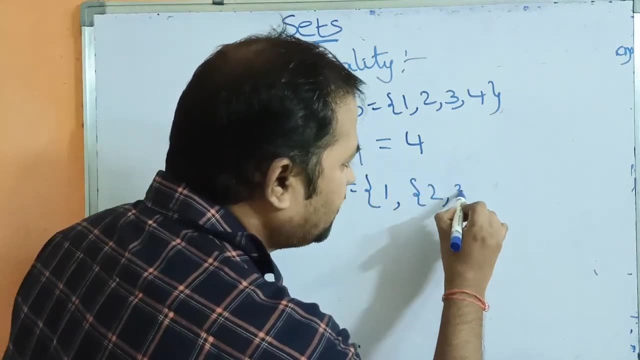 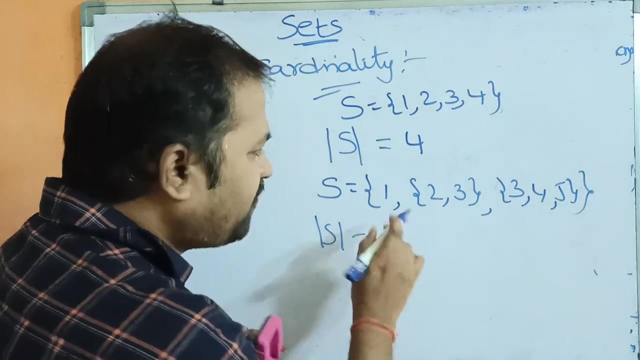 is equal to here. this set contains how many elements? four elements, so mod s is equal to four. so let us take another example. we have one more set like this: s is equal to 1 comma, 2 comma 3, 3 comma, 4 comma 5 nested set. okay, now what is mod s here? 1 means one element, whereas this 2. 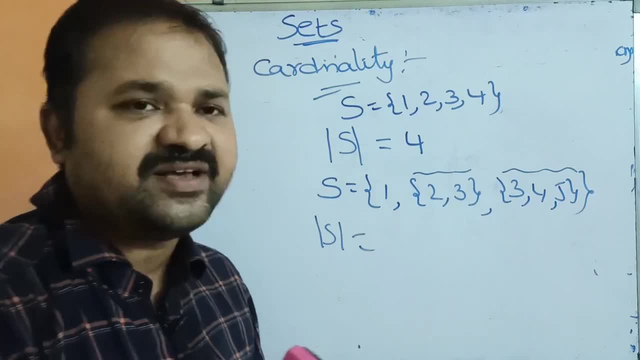 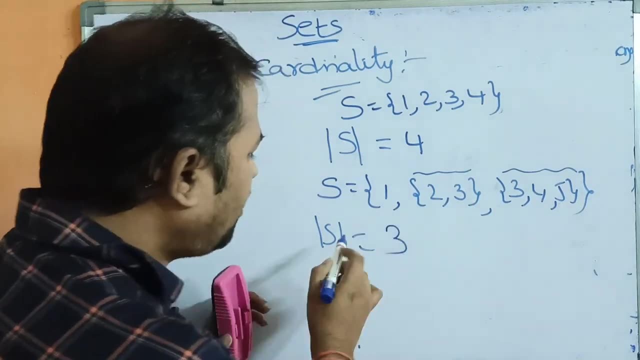 comma 3 is another element, whereas this 3 comma 4, comma 5 is another element. so mod s means 3 elements only. so it is not 3 plus 3, 6 elements. okay. so cardinality means it is represented by mod s. so cardinality is nothing but size of the set. 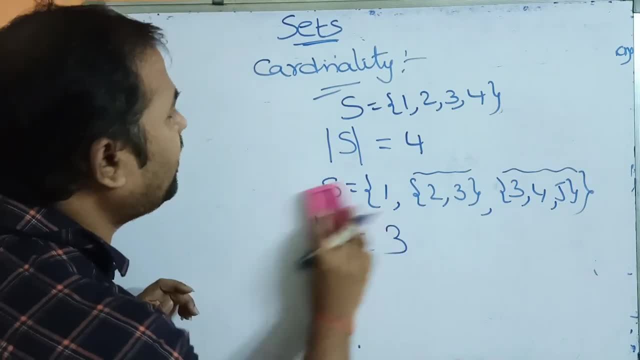 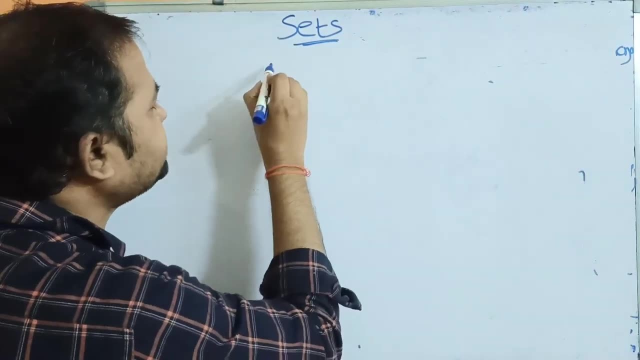 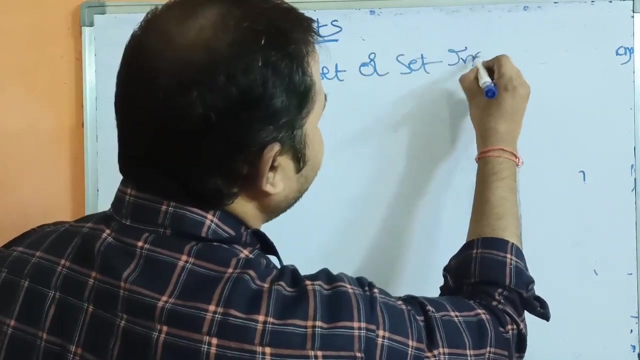 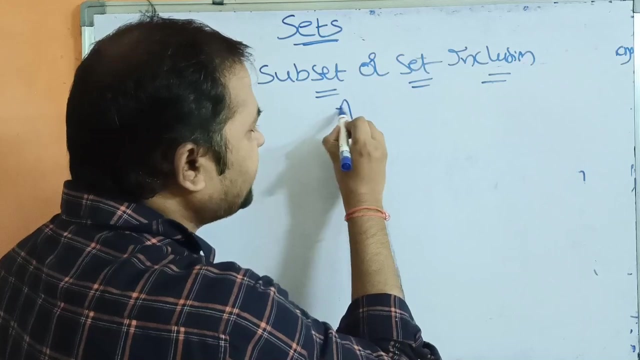 the number of elements which are present in the set. now let us see the next terminology, that is subset. what is a subset? subset can also be called as inclusion of a set, subset or set inclusion, subset or said set inclusion. let us see what is subset. let we have two sets, such as a and b. then we 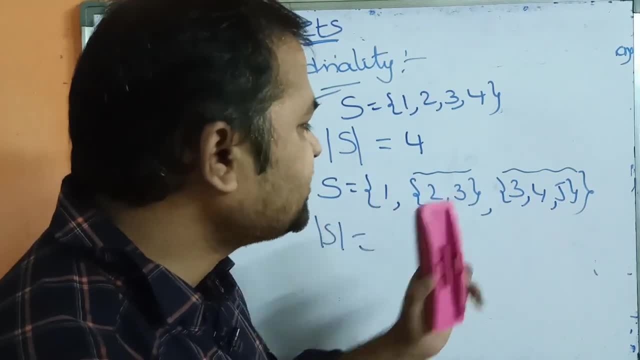 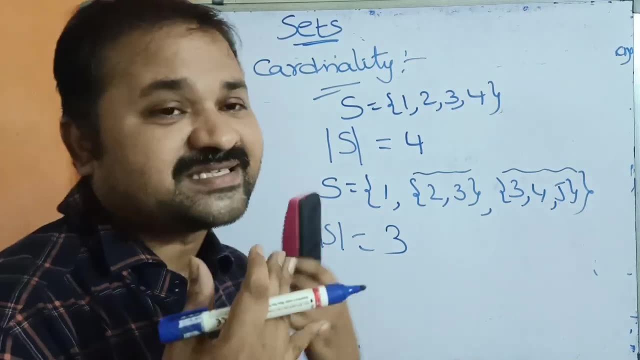 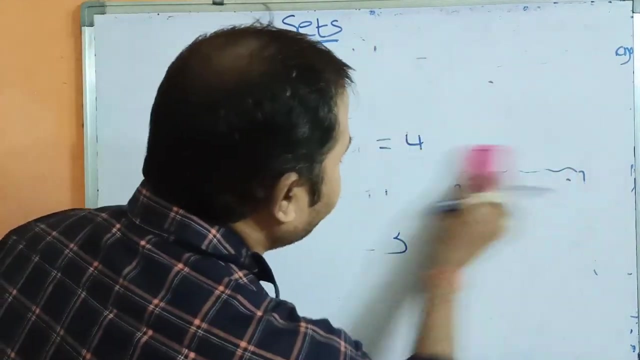 element. so mod s means 3 elements only. so it is not 3 plus 3, 6 elements. okay, so cardinality means it is represented by mod s. so cardinality is nothing but size of the set, the number of elements which are present in the set. now let us see the next two terminology. that is subset? what is a? 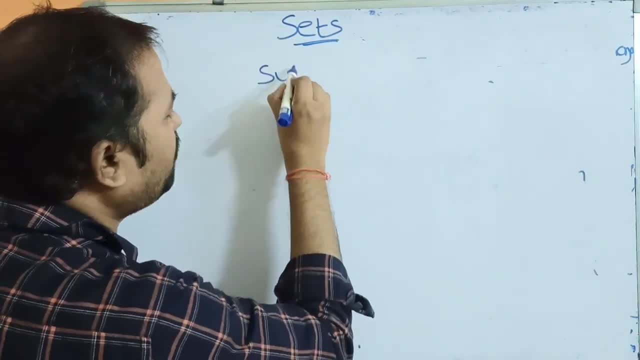 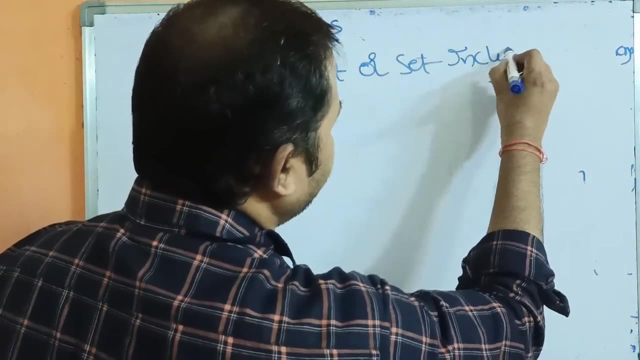 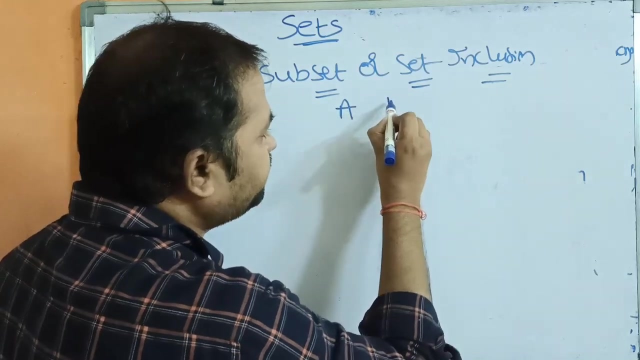 subset. subset can also be called as inclusion of a set, subset, subset or set inclusion, subset or said set, inclusion. let us see what is subset. let we have two sets such as a and b. then we can say that a subset, b subset is represented with the help of 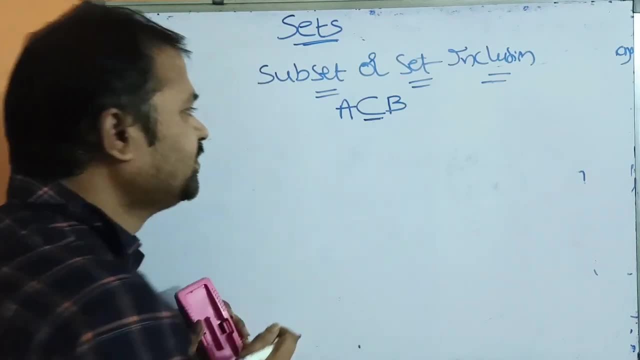 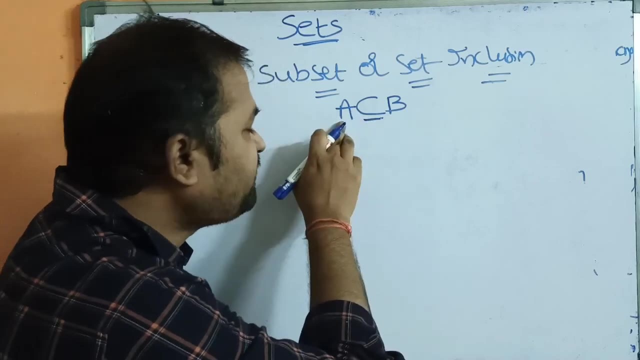 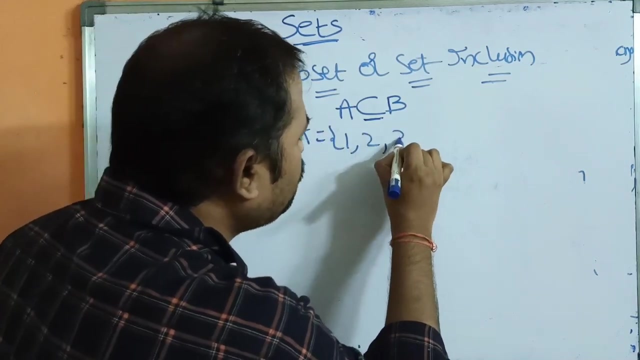 this symbol. okay, here we have to use this equal to also. okay, then we can say: let we have two sets such as a and b. then we can say that a subset b- if every element of a set is a subset of a set of a- is present in b. let us take some example: a is equal to 1 comma, 2 comma, 3. next b is equal to: 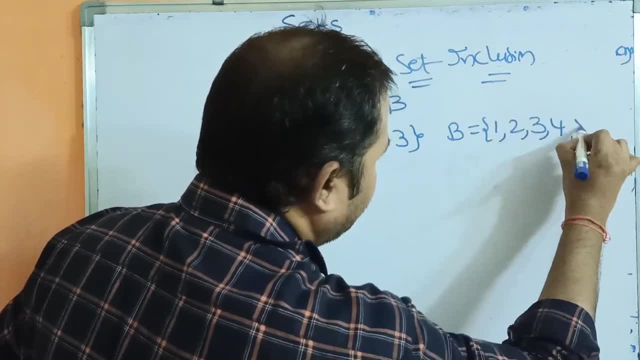 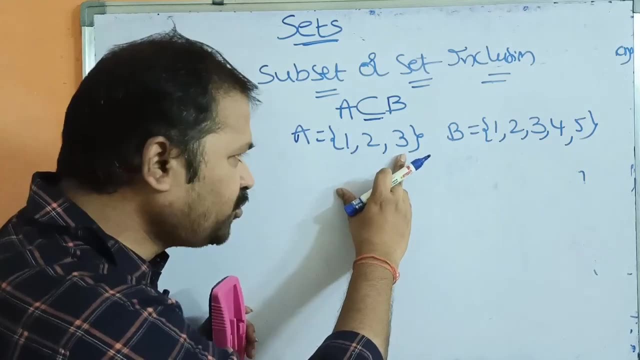 1 comma 2 comma 3 comma 5, if you consider this one, here we can write as a subset b. why? because what are the elements of a? 1, 2, 3? the elements of a are present in b. this 1, 2, 3 is present in b. 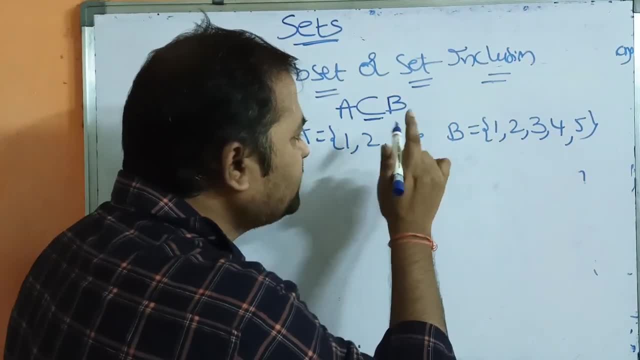 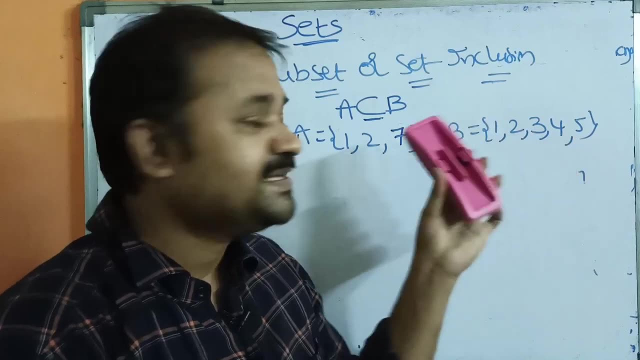 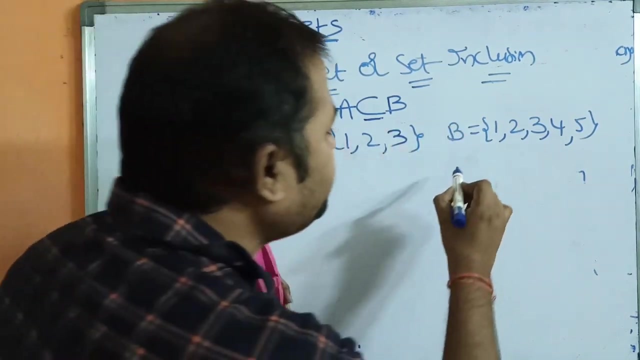 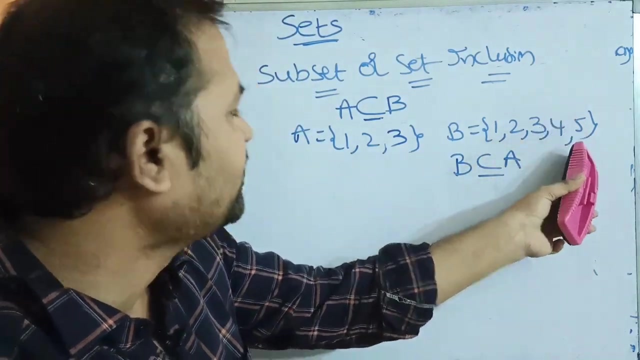 so we can say that a subset b. okay, but let us assume that we have 1, 2, 7. we can't say a subset b. why? because 7 is not present in b. 7 is not present in this set. okay, now can we say b subset a? can we say b subset a? we can't say b subset a. why? because 4 and 5. 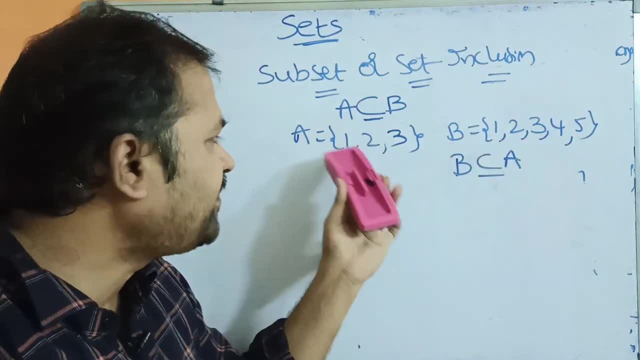 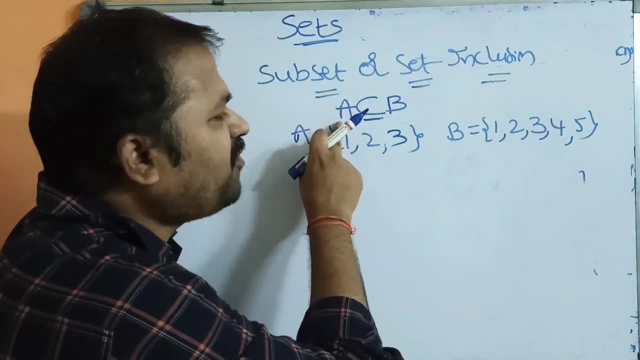 are not present in a. only the first three elements are present in a. the last two elements are not present in a. okay here, what is a subset b? if every element of a is present in b, then we can say that a is subset b. we should not bother about the remaining elements. 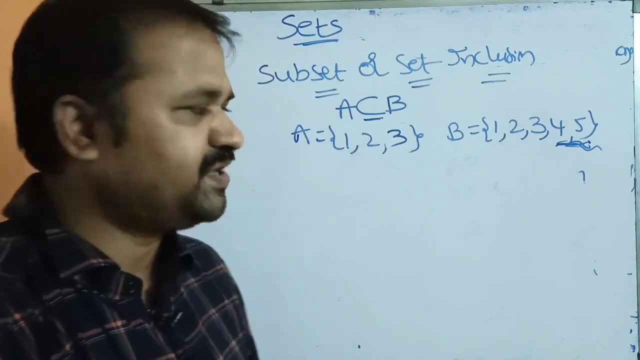 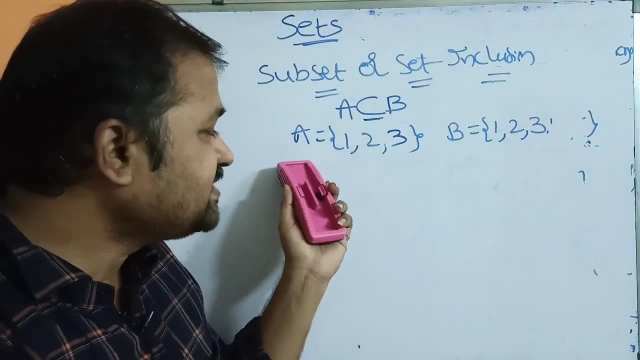 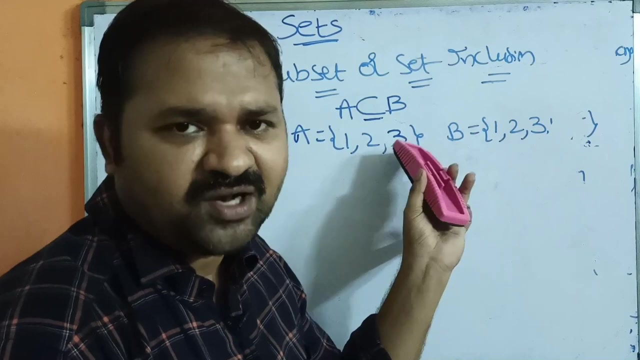 of the b. b contains two more elements. we should not bother about that. okay, let us assume that b also contains 1, 2, 3. b also contains 1, 2, 3. then we can say a subset b. yes, why? because every element of a, that is 1, 2, 3, is present in b. so now also we can say that a subset b. okay, so this is. 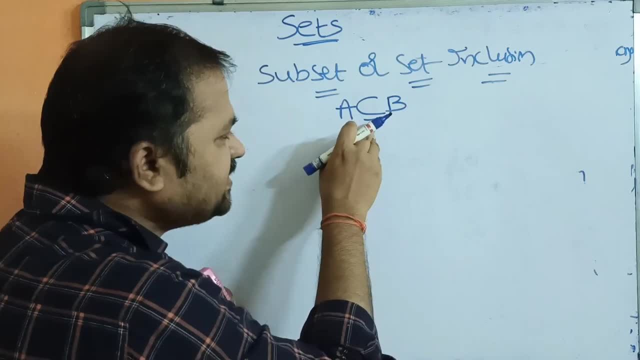 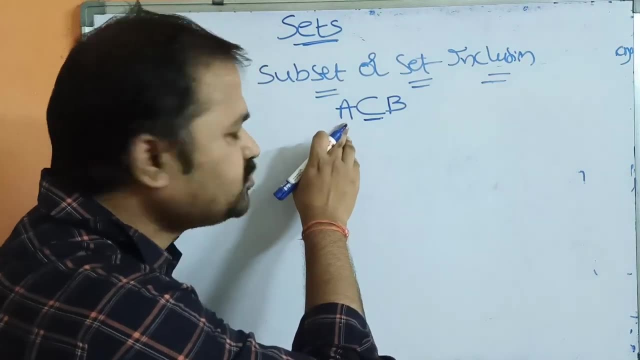 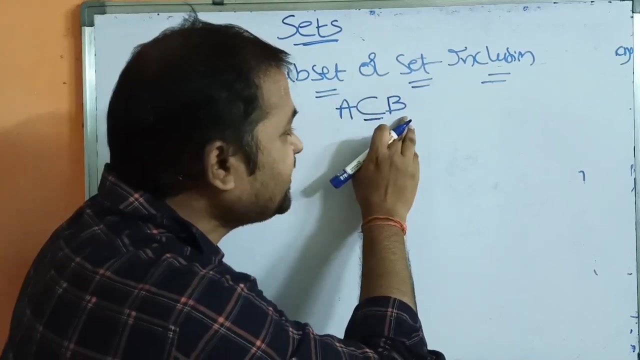 can say that a subset b subset is represented with the help of the symbol. okay, here we have to use this equal to also. okay, then we can say: let we have two sets such as a and b. then we can say that a subset b if every element of a is present in b. let us take some example: a is equal. 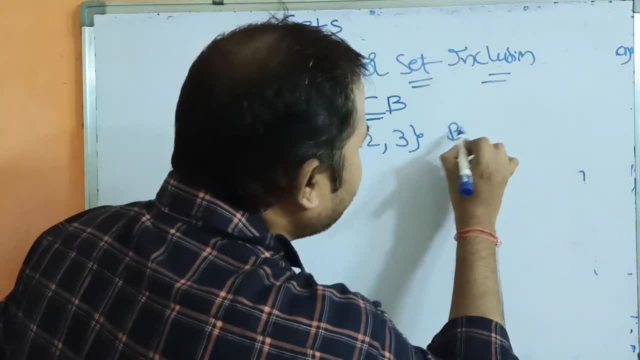 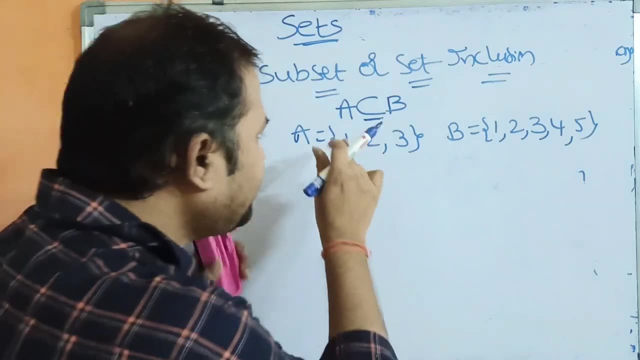 to 1 comma 2 comma 3 next to b is equal to 1 comma 2 comma 3 comma 5. if we consider this one here we can write as a subset b. why? because what are the elements of a? 1, 2, 3, the elements of a. 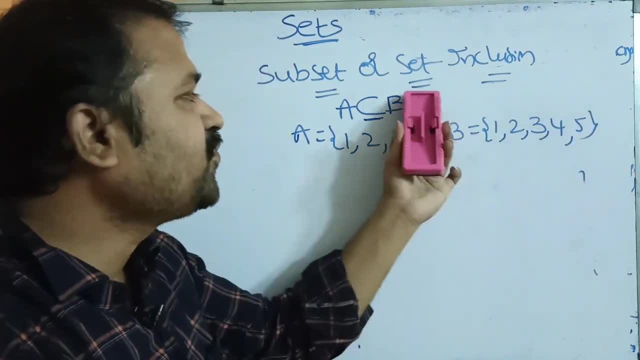 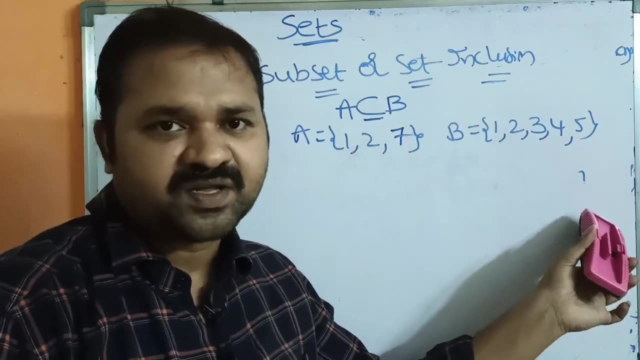 are present in b. this 1, 2, 3 is present in b, so we can say that a subset b. okay, but let us assume that we have 1 2, 7. then we can't say a subset b. why? because 7 is. not present in b. this is present in 1, b and 2, which are present in a subset b of the or a subset of a subset of a subset of b. if we explain this, we canrit that we can see we she also call subset of the element a to subjects. 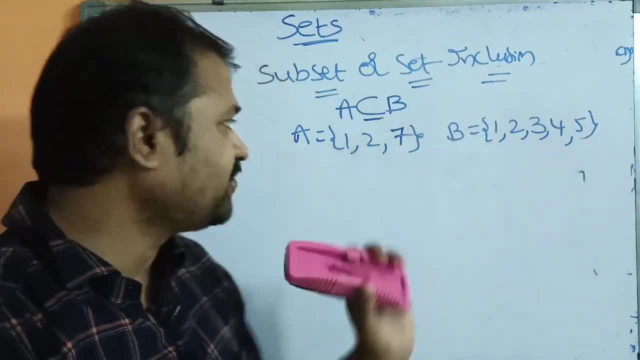 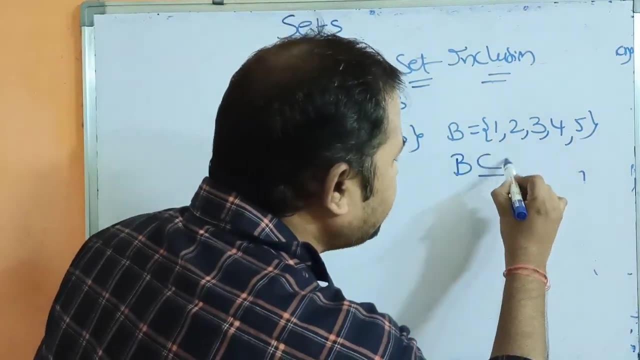 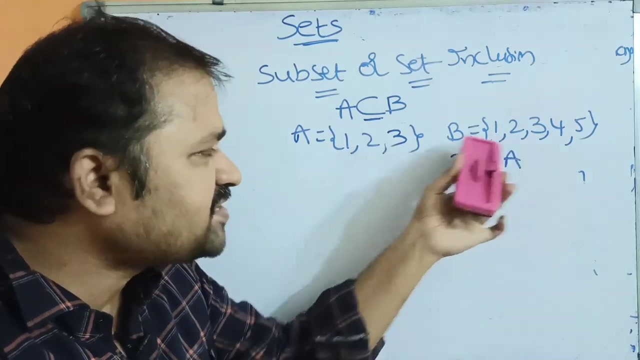 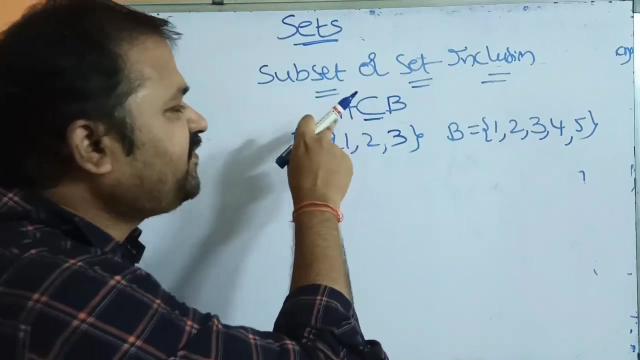 present in b. 7 is not present in this set. okay now, can we say b subset a? can we say b subset a? we can't say b subset a why? because 4 and 5 are not present in a. only the first three elements are present in a. the last two elements are not present in a. okay here, what is a subset b if 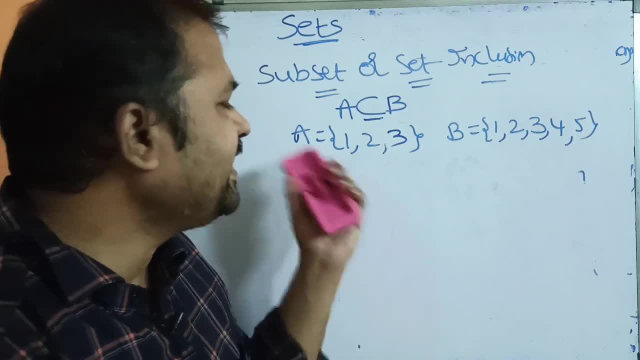 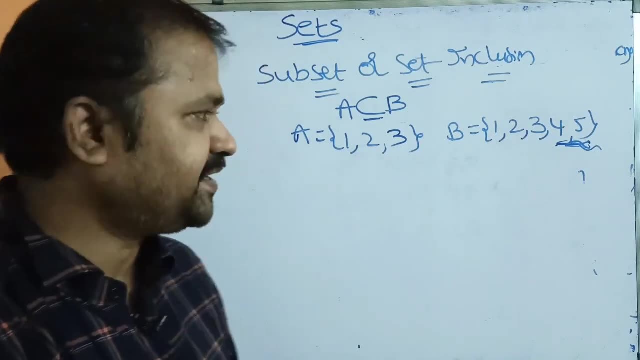 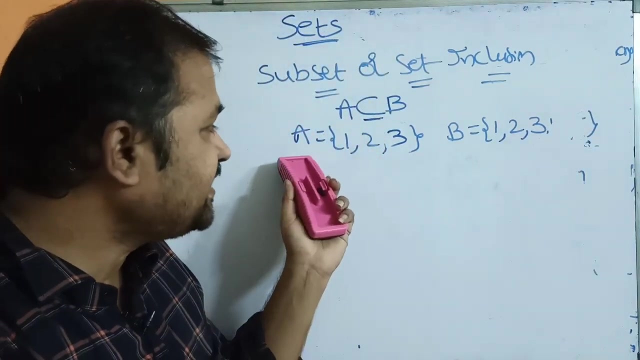 every element of a is present in b, then we can say that a is subset b. we should not bother about the remaining elements of the b. b contains two more elements. we should not bother about that. okay, let us assume that b also contains 1, 2, 3. b also contains 1, 2, 3, then we can say a subset b. 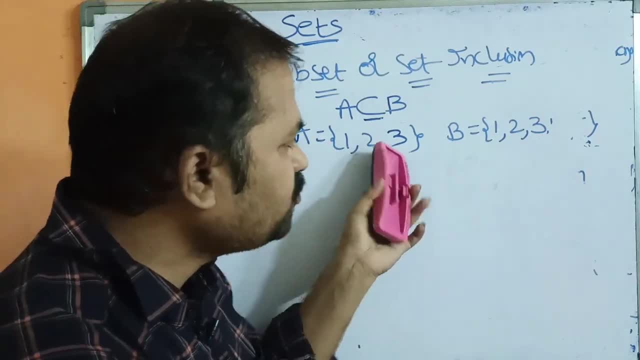 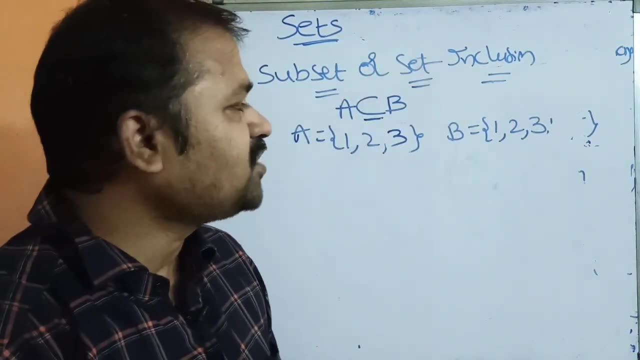 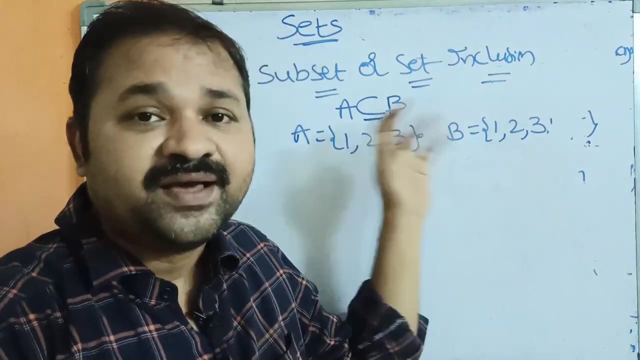 yes, why? because every element of a, that is, 1, 2, 3- is present in b. so now also we can say that a subset b. okay, so this is about subset, or this can also be called a subset b as set inclusion. why? because every element of a is included in b. every element of a is available. 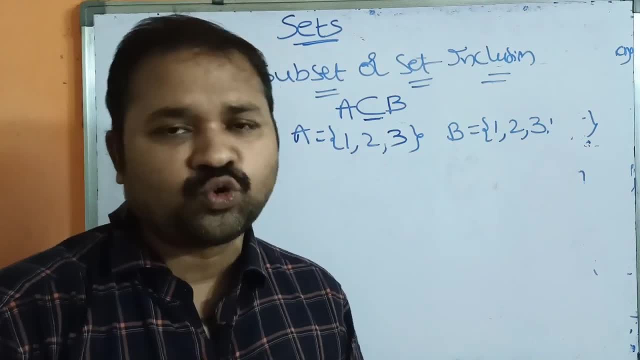 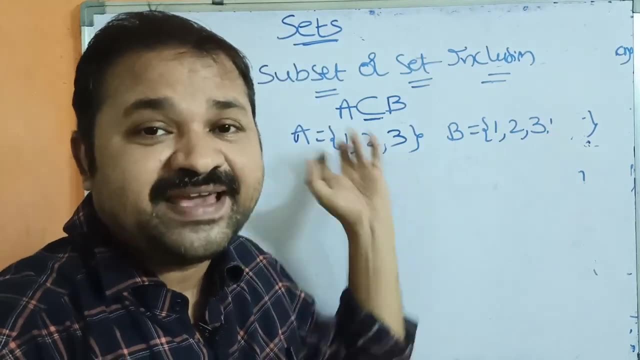 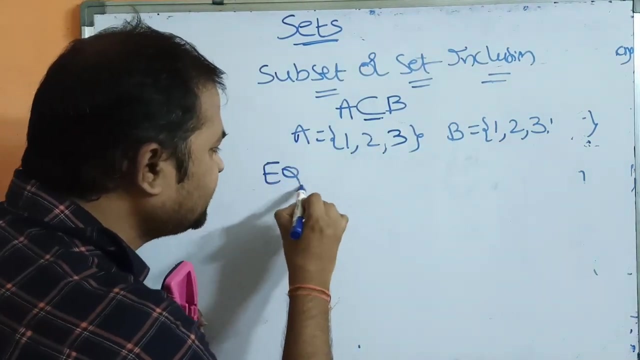 about subset, or this can also be called as set inclusion. why? because every element of a is included in b. every element of a is available in b, so that's why this can also be called as set inclusion. now let us see the next to terminology. so that is equality. 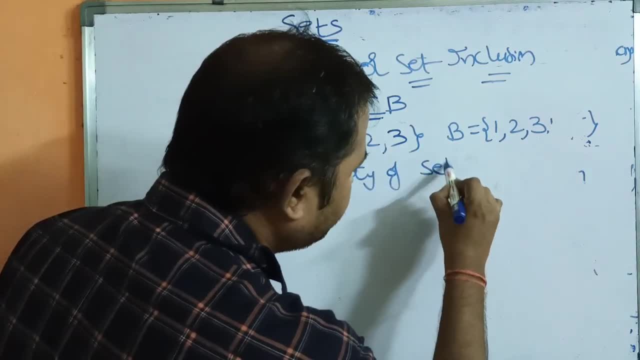 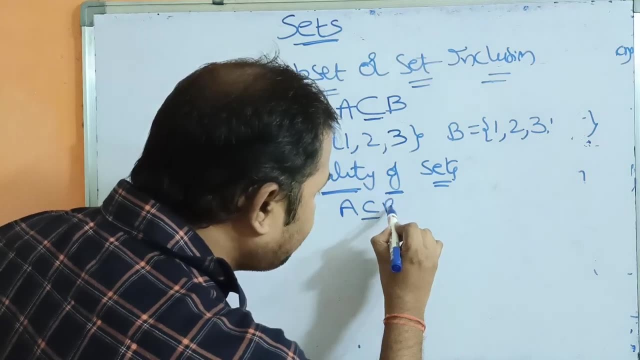 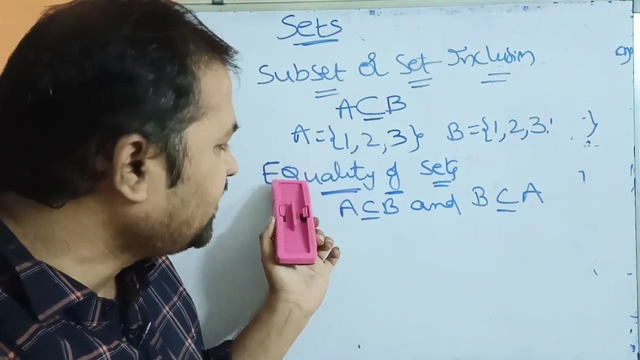 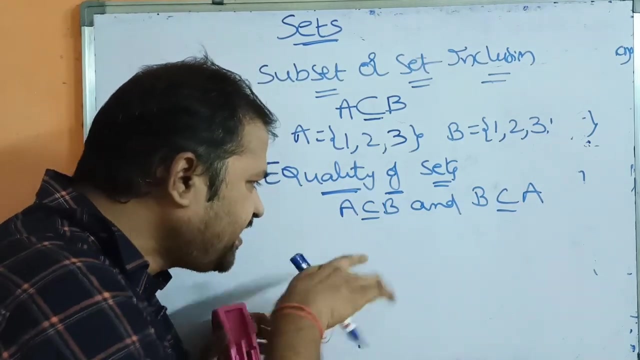 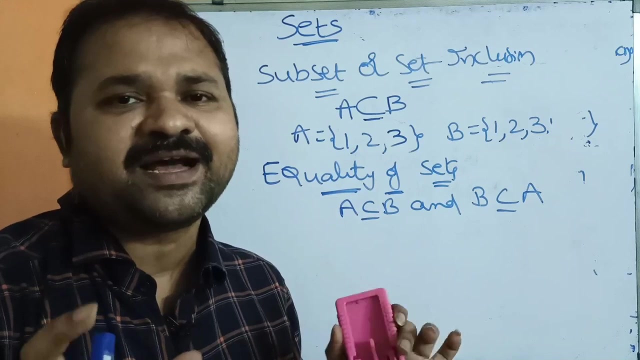 of sets. equality of assets. we can say that two sets are equal if, if a subset b and b subset a. we can say that two sets are equal if, and only if, a subset b and b subset a. that means every element of a must present in b as well as every element of b must present in a. that means a and b contain. 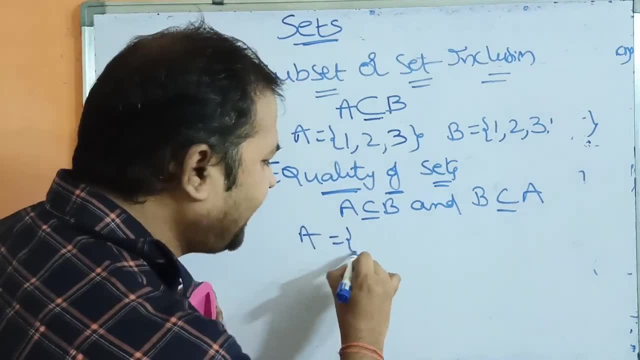 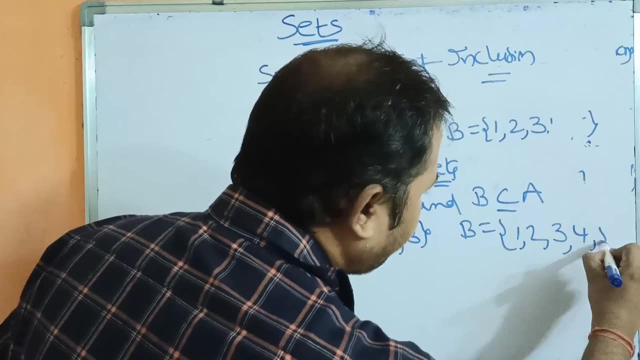 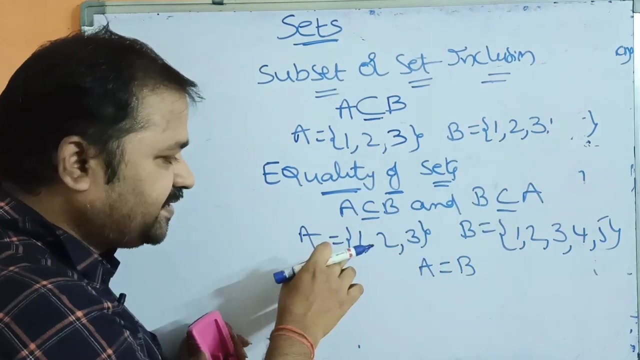 same number of elements. let us take an example for this. a is equal to 1, 2, 3, b is equal to 1, 2, 3, 4, 5. now can we say a subset b, a equal to b. so when we can say that a equal to b, when a subset b and b subset a, if you consider a subset b, a elements. 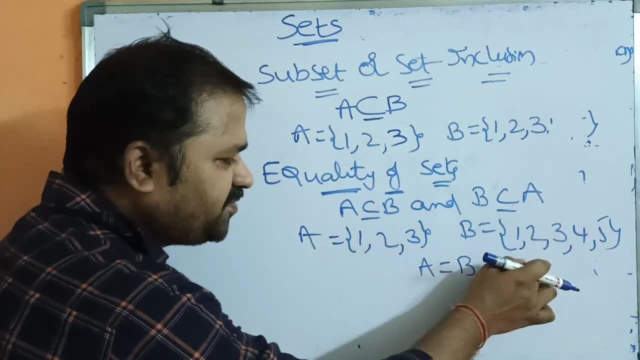 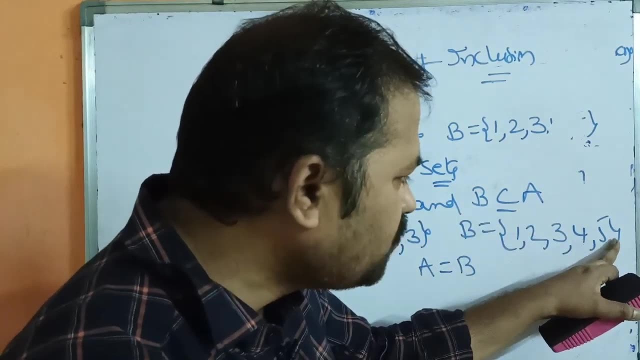 are 1, 2, 3. b elements are 1, 2, 3, 4, 5. here a subset b. why? because every element of a is present in b, but we can't say b subset a. why? because b contains two more elements: 4, 5. here every element of b is. 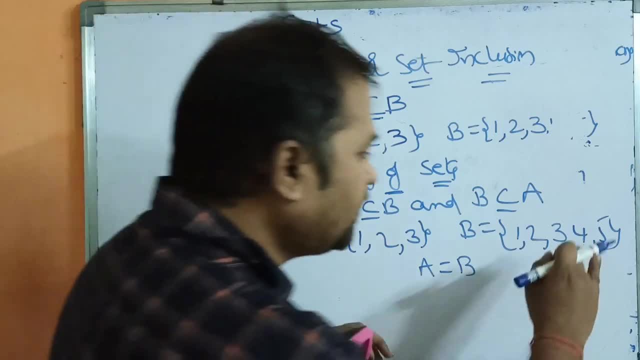 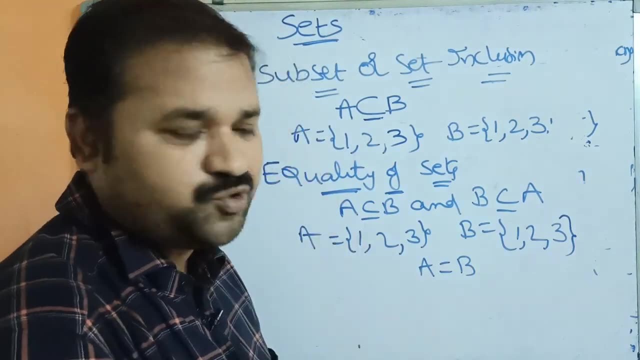 not present in a, so we can say that a is not equal to b. let us eliminate 4, 5. let us assume that b also contains 1, 2, 3. now we can say that a equals to b. why? because every element of a is present in b. 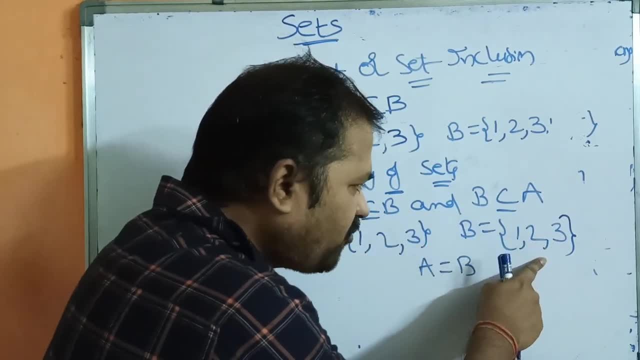 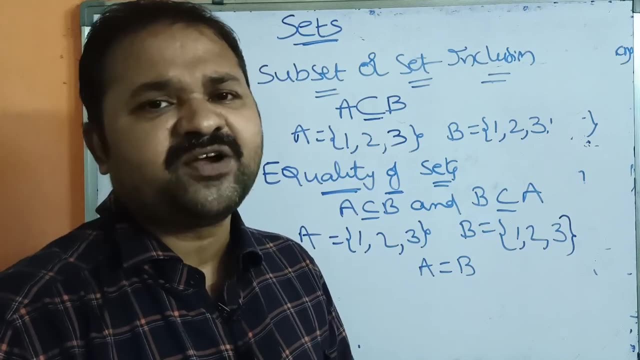 that means a subset b as well as every element of b, that is, 1, 2, 3. every element of b is present in a, so we can say that a is equal to b. so we can say that a is equal to b when both the sets contains. 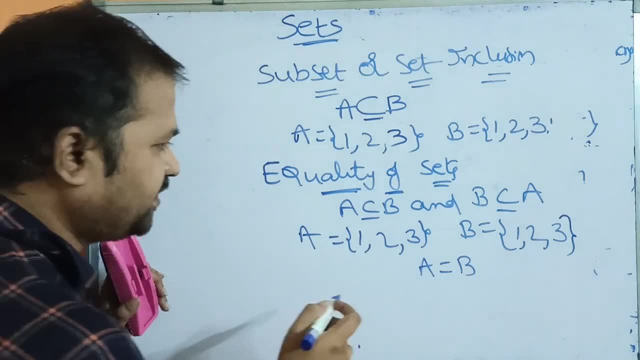 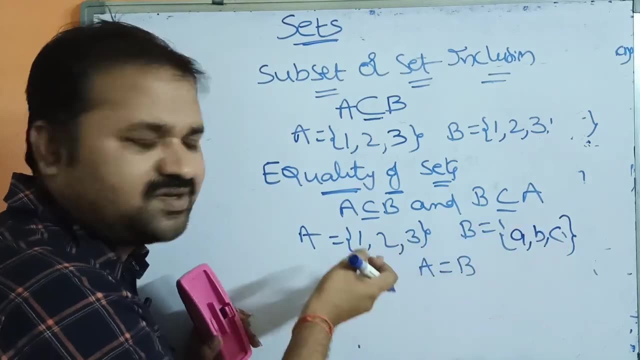 same number of elements, okay, same elements, okay. if we have abc here, then we can't say a is equal to b. why? because a elements are 1, 2, 3, b elements are a, b, c. so 1, 2, 3. they are not in b as well as. 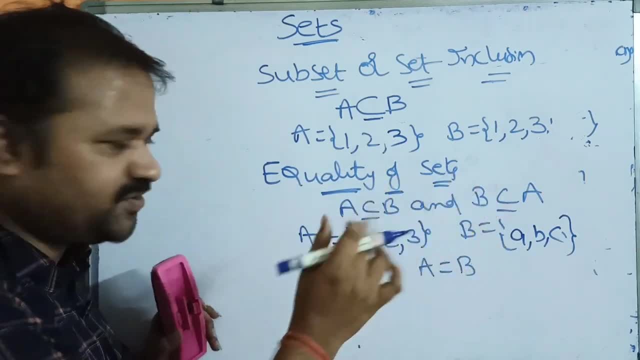 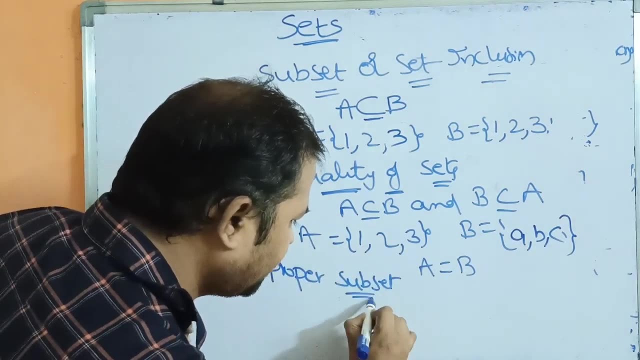 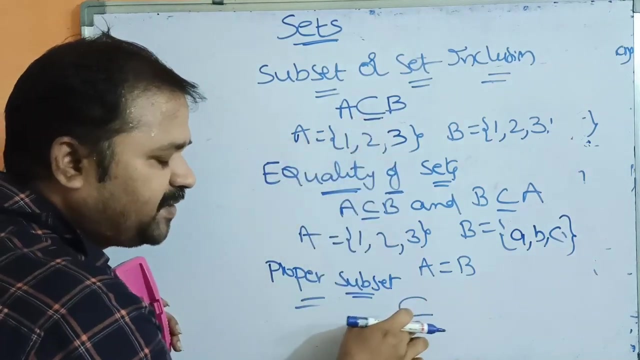 b elements a, b, c. they are not in a. okay, same elements, okay. and the next concept, next to terminology, is proper subset, proper subset, okay, proper subset is represented by this symbol. here there is no need of this equal operator. here we have equal operator, but here we don't. 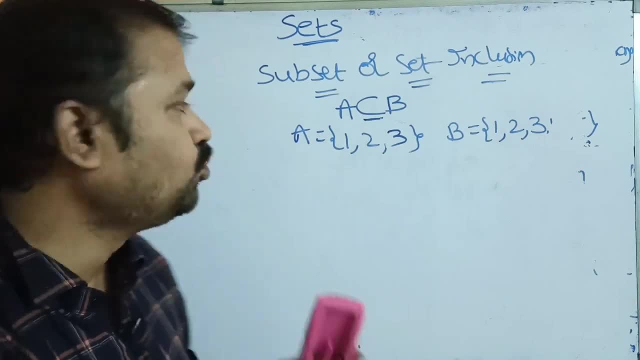 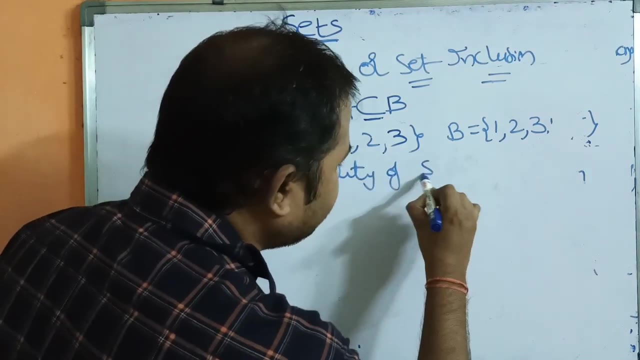 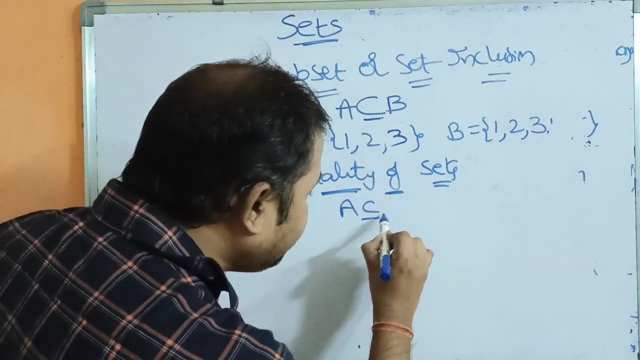 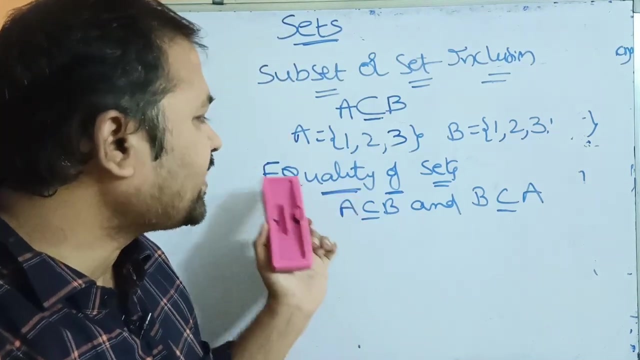 in b, so that's why this can also be called as set inclusion. now let us see the next two. so that is equality of sets. equality of sets. we can say that two sets are equal if, if a subset b and b subset a. we can say that two sets are equal if, and only if, a subset b and b subset a. that means every. 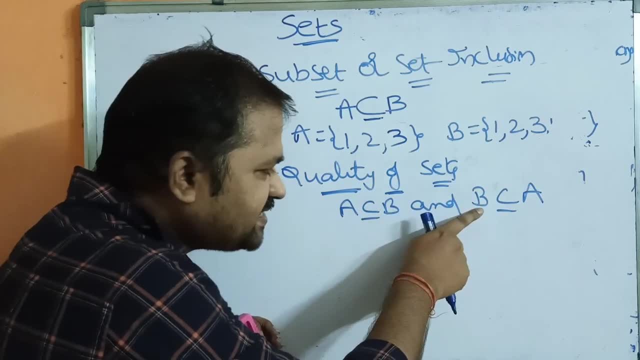 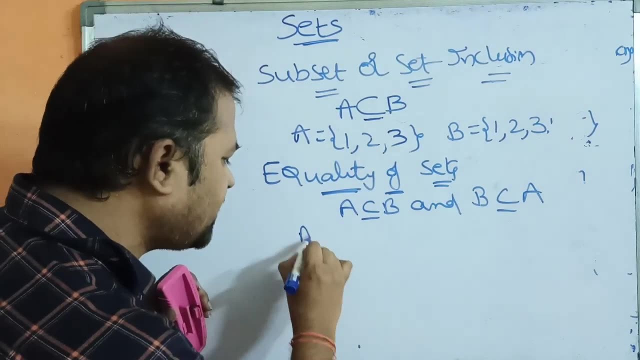 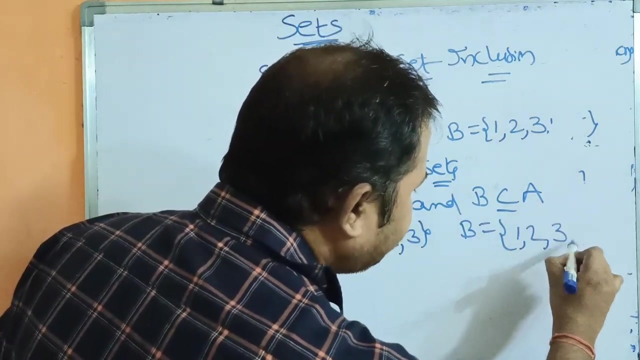 element of a must present in b, as well as every element of b must present in a. that means a and b contain same number of elements. let us take an example for this. a is equal to 1, 2, 3. b is equal to 1, 2, 3, 4, 5. now can we say a subset b: a equal to b. a is equal to 1, 2, 3. b is equal to 1, 2, 3, 4, 5. 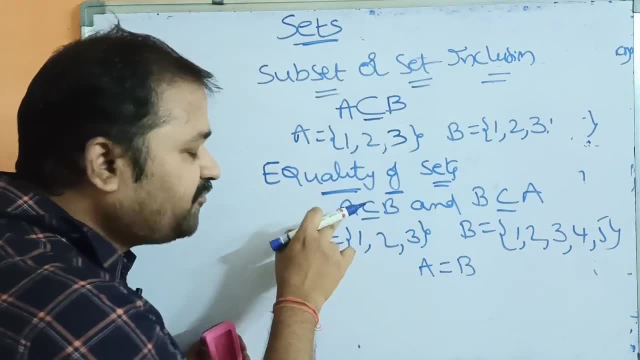 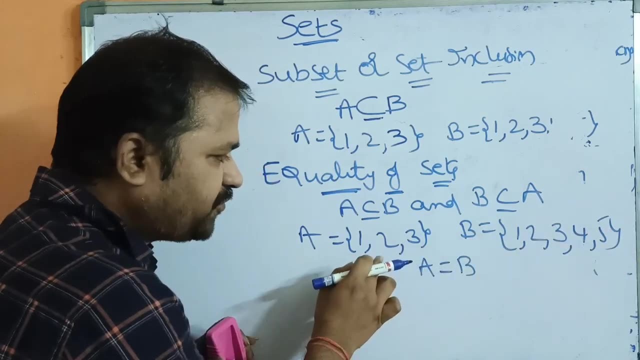 so when we can say that a equal to b, when a subset b and b subset a, if you consider a subset b, a elements are 1, 2, 3, b elements are 1, 2, 3, 4, 5. here a subset b. why? because every element of a is present in b. 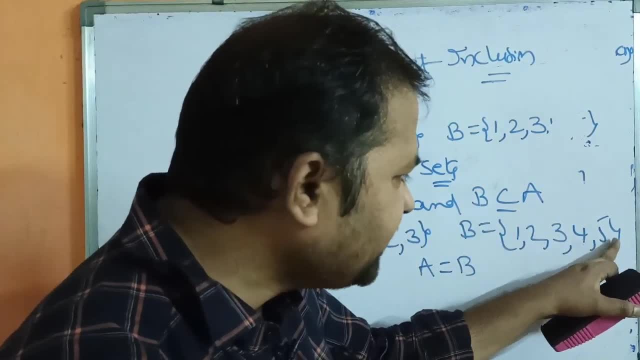 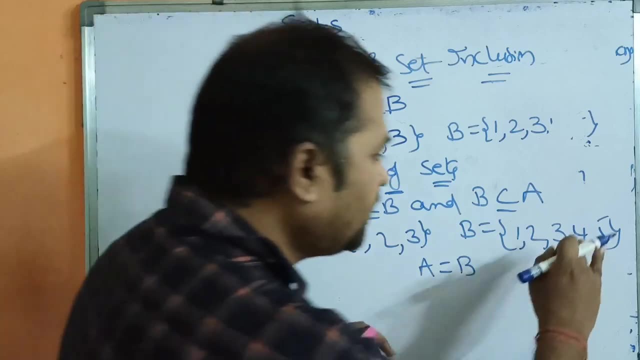 but we can't say b subset a. why? because b contains two more elements: 4, 5. here every element of b is not present in a. so we can say that a is not equal to b. let us eliminate 4, 5. let us assume that b also 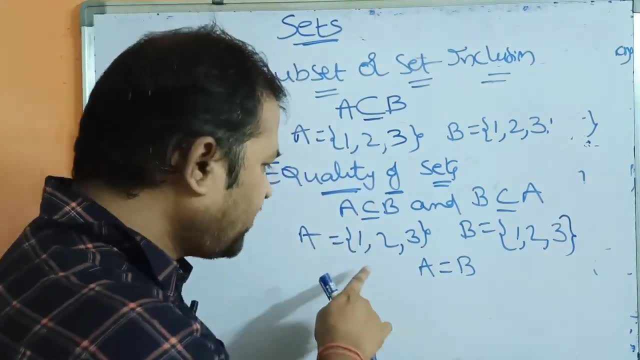 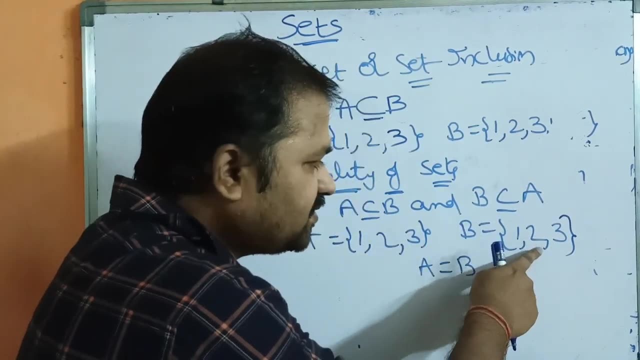 contains 1, 2, 3. now we can say that a equals to b. why? because every element of a is present in b. that means a subset b as well as every element of b, that is, 1, 2, 3. every element of b is present in a. 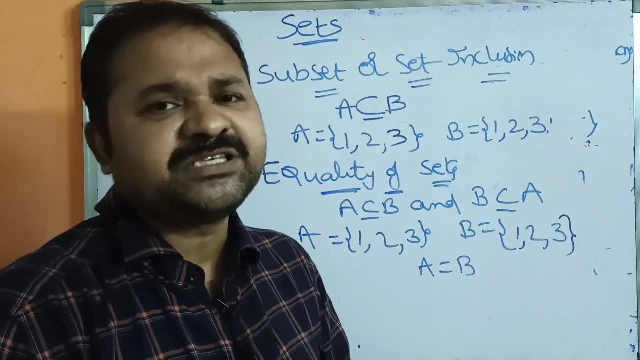 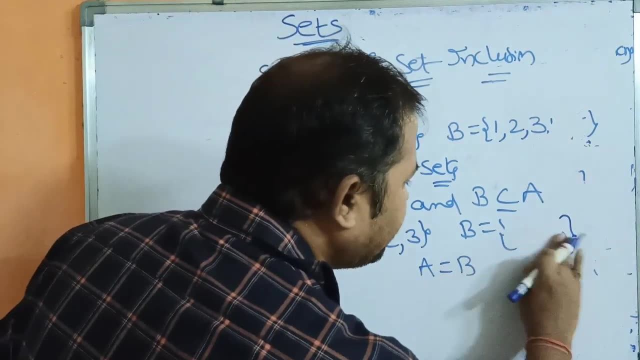 so we can say that a is equal to b. so we can say that a is equal to b when both the sets contains same number of elements. okay, same elements, okay. if we have abc here, then we can't say a is equal to b. why? because a elements are 1, 2, 3, b elements are abc, so 1, 2, 3. 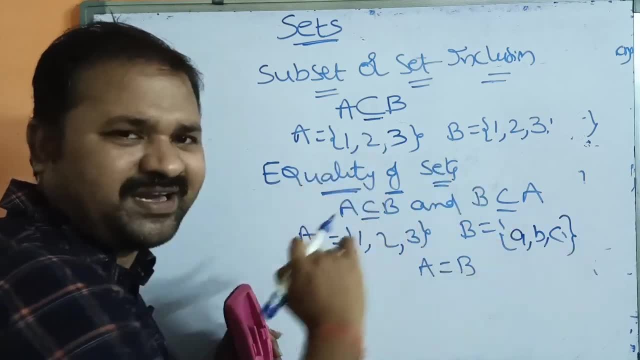 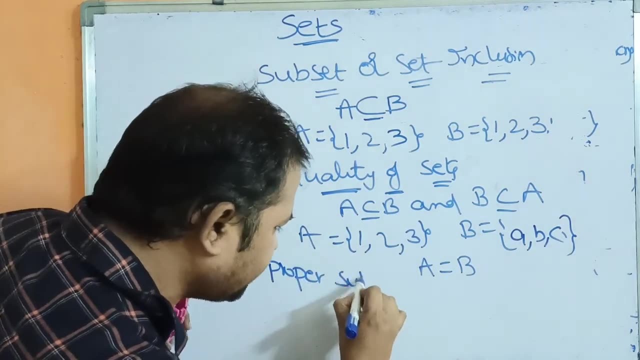 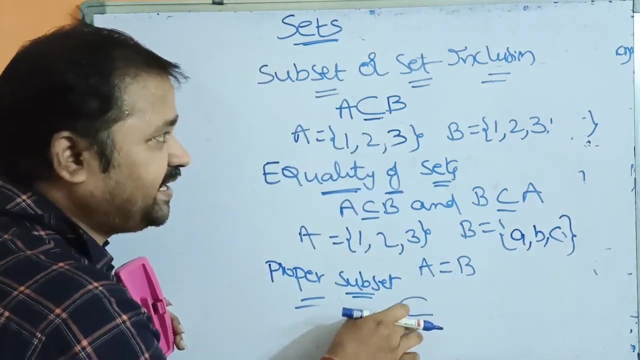 they are not in b as well as b elements, abc. they are not in a: okay, same elements, okay. and the next concept, next to terminology, is proper subset, proper subset, okay. proper subset is represented by this symbol. here there is no need of this equal operator. here we have equal operator. but 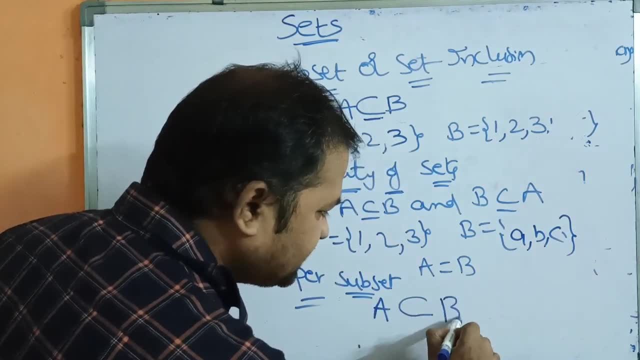 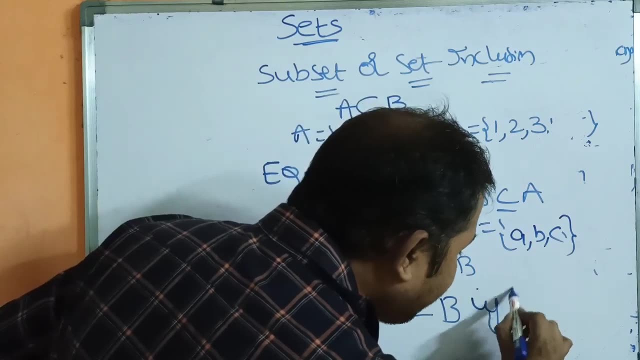 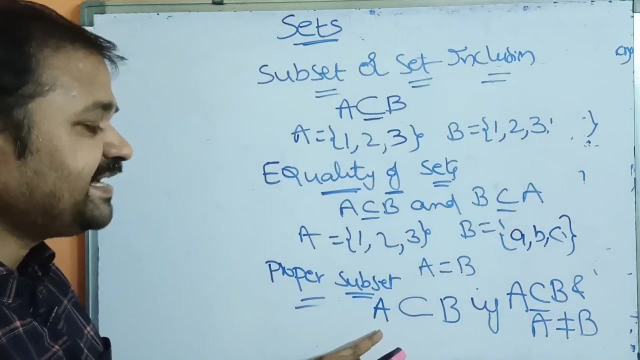 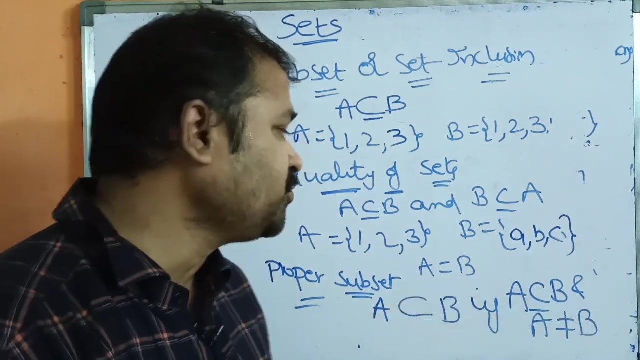 here we don't have equal operator, so this is nothing but proper subset b. we can say that a is a proper subset b if, if, if a subset b as well as a not equal to b. so if we consider this, this example: a is equal to 1, 2, 3. 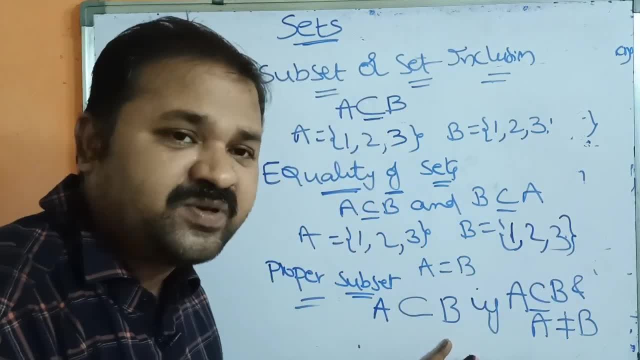 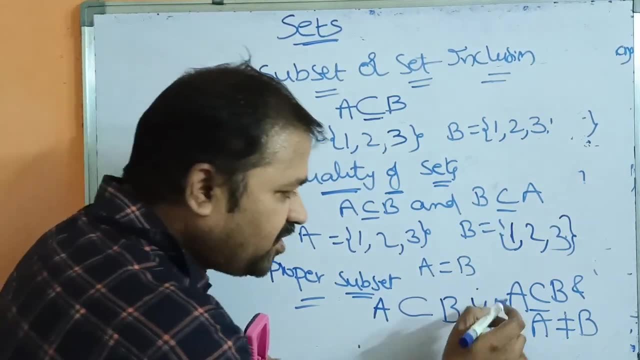 b is equal to 1, 2, 3. now can we say a subset b? we can't say like that. why? because, i'm sorry, can we say a proper subset b? no, why? because here, what is the first condition? a subset b. so that means every element of a must present. 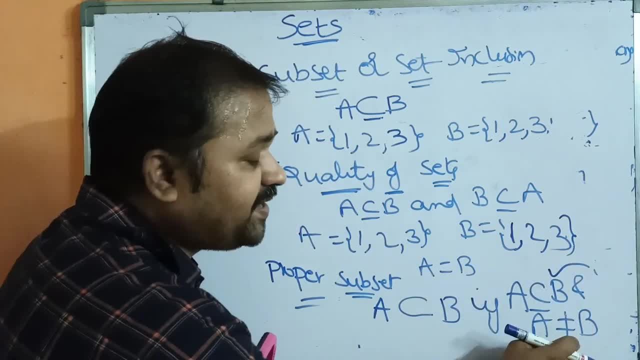 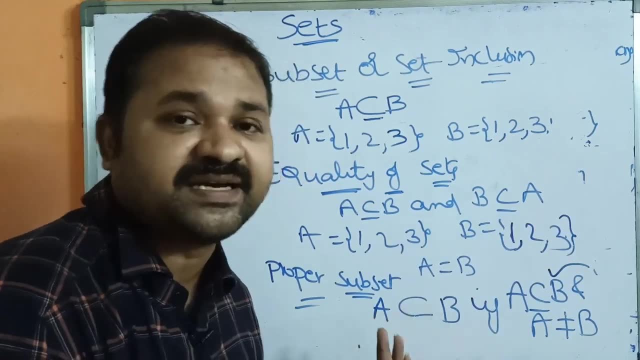 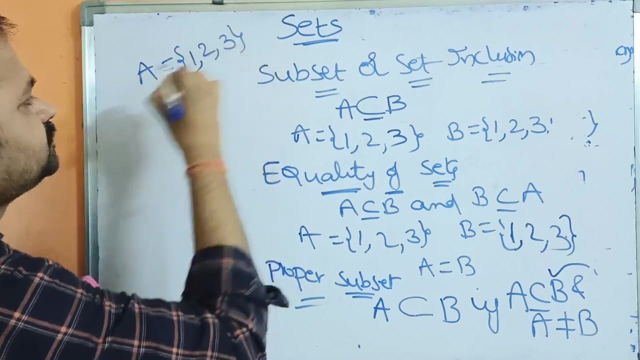 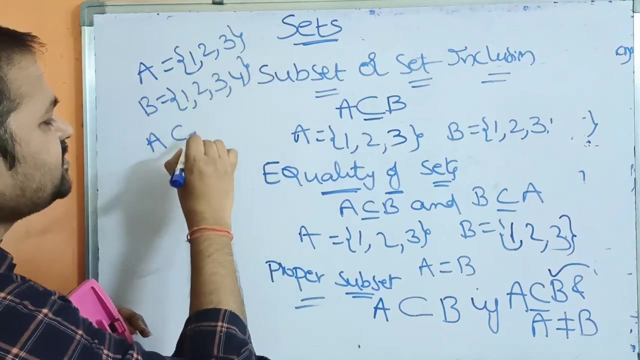 in b. yes, that condition is satisfied. next: a not equal to b. but here what is the problem? a and b are equal only so that means we can't say a proper subset b. okay, let us take one more example. let a is equal to, let a is equal to 1, 2, 3. b is equal to 1, 2, 3, 4. now can we say a proper subset b, can we? 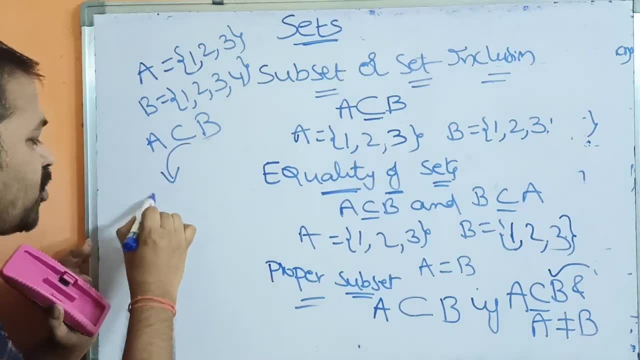 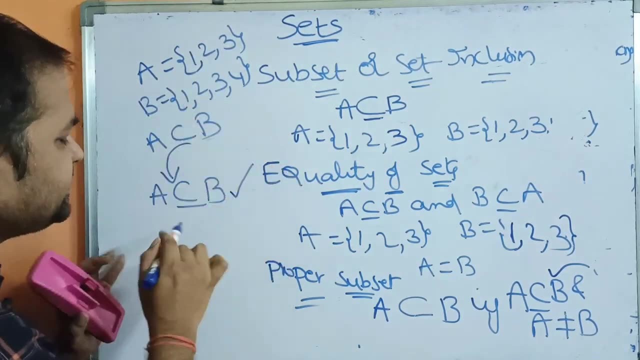 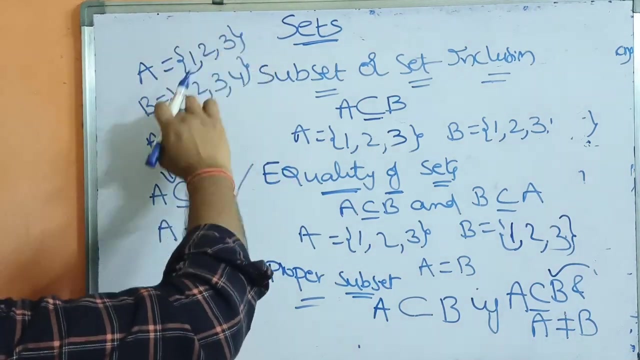 say a proper subset b. here it has to satisfy two properties. the first property is a subset b. that means every element of a must present in b. yeah, this condition is satisfied. and the second condition is a not equal to b. here a and b are not equal. okay, a contains 1- 2. 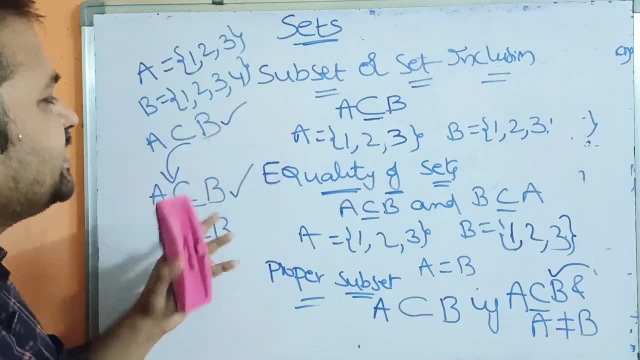 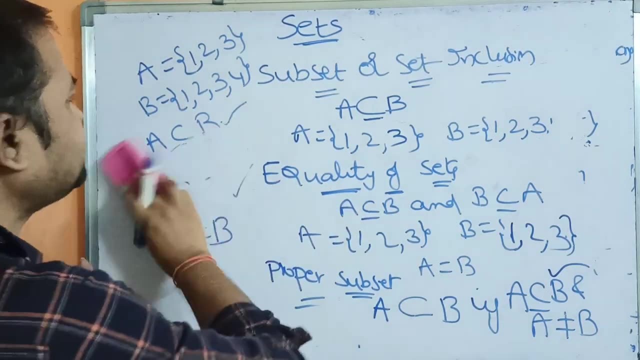 3 b contains 1, 2, 3, 4, 5, so we can say that a proper subset b. so this is about subset or set, inclusion and equality of two sets and proper subset. okay, now let us see about two more terminologies, such as: 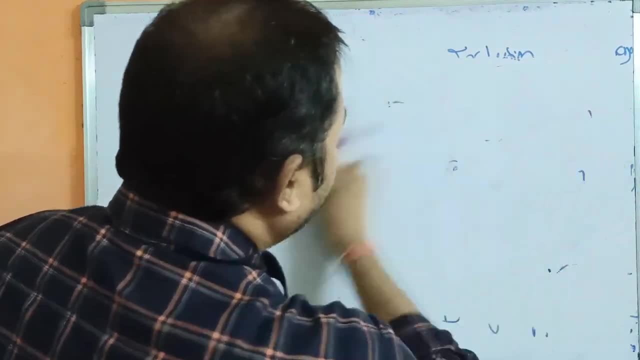 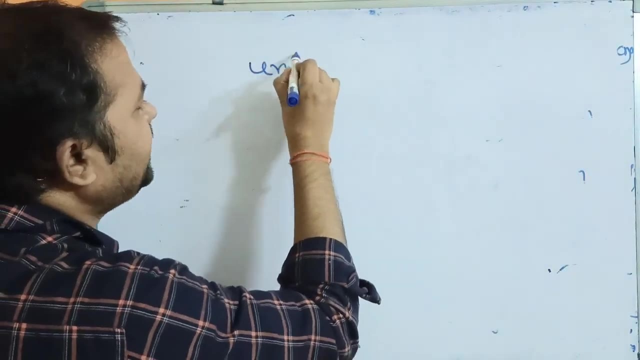 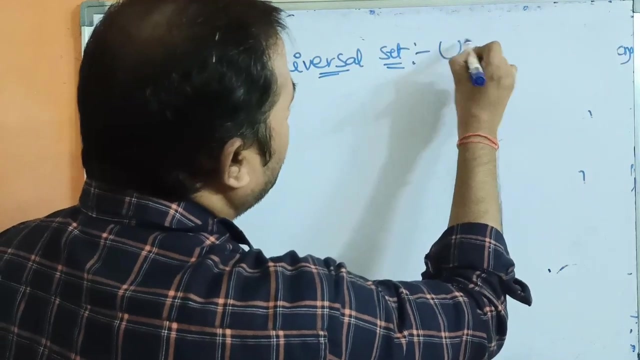 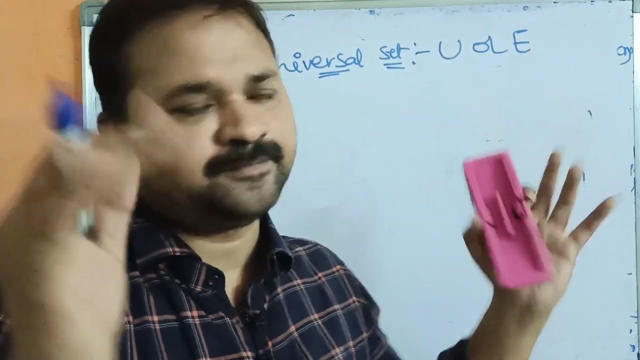 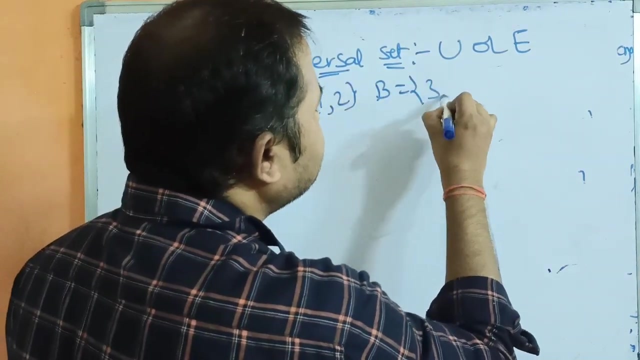 ah, such as universal set and empty set. first let us see about universal set. universal set is denoted by u, or we can use e also. Universal set means union of all the sets. Let we have three sets like this. Let a is equal to 1, 2. b is equal to 3, 4. c is equal to a- b. 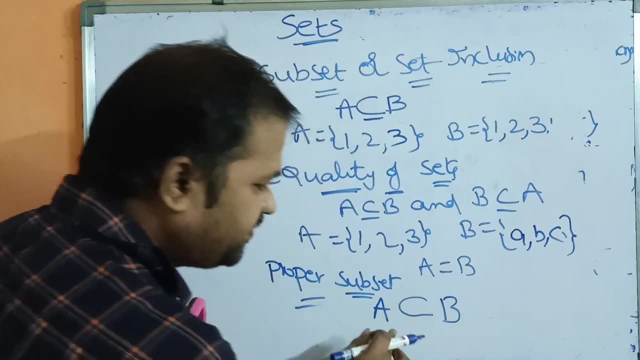 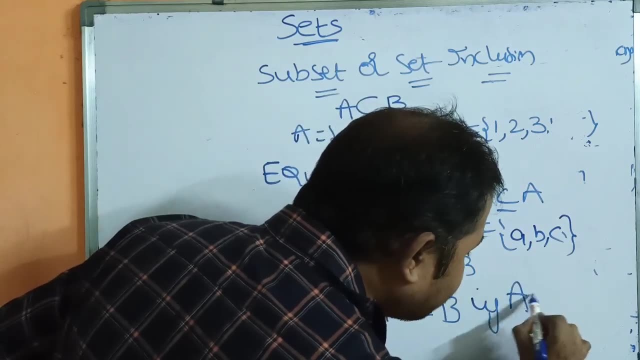 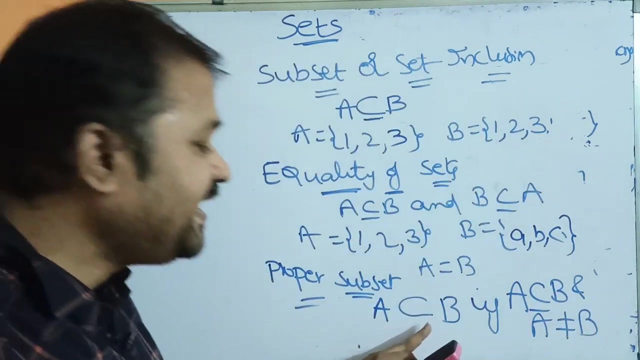 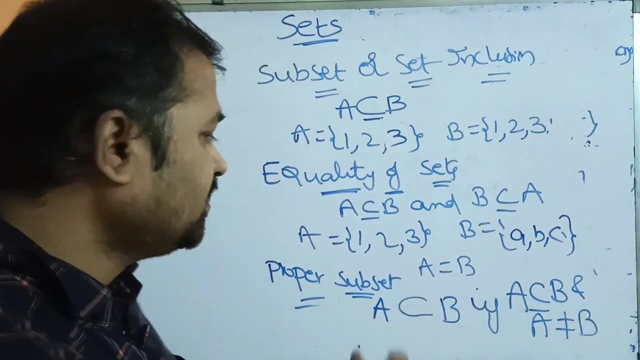 have equal operator. so this is nothing but proper subset b. we can say that a is a proper subset b if if a subset b and a not equal to b. so we can say that a proper subset b if a subset b as well as a not equal to b. so if we consider these, this example: a is equal to 1, 2, 3. 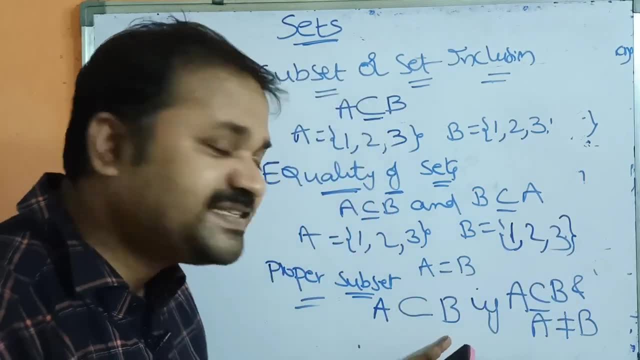 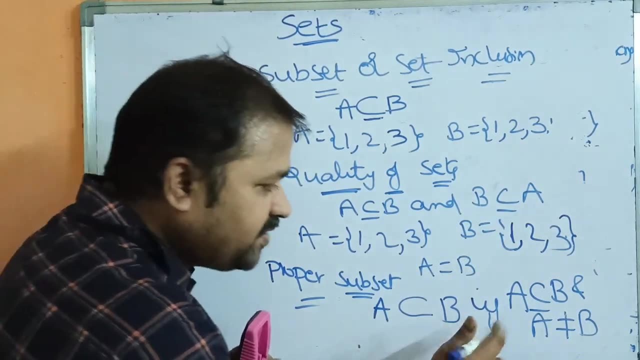 b is equal to 1,, 2,, 3.. Now can we say A subset B? We cannot say like that, Why? Because, I am sorry, can we say A proper subset B? No, Why? Because here, what is the first condition? A subset B, So that 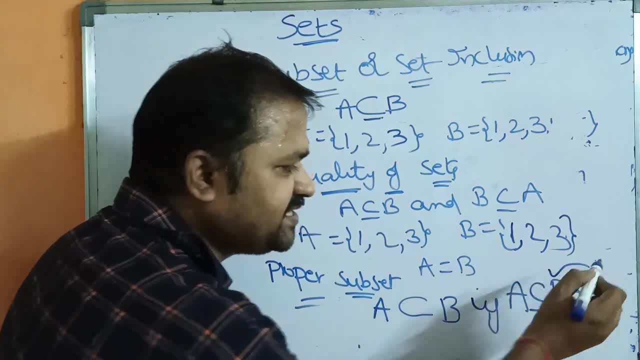 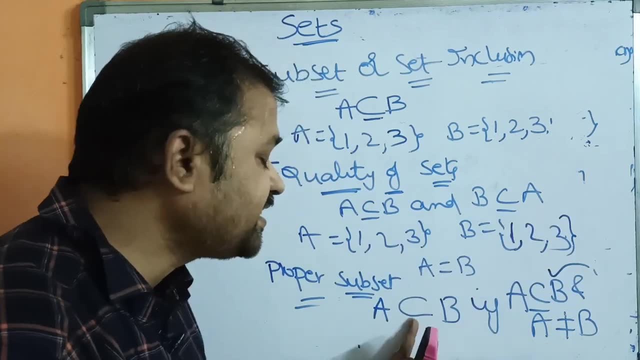 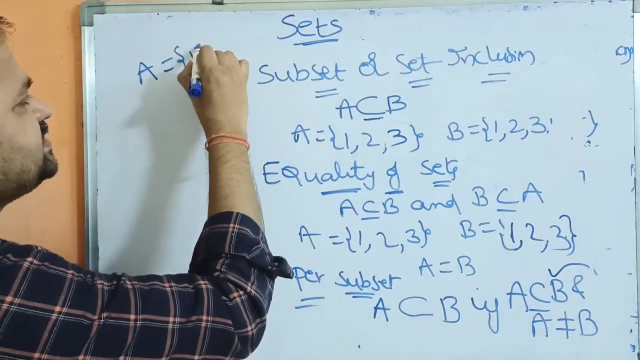 means every element of A must present in B. Yes, that condition is satisfied. Next: A not equal to B. But here what is the problem? A and B are equal only. So that means we cannot say A proper subset B. Let us take one more example. Let A is equal to 1, 2, 3.. B is equal to 1, 2, 3, 4.. Now can we? 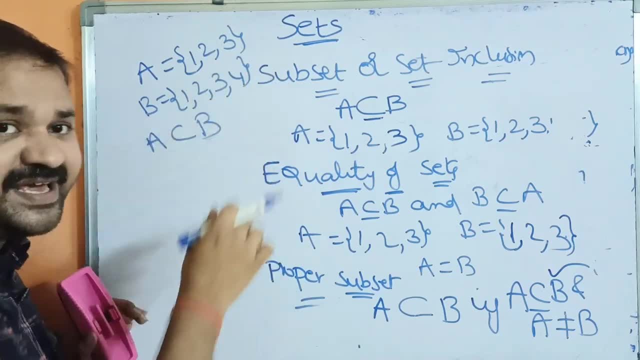 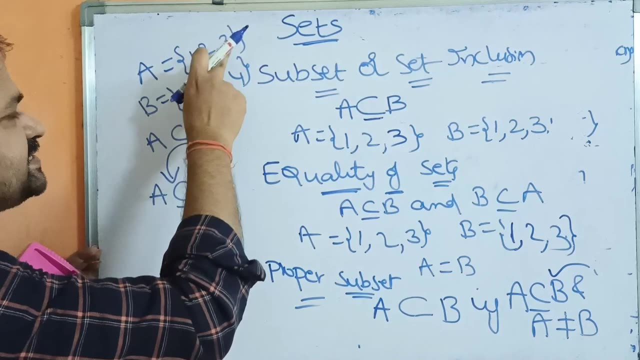 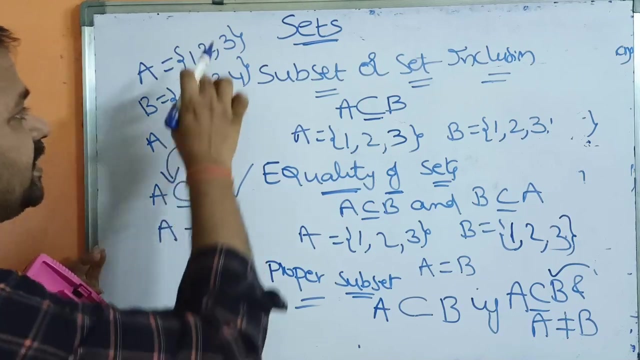 say A proper subset B. Can we say A proper subset B Here? it has to satisfy two properties. The first property is A subset B. That means every element of A must present in B. Yes, this condition is satisfied. And the second condition is A not equal to B Here A not equal to B. So that means 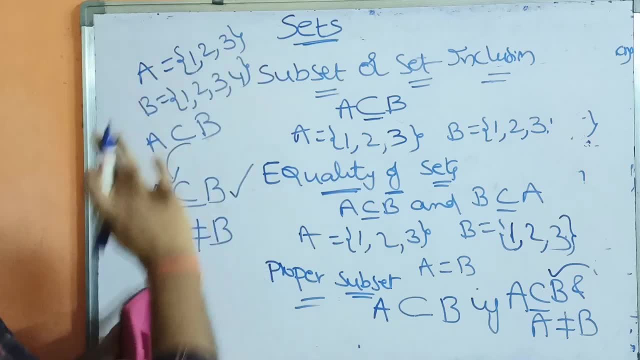 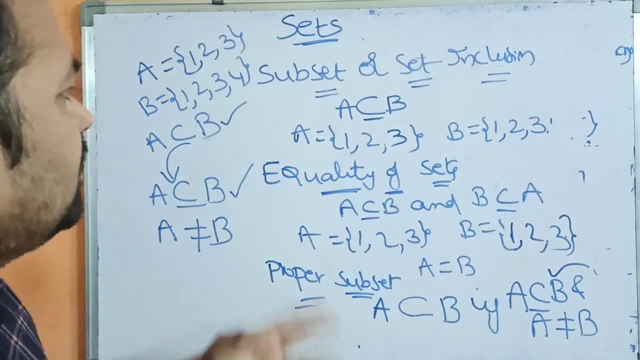 A and B are not equal. A contains 1, 2, 3.. B contains 1, 2,, 3,, 4, 5.. So we can say that A proper subset B. So this is about subset or set, inclusion and equality of two sets and proper. 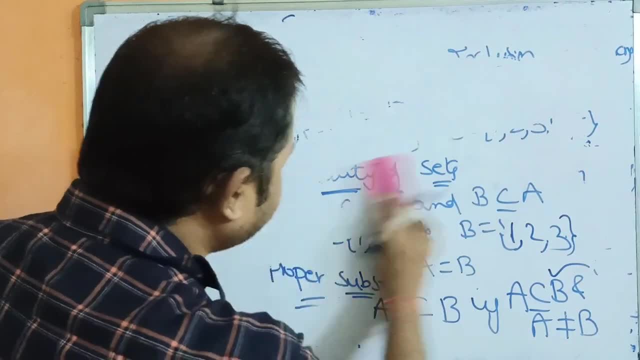 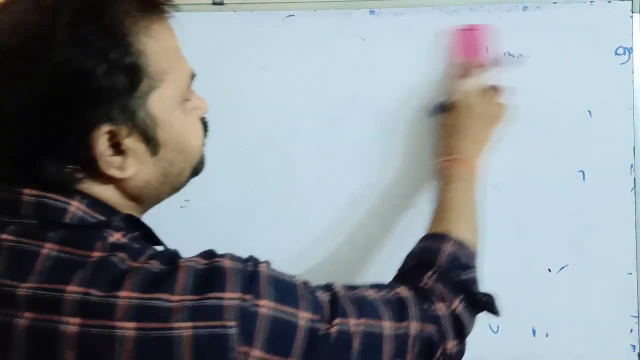 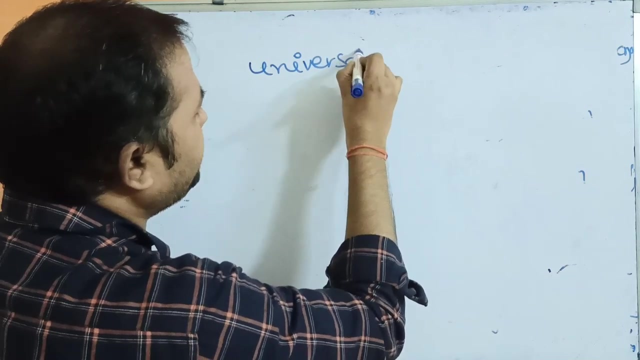 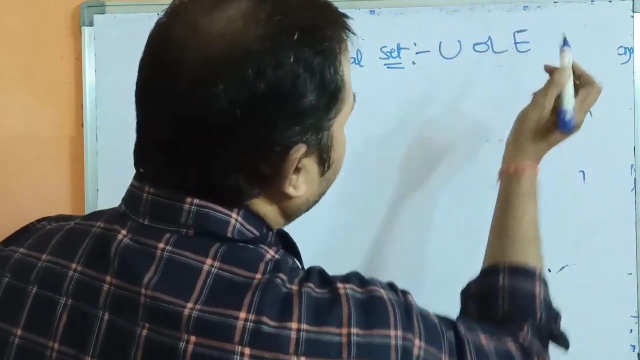 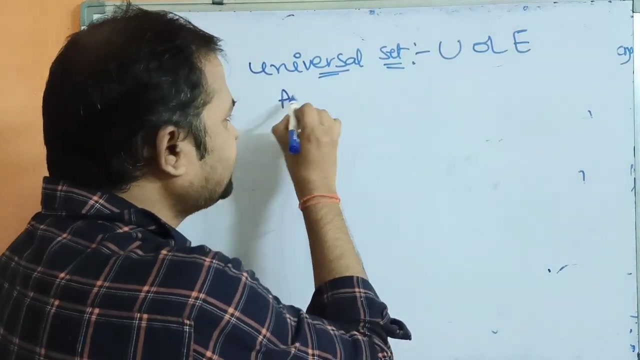 subset. Now let us see about two more terminologies, such as universal set and empty set. First let us see about universal set. Universal set is denoted by U, or we can use E also. Universal set means union of all the sets. Let we have three sets like this. Let A is equal to 1, 2. B is equal. 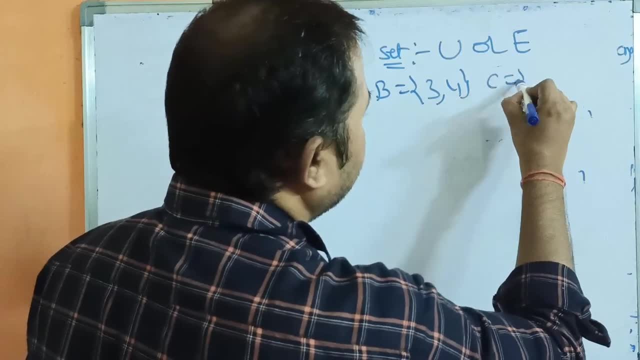 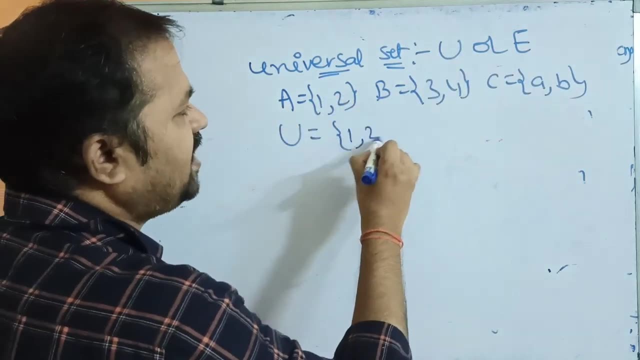 to 3, 4.. C is equal to A, B. Then we can say that universal set is nothing but union of all these sets, So 1,, 2,, 3,, 4.. So let us see about universal set First. let us see about universal set Universal. 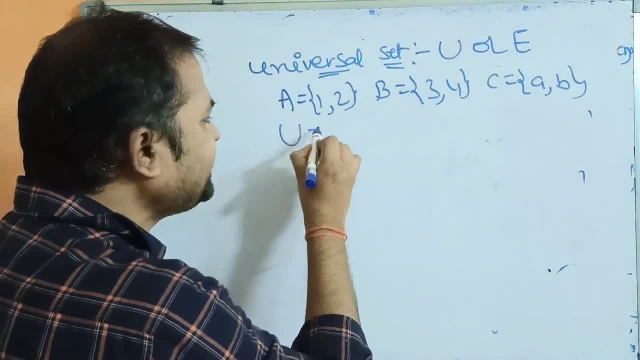 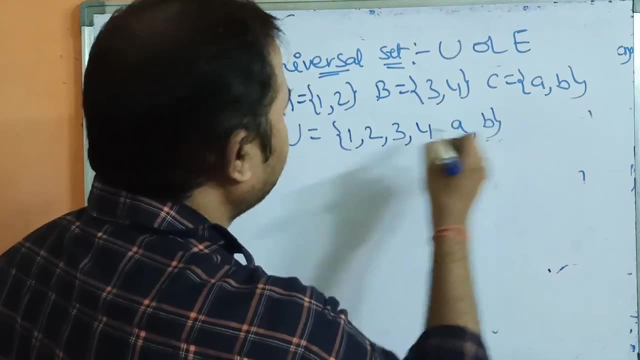 Then we can say that universal set is nothing but union of all these sets. So 1 comma, 2 comma, 3 comma, 4 comma, a comma b. So universal set is represented by u or e. Now let us see about. 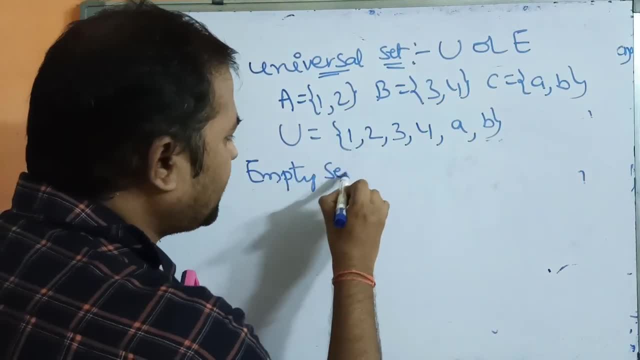 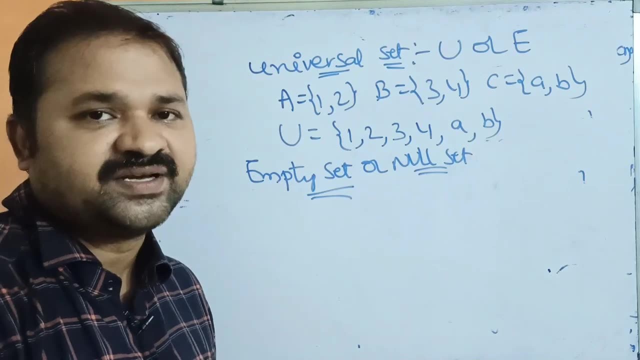 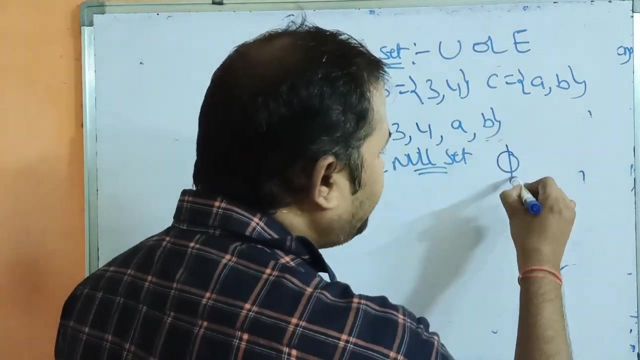 empty set or null set, Empty set or null set. So what is empty set? Empty set means if the set doesn't contains any elements. If the set doesn't contains any elements, then it is called as empty set. Empty set is denoted by the symbol pi. So here the example is: pi is equal to empty curly. 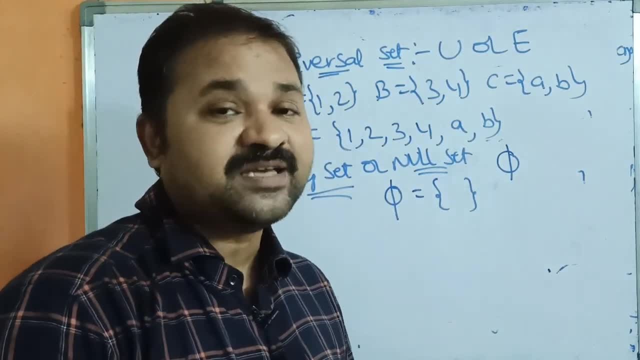 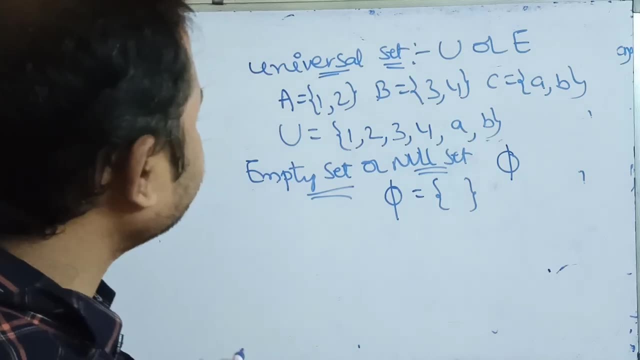 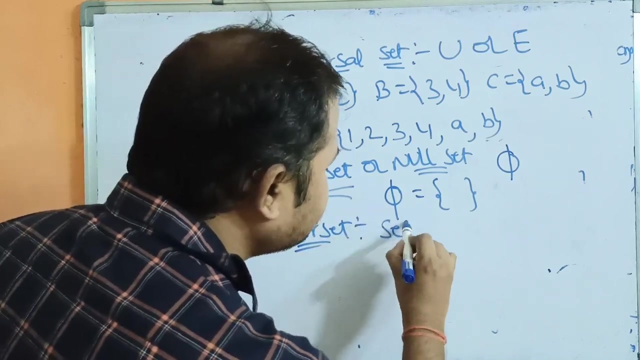 braces. So within the curly braces, no elements. Why? Because empty set means the corresponding set doesn't contain any elements. Now let us see one more: empty set is over. Now let us see one more terminology, that is power set. Power set means set of all subsets. Power set means set. 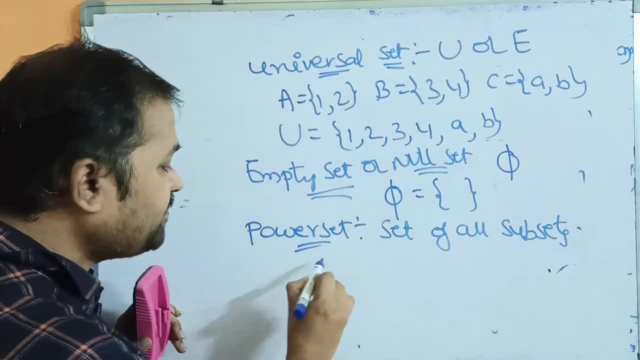 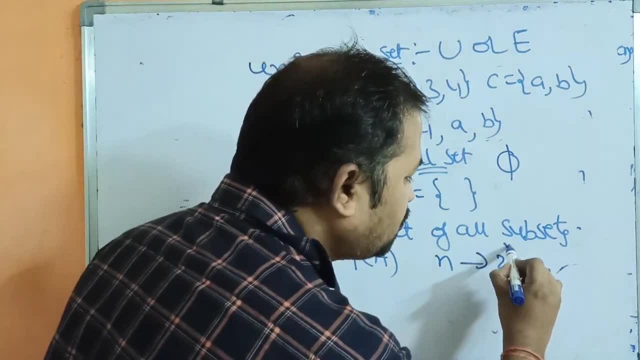 p of a. So if the set contains, then it is called as p of a. So if the set contains, then it is called as n elements. Then power set totally contains two power n elements. That means, if the set 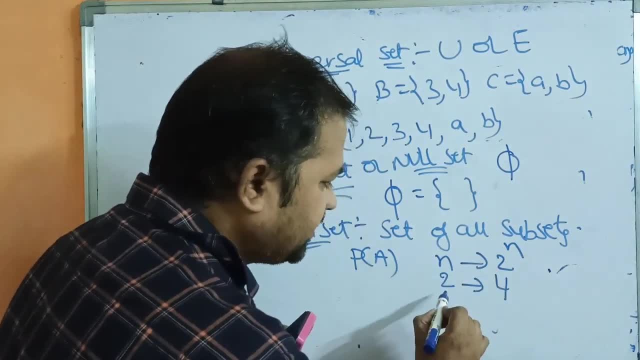 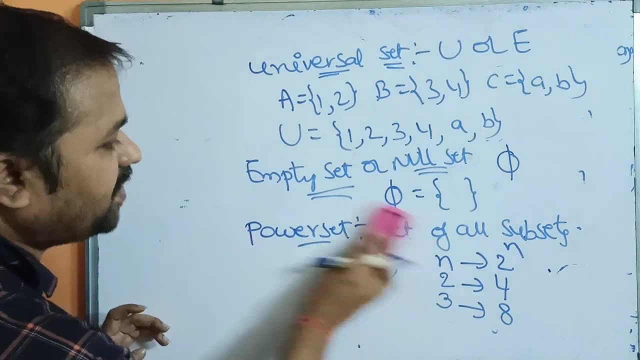 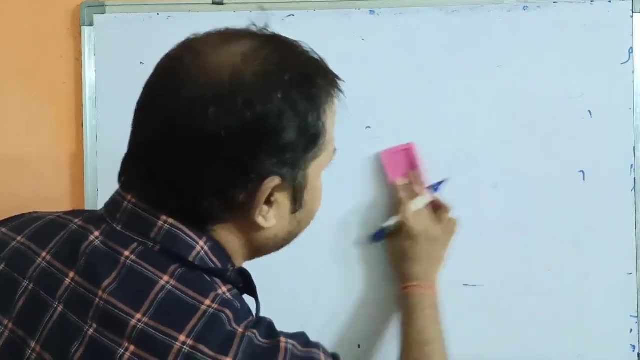 contains two elements, then power set contains four elements. If the set contains three elements, then power set contains two, power three, eight elements. So power set means set of all subset. Now let us see an example for the power set Power set. let us take two examples In the 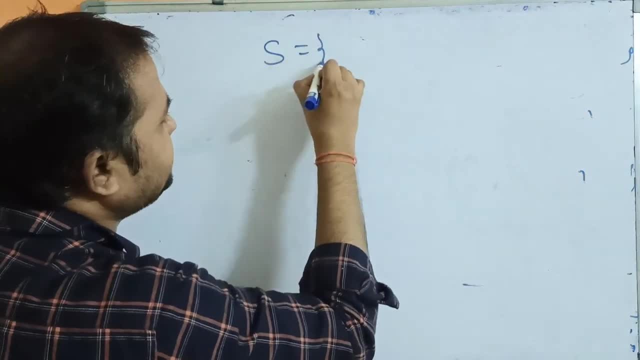 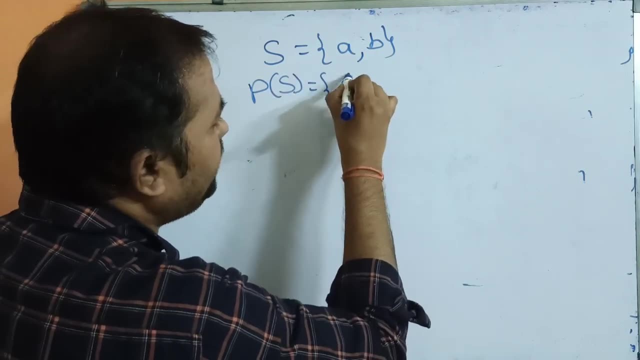 first example take two elements. So let we have a set like this: s is equal to a comma b, Then P of S, power set of S is equal to here. first we have to take pi, So pi is the minimum subset. 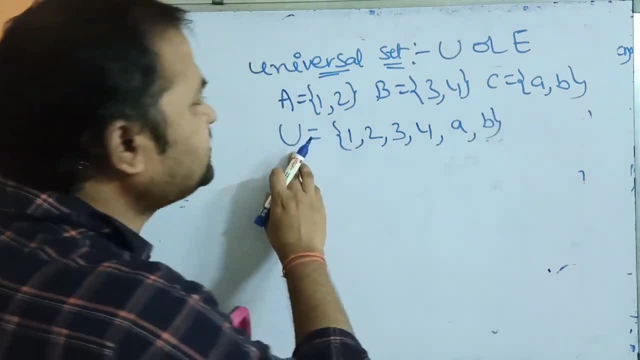 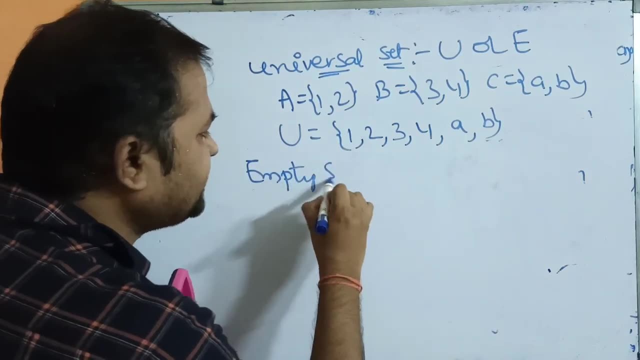 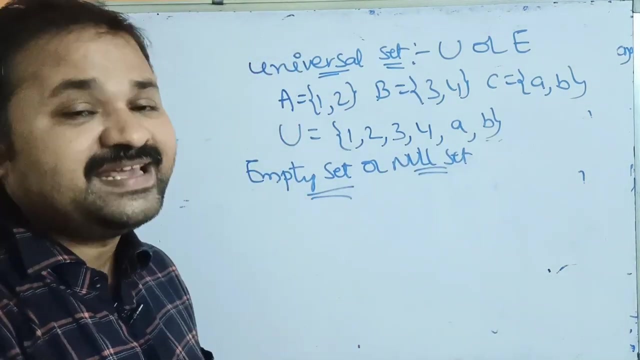 set is half set: 1,, 2,, 3,, 4,, A, B. So universal set is represented by U or E. Now let us see about gloomy or null set. O means empty set means if the set does not contains any elements, then it is called as empty set, Empty set. 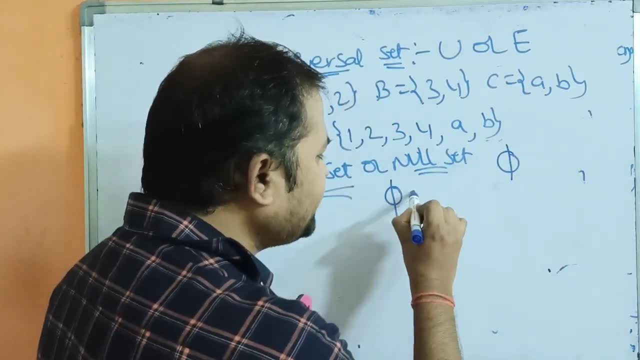 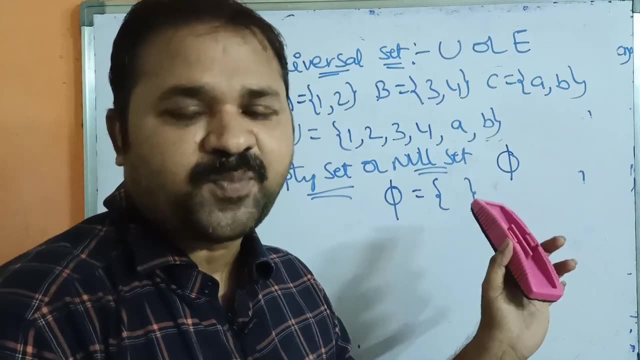 is denoted by the symbol PI. So here the example is: PI is equal to empty curly braces. And then Nh. one sixteenth discussion is discussed here. Hello, Closure, Jai, Greetings from the N persecuted Burke School of doctor, homemade curly braces. so within the curly braces no elements. why? because empty set means the corresponding set. 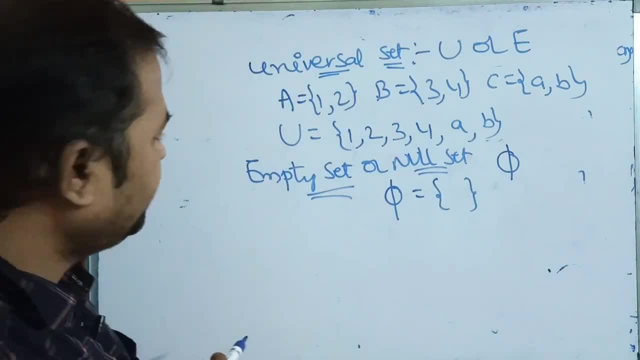 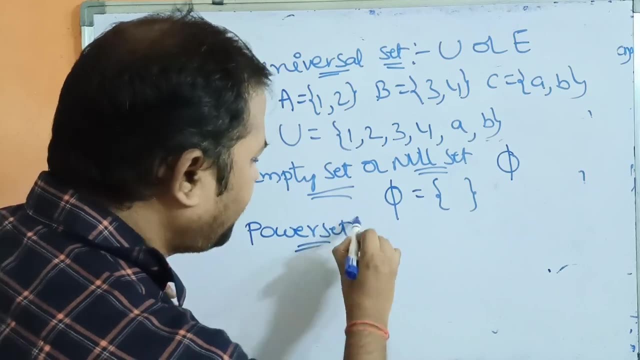 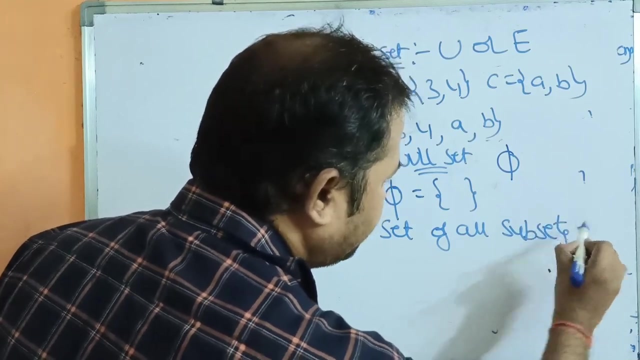 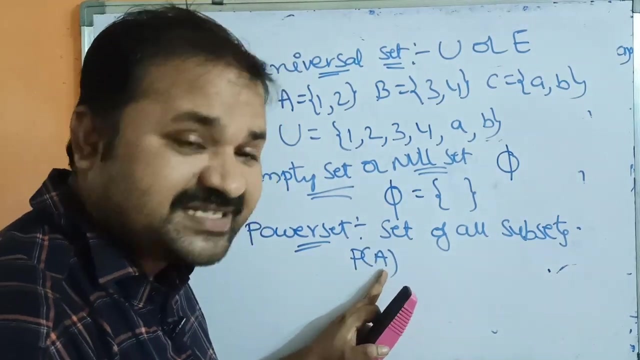 doesn't contain any elements. now let us see one more empty set is over. now let us see one more terminology, that is power set. power set means set of all subsets. power set means set of all subsets. power set is denoted by the symbol p of a, suppose if the set contains, if the set a contains n. 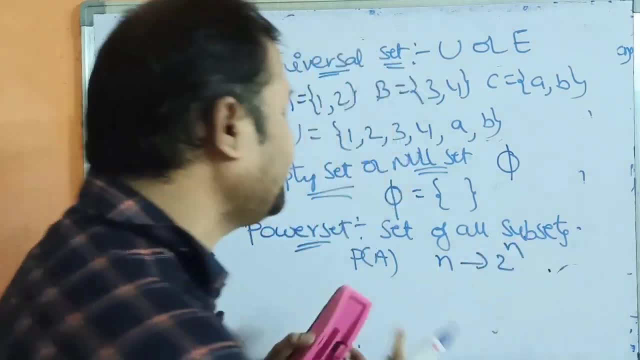 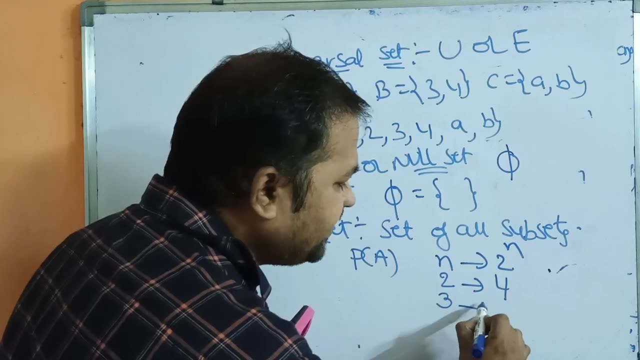 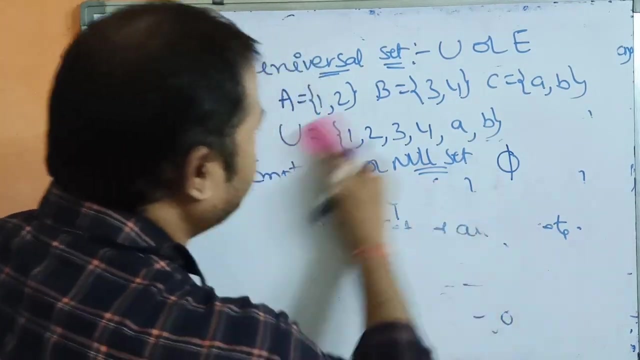 elements, then power set totally contains two power n elements. that means, if the set contains two elements, then power set contains four elements. if the set contains three elements, then power set contains two, power three, eight elements. so power set means set of all subset. now let us see an. 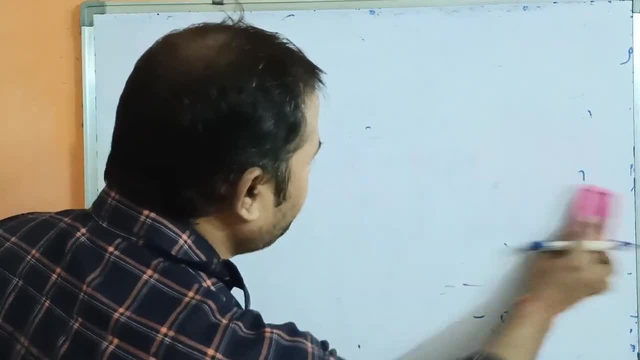 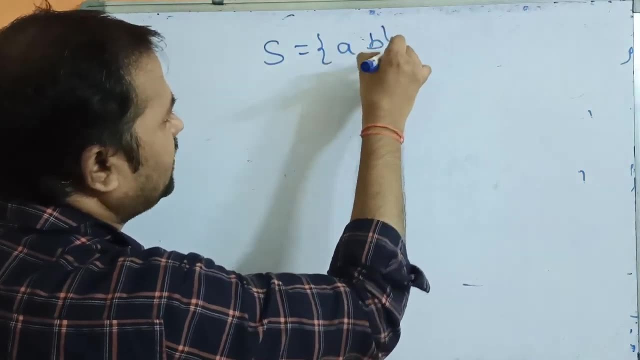 example for the power set, Power set. Let us take two examples. In the first example take two elements. So let we have a set like this: S is equal to A, comma B, Then P of S- power set of S- is equal to. 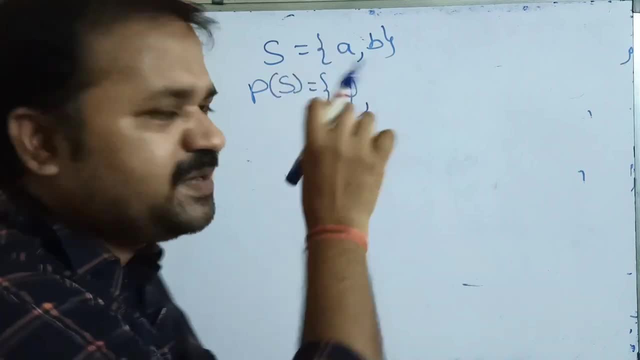 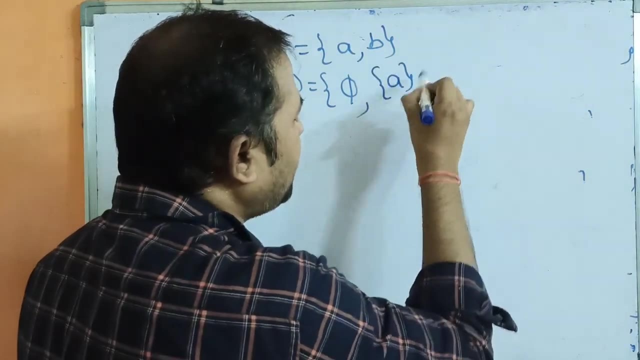 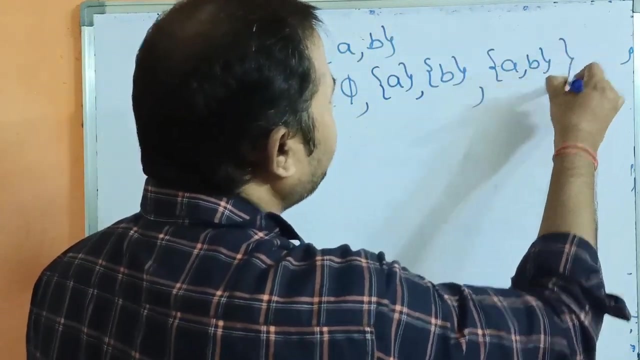 here. first we have to take pi, So pi is the minimum subset. Next we have to take a set which contains a single element. Single element set means A comma B. Next take a set with two elements, So A comma B. So here, how many elements are there? 1,, 2,, 3,, 4.. Here 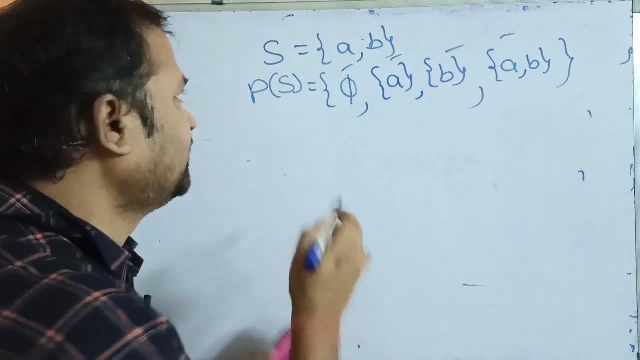 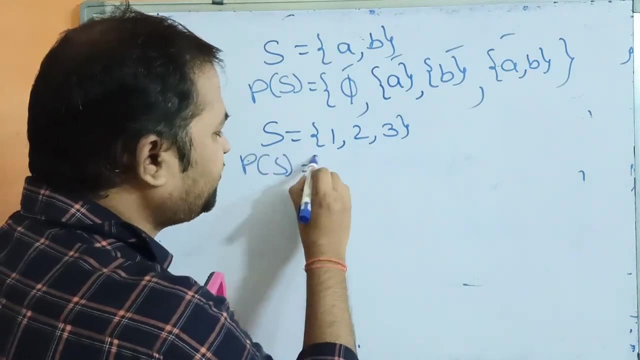 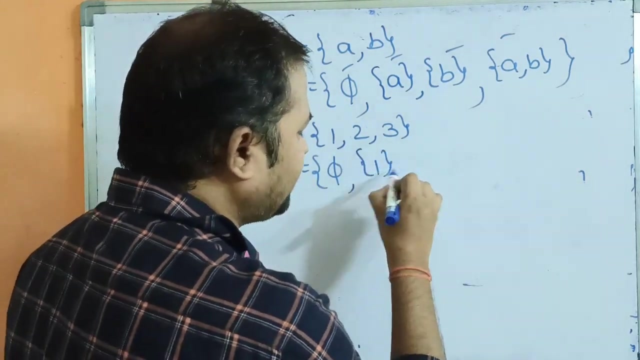 the set contains two elements, So power set contains four elements. Now let us take one more example. S is equal to 1 comma, 2 comma 3.. Then P of S is equal to, so here the minimum subset is pi comma. Next, here the set contains three elements, So we have to take the set. 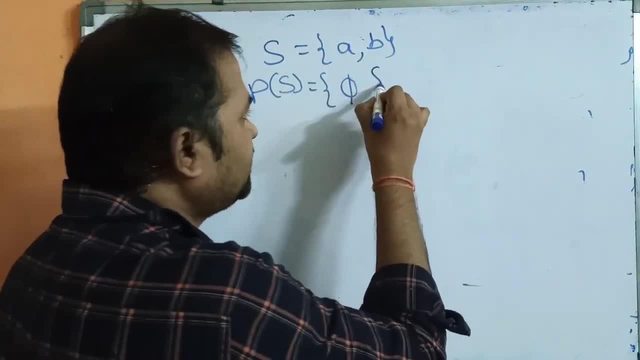 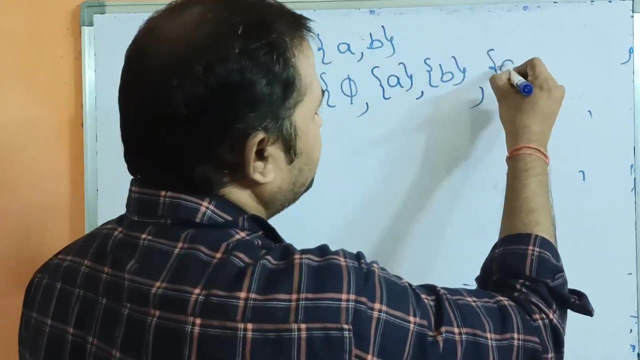 Next we have to take a set which contains a single element. Single element set means A, B. Next take a set with two elements, So A, B. So here how many elements are there? 1,, 2,, 3,, 4.. 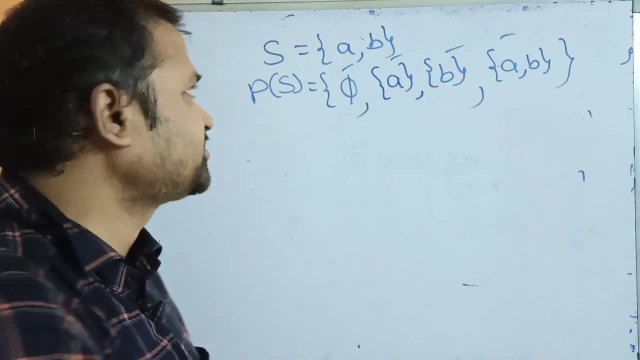 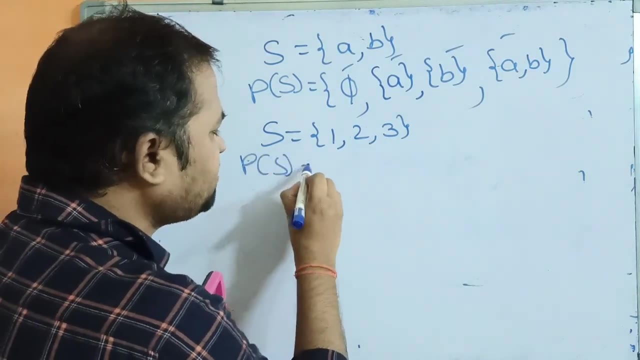 Here the set contains two elements, So power set contains four elements. Now let us take one more example. S is equal to 1,, 2,, 3.. Then P of S is equal to, so here the minimum subset is pi. 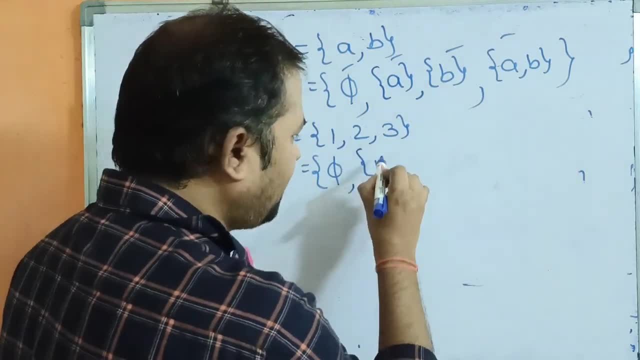 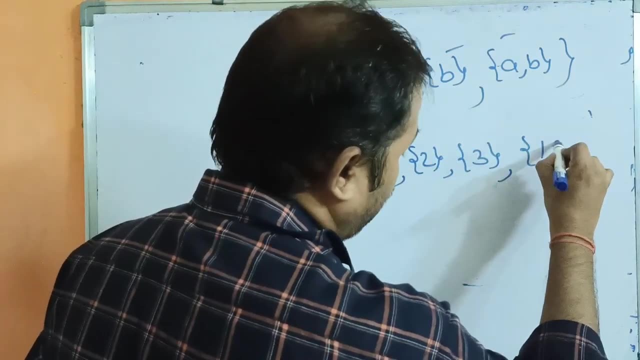 Next here, the set contains three elements, So we have to take the set with only one term, So 1,, 2, 3.. Now let us take the set with two terms, So 1, 2, 1, 3,, 2, 3.. 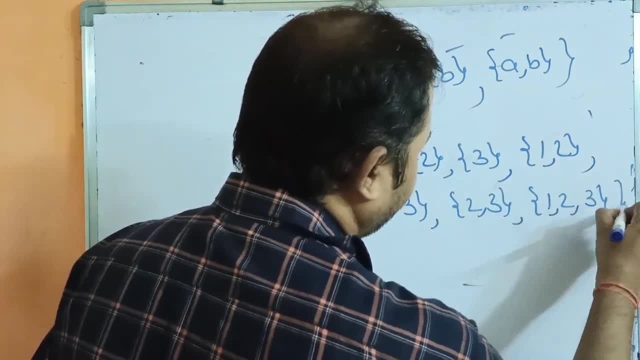 Next set with three elements. So only one, Only one combination: 1, 2, 3.. Okay, So if you consider here 1, 2,, 3, 4,, 5,, 6,, 7, 8.. 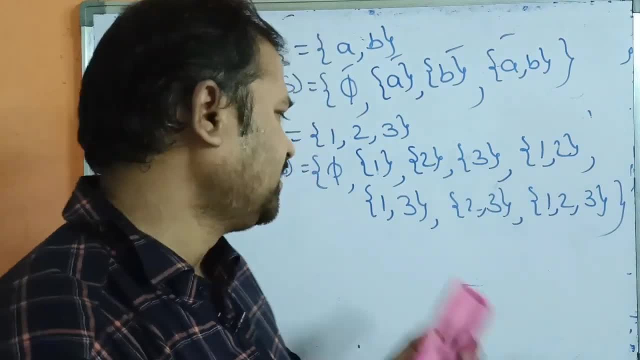 Eight elements. Here we have 1, 2.. So there is no need to take 2, 1.. Here we have 1, 3.. There is no need to take 3, 1.. Here we have 2, 3.. 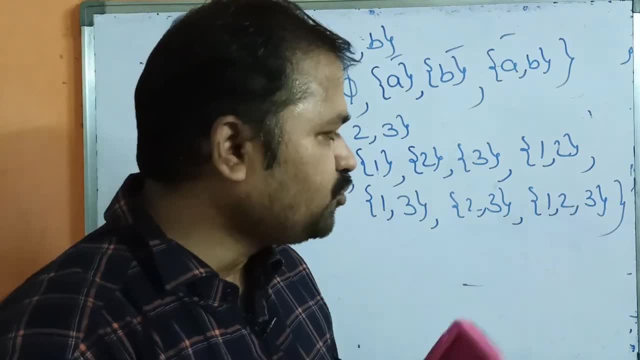 There is no need to take 2, 3.. 3, 2.. Here we have 1,, 2, 3.. So there is no need to take 2, 3, 1, 2, 1, 3, 3, 1, 2, 3,, 2, 1.. 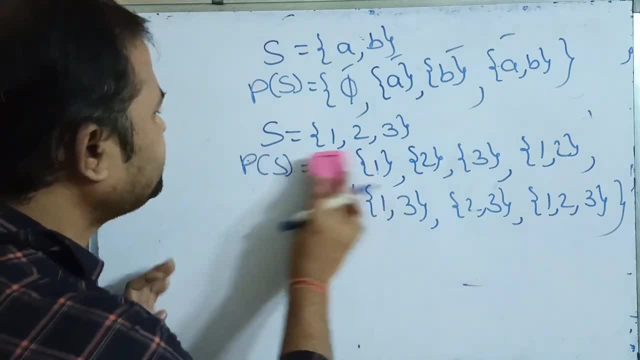 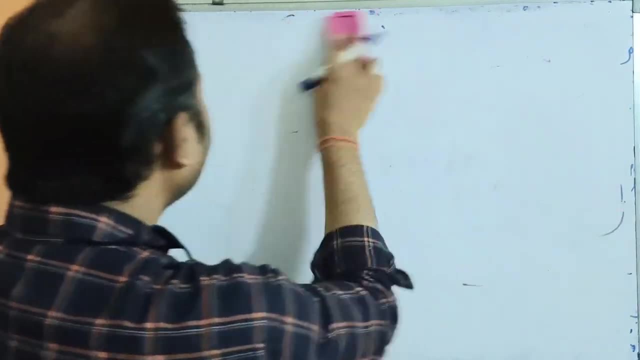 Okay, So this is nothing but power set. So these are the various terminologies regarding the set. Now let us see about set operations. Set operations: We can perform various operations on the set. Mainly, we can perform seven operations. 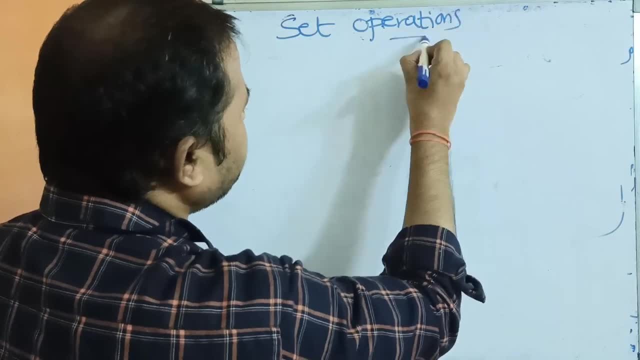 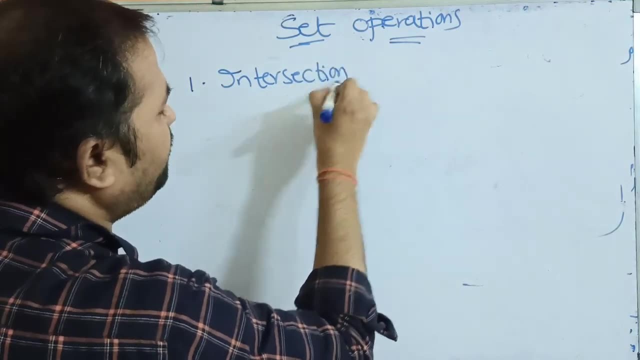 Let us see all the operations one by one. The first operation is intersection. So what is intersection? Intersection is denoted by the symbol reverse of U, or we can use this is nothing but intersection, Okay. Or we can use reverse of V also. 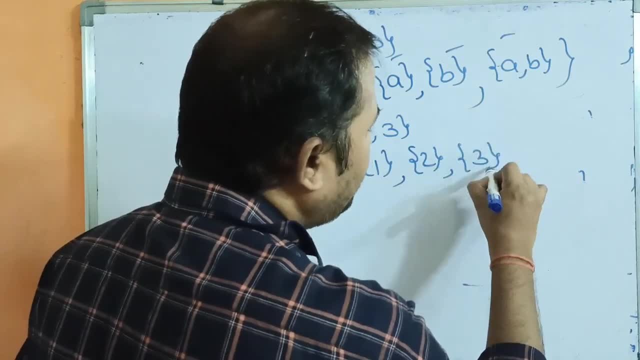 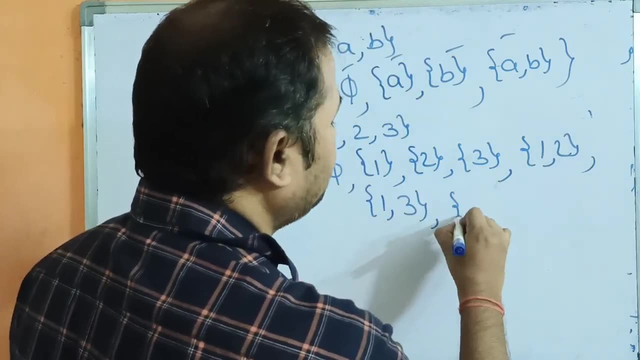 with only one term, So 1 comma, 2 comma, 3.. Now let us take a set with only one term, So 1 comma, 2 comma 3.. Now let us take a set with two terms, So 1 comma, 2 comma, 1 comma, 3 comma, 2 comma, 3.. Next, a set with three. 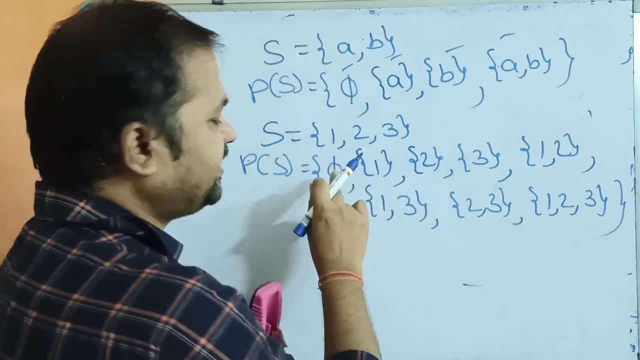 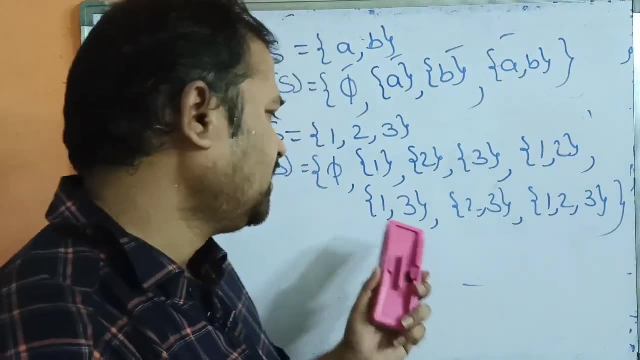 elements, So only one combination: 1,, 2, 3.. So if you consider here 1,, 2,, 3,, 4,, 5,, 6,, 7,, 8,, eight elements, Here we have 1, 2. So there is no need to take 2, 1. Here we. 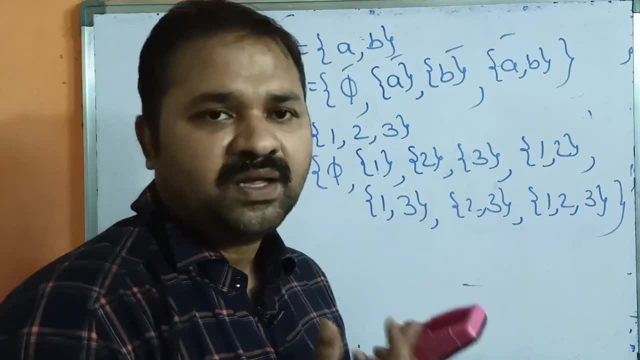 have 1, 3.. There is no need to take 3, 1.. Here we have 2, 3.. There is no need to take 2, 3.. 3, 2.. Here we have 1,, 2, 3.. So there is no need to take 2, 3, 1, 2, 1, 2, 3, 2,. 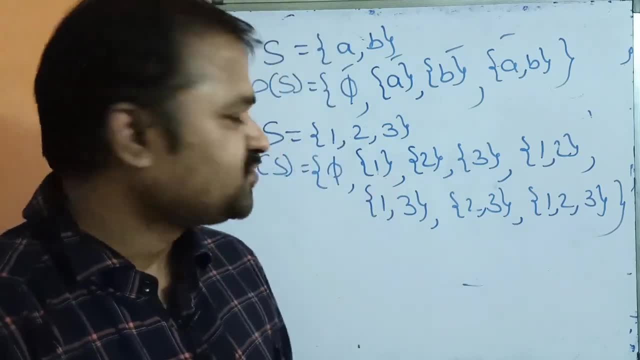 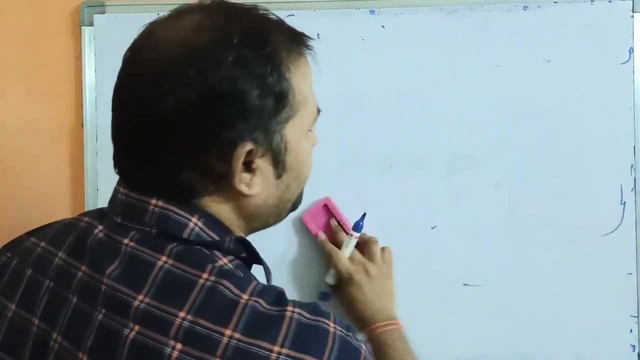 1, 3, 3, 1, 2, 3, 2, 1.. So this is nothing but power set. So these are the various terminologies regarding the set. Now let us see about set operations. Set operations We can perform. 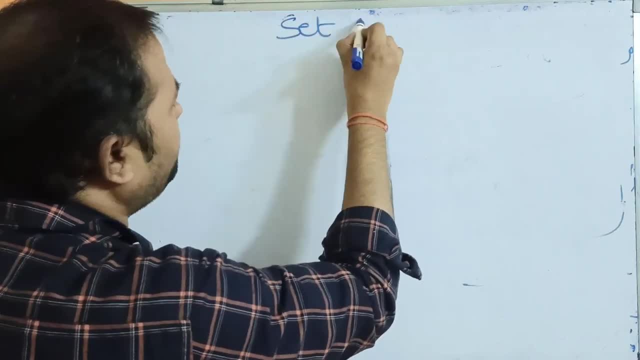 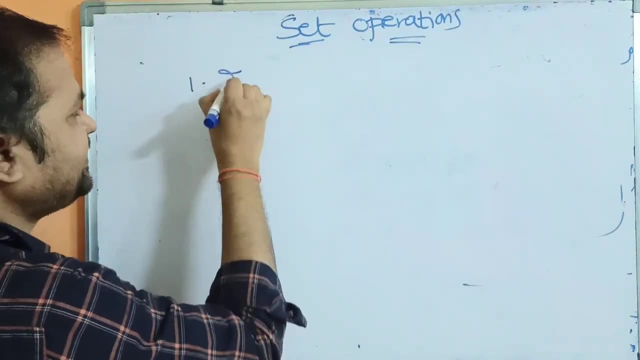 various operations on the set. Mainly we can perform seven operations. Let us see all the operations one by one. The first operation is intersection. So what is intersection? Intersection is denoted by the symbol reverse of U, or we can use 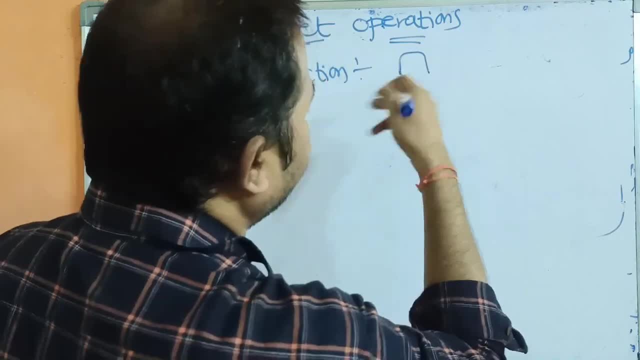 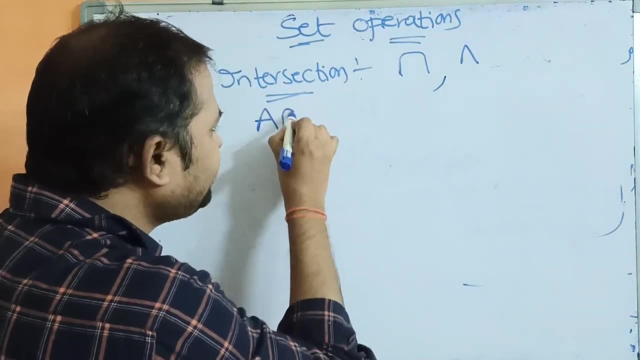 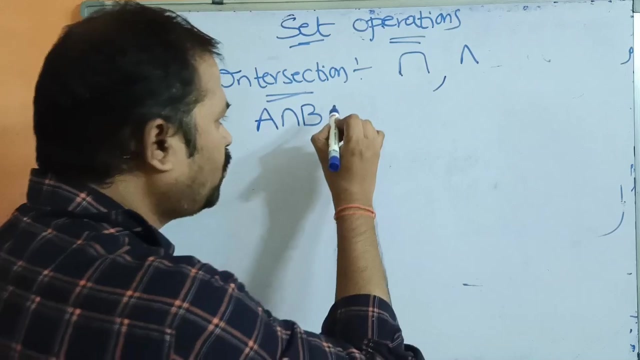 this is nothing but intersection. Or we can use reverse of V also. We can use this symbol also. Let we have two sets such as A- B. Then the intersection of A and B is denoted by A and B In symbolically. we can represent like this: So A and B is equal to. we can. 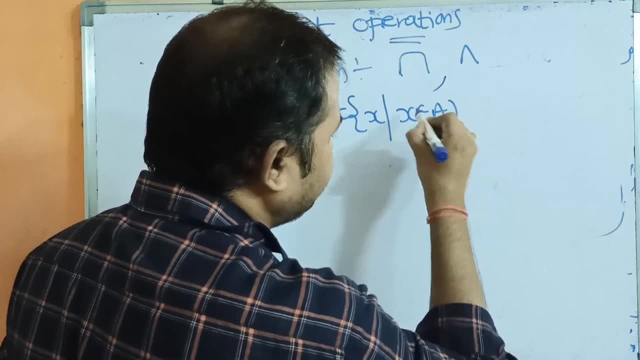 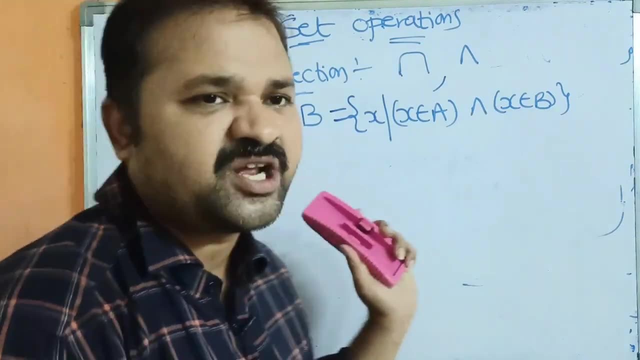 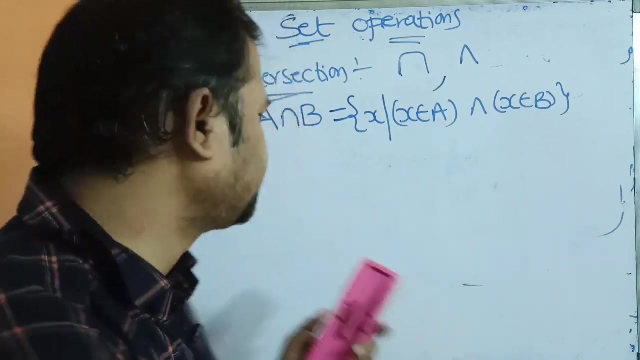 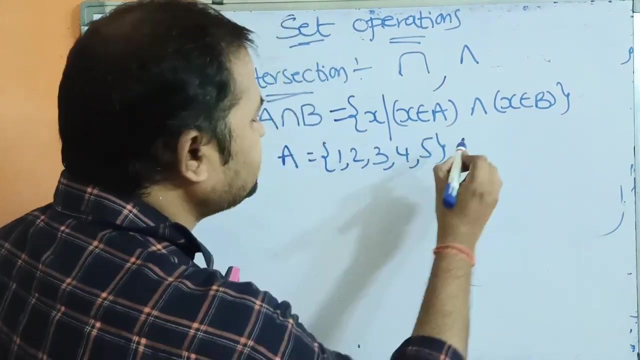 write as X, such that X belongs to the first set, that is, A, and X belongs to the second set, B. So what is intersection? Intersection means the common elements of both the sets. Intersection means the common elements of both the sets. Let we have A. A is equal to 1,, 2,, 3,, 4, 5.. Let B is equal to 3,, 5,, 6,. 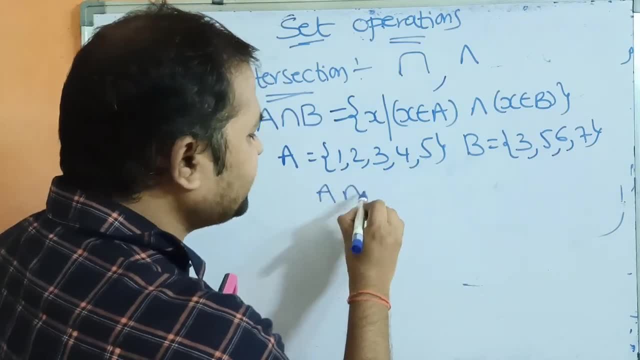 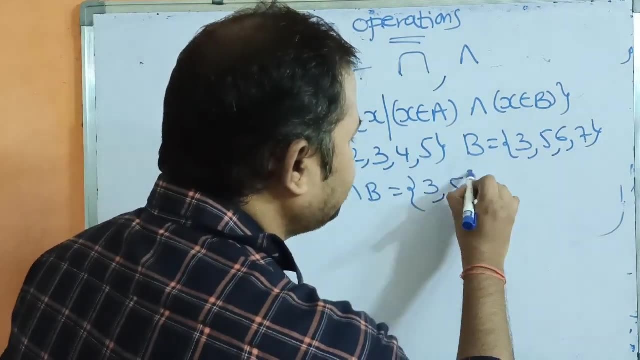 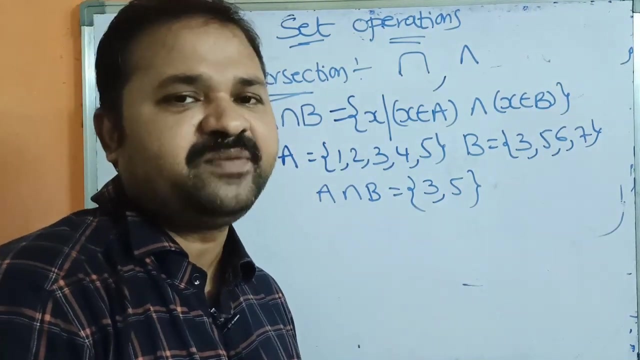 7.. Then what is A intersection B? A intersection B means the common elements present in both A and B. So what are the common elements? 3, 5.. So we can say that A intersection B is equal to 3, 5.. A intersection B is similar to B intersection A. B intersection A means: 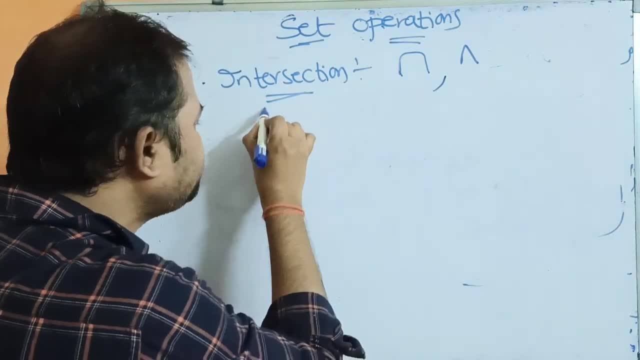 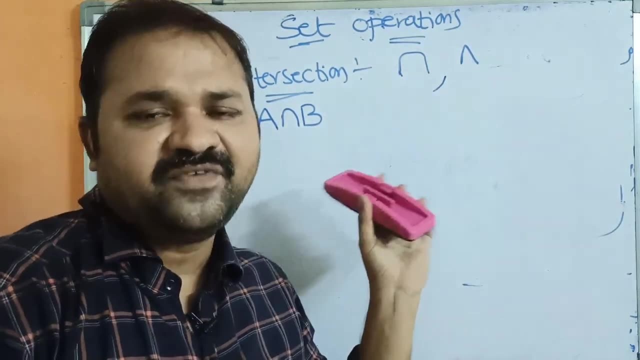 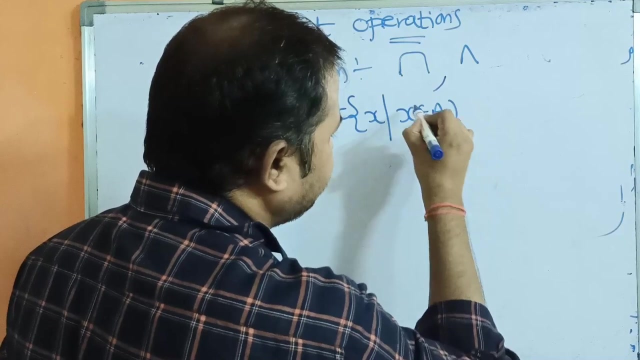 We can use this symbol also. Let we have two sets such as A- B. Then the intersection of A and B is denoted by A and B In symbolically we can represent like this: So A and B is equal to. we can write as X, such that X belongs to the first set, that is, A, and X belongs to the second set, B. 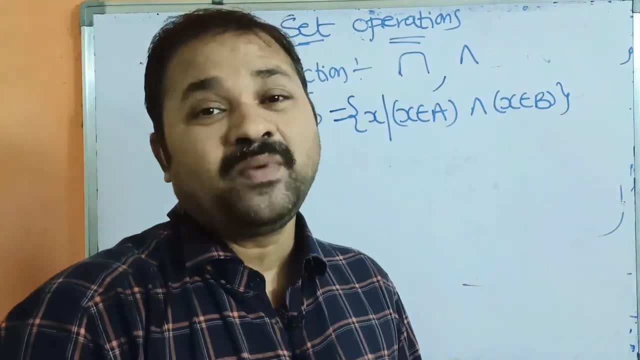 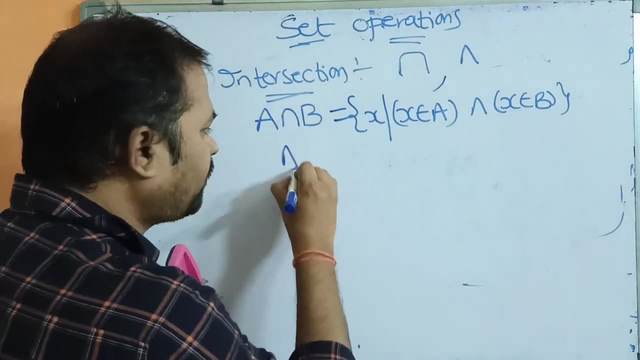 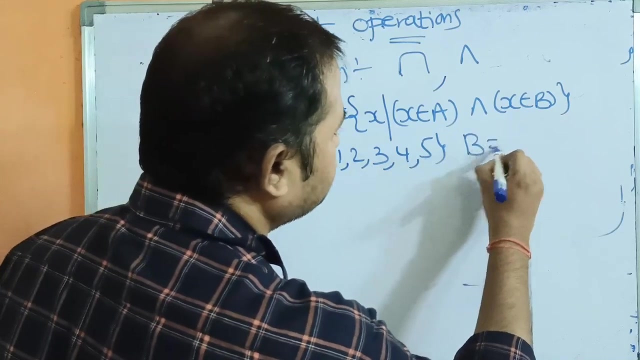 So what is intersection? Intersection means the common elements of both the sets. Intersection means the common elements of both the sets. Let we have A. A is equal to 1,, 2,, 3., 4,, 5.. Let B is equal to 3,, 5,, 6,, 7.. 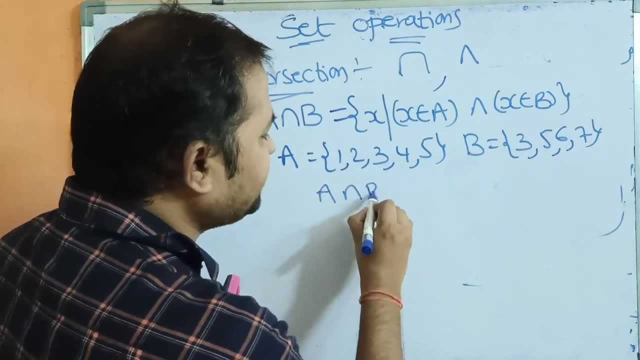 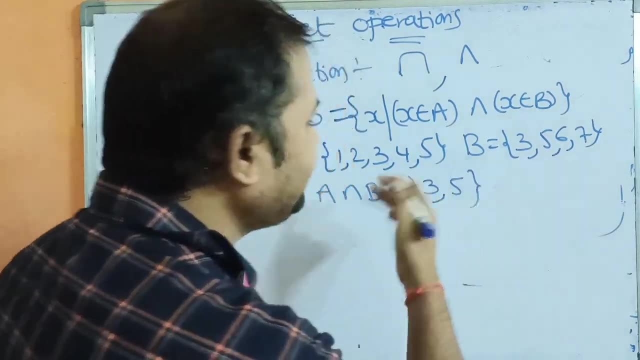 Then what is A intersection B? A intersection B means the common elements present in both A and B. So what are the common elements? 3, 5.. So we can say that A intersection B is equal to 3, 5.. 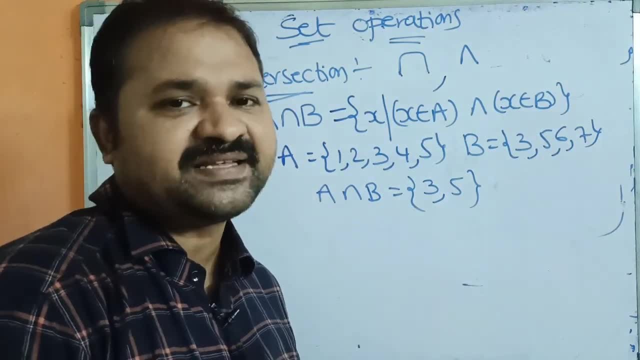 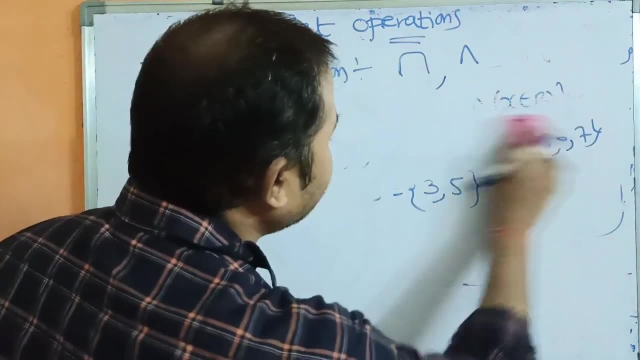 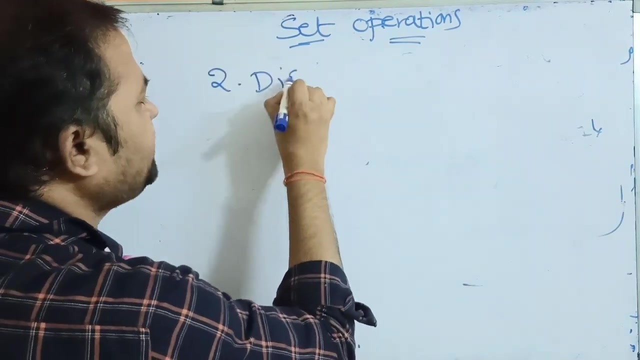 A intersection B is similar to B intersection A. B intersection A means the common elements of B and A. Okay, So this is about intersection operation. Now let us see the second operation. The second operation is disjoint operation. The second operation is disjoint operation. 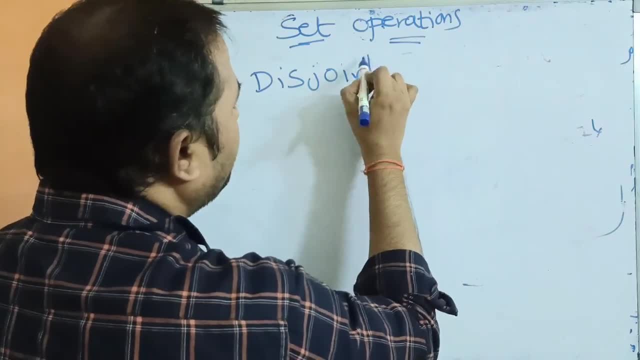 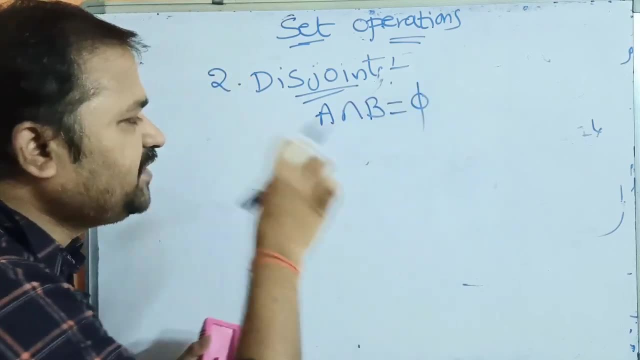 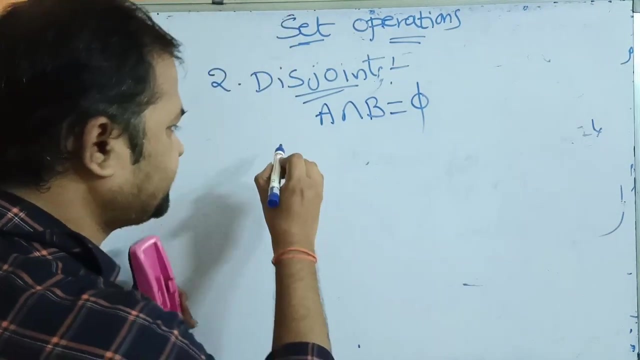 Two sets are said to be disjoint. Two sets are said to be disjoint if A intersection B is equal to pi. That means, if the sets A and B doesn't have any common element, then we can say that those two are disjoint sets. Let we have two sets such as A is equal to 1, 2.. 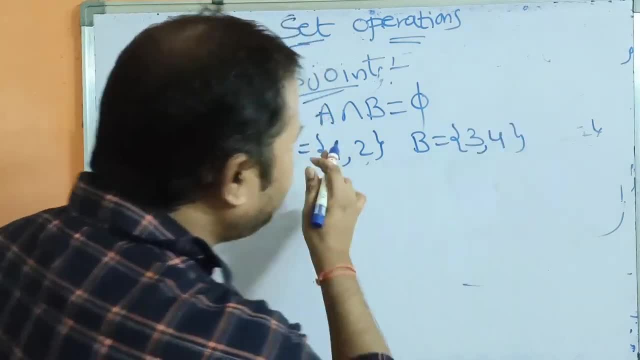 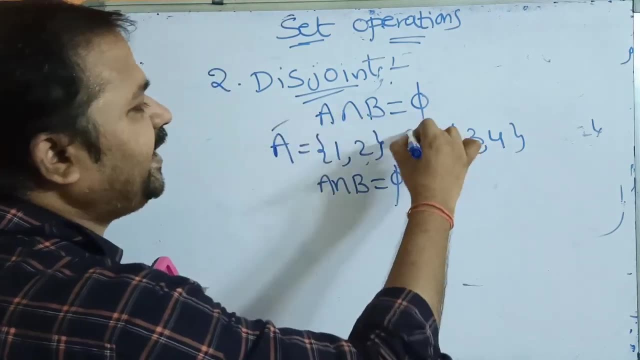 B is equal to 3, 4.. Here in A and B we don't have any common element. So we can say that A and B is equal to pi. So we can say that these two, A and B, are disjoint sets. 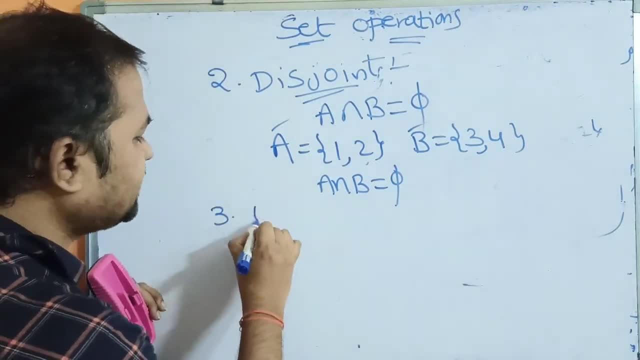 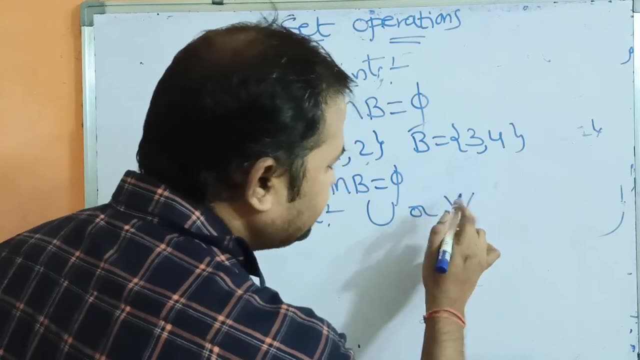 Okay, Disjoint sets. Now let us see about the third operation, That is, union operation. Okay, So union means we use U symbol, or we can use this: V also Okay, V also Okay, Okay. So this is denoted with the help of this symbol. 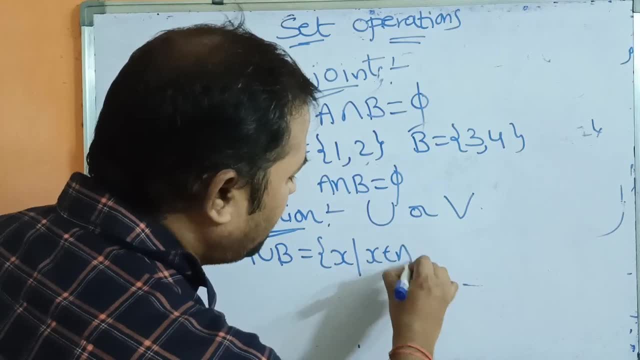 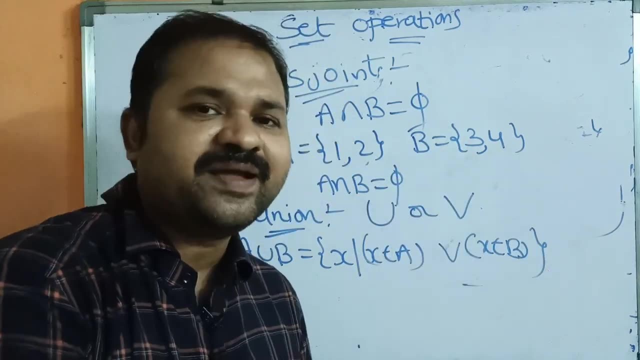 A union. B is equal to X, such that X belongs to A or R symbol. So X belongs to B. So union means it contains the elements of A or the elements of B. That means it contains the elements of A as well as the elements of the B. 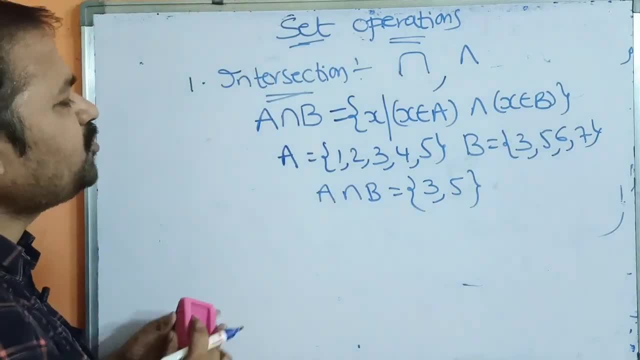 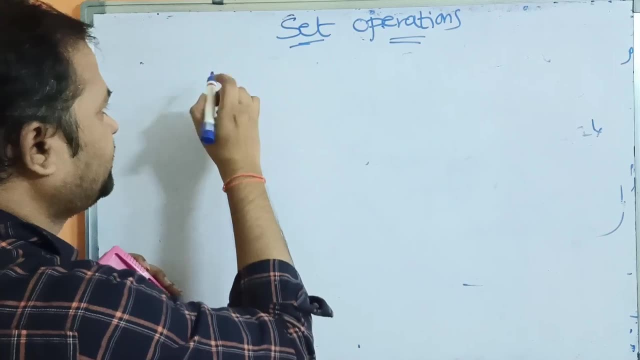 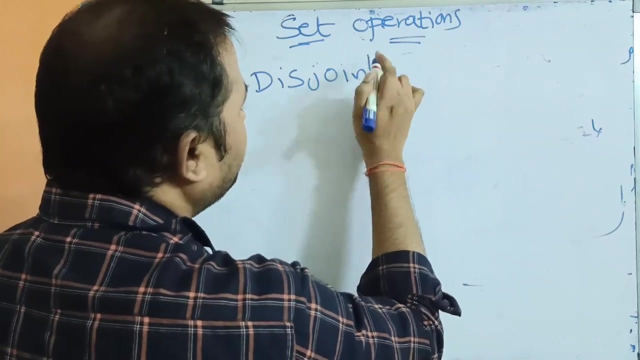 the common elements of B and A. So this is about intersection operation. Now let us see the second operation. The second operation is disjoint operation. The second operation is disjoint operation. Two sets are said to be disjoint. Two sets are said to be disjoint. 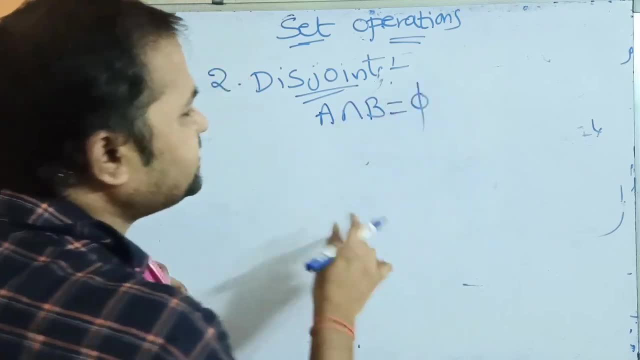 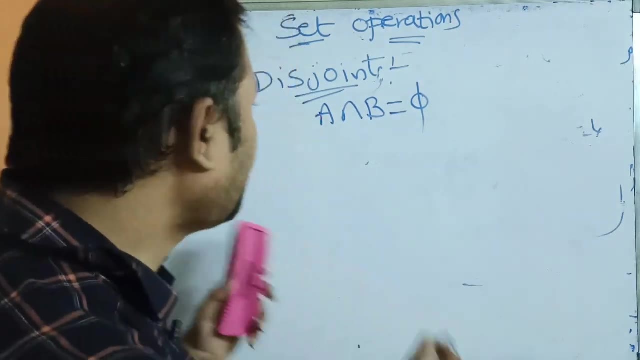 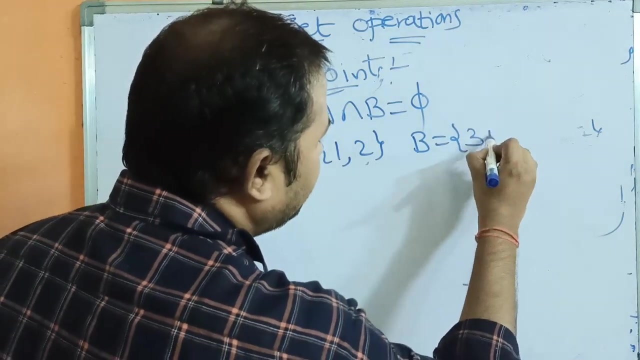 if A intersection B is equal to pi. If the sets A and B doesn't have any common element, then we can say that those two are disjoint sets. Let we have two sets such as: A is equal to 1, 2.. B is equal to 3, 4.. Here: 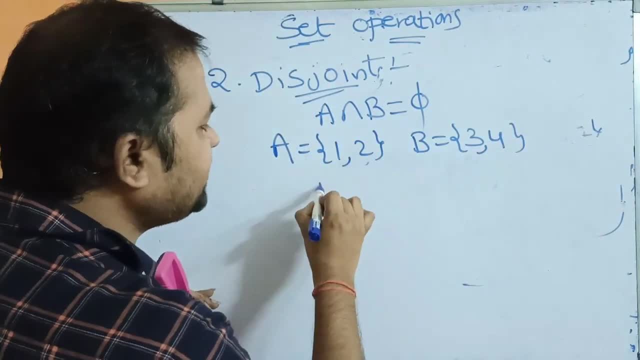 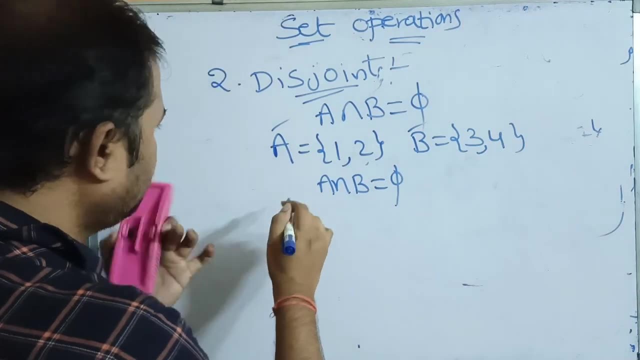 in A and B we don't have any common element. So we can say that A and B is equal to pi. So we can say that these two A and B are disjoint sets. Now let us see about the third operation, That is, union operation. 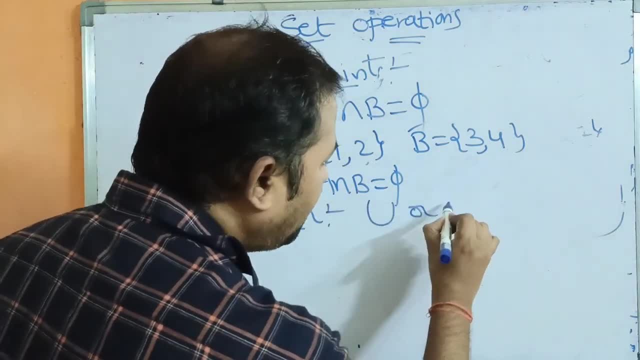 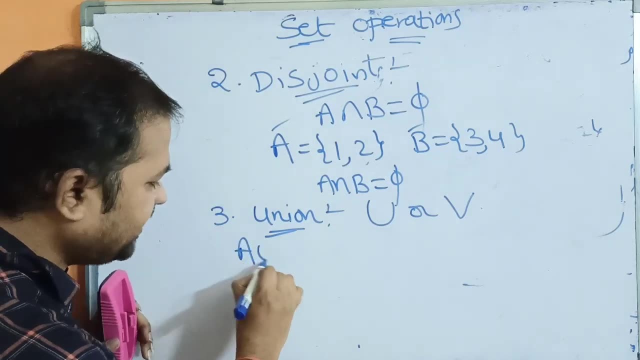 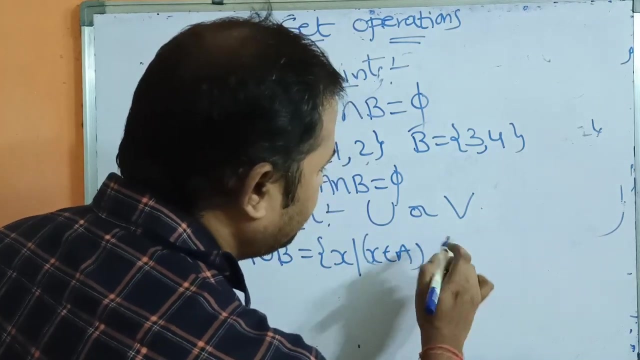 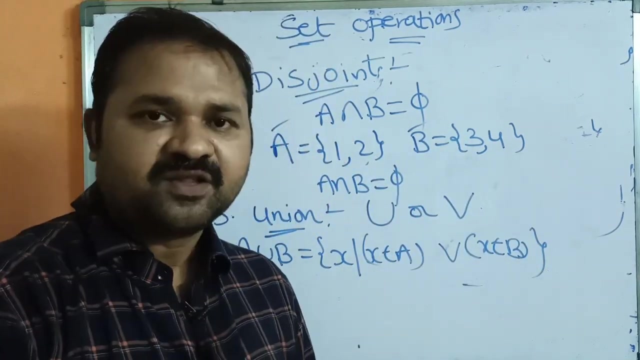 So union means we use a U symbol, or we can use this V also, So this is denoted with the help of this symbol. A union. B is equal to X, such that X belongs to A, or R symbol, So X belongs to B. So union means it contains the elements of A or the elements of B. That 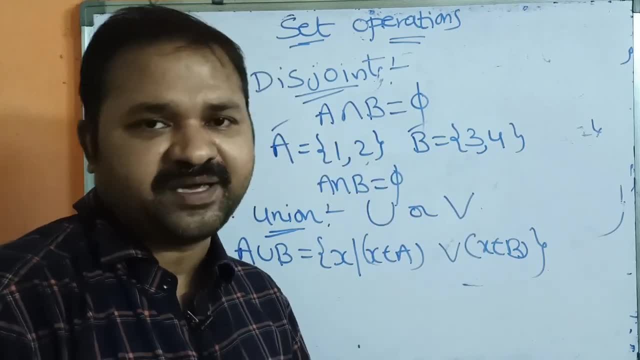 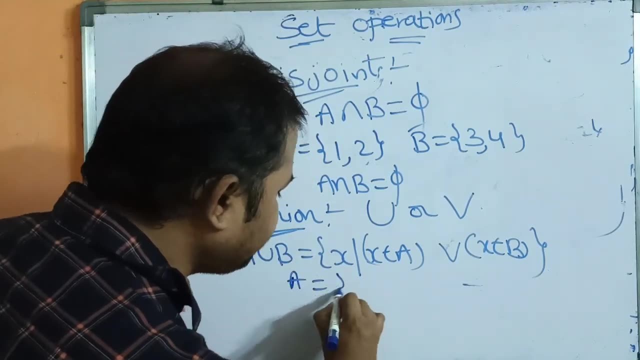 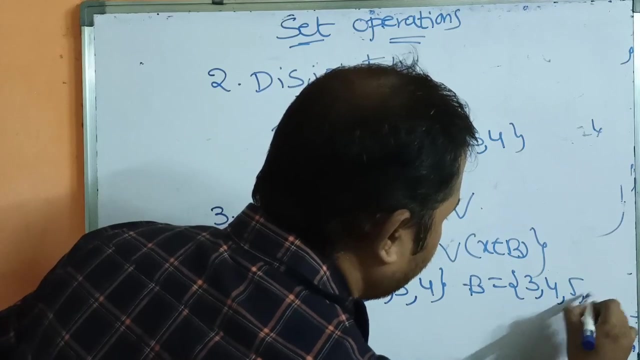 means it contains the elements of A as well as the elements of the B. If duplicate elements are there, then we have to write only once. Let we have two sets such as A is equal to 1,, 2,, 3,, 4.. B is equal to 3,, 4,, 5,, 6.. So then, what is A union B? A union B means what We 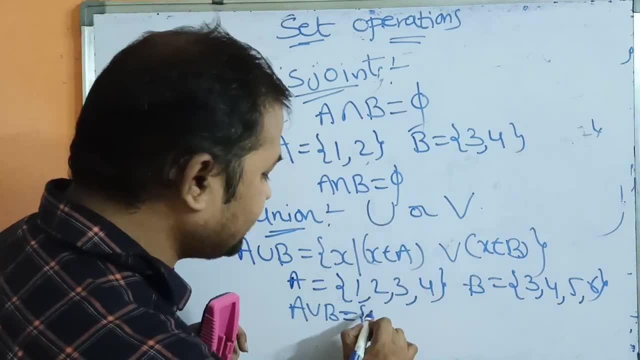 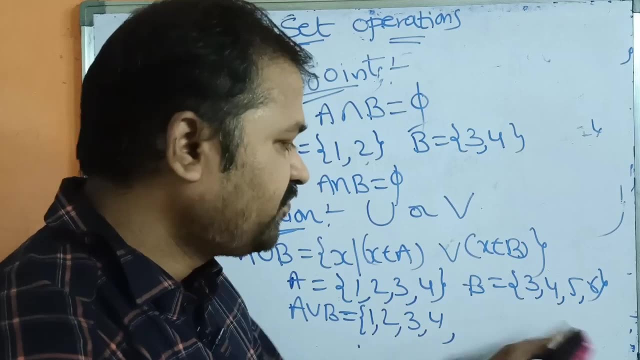 have to write both the set elements. So what are set A elements 1,, 2,, 3, 4? What are B elements 3,, 4,, 5, 6?? But 3, 4 is already present in A, So we have to write the remaining elements. 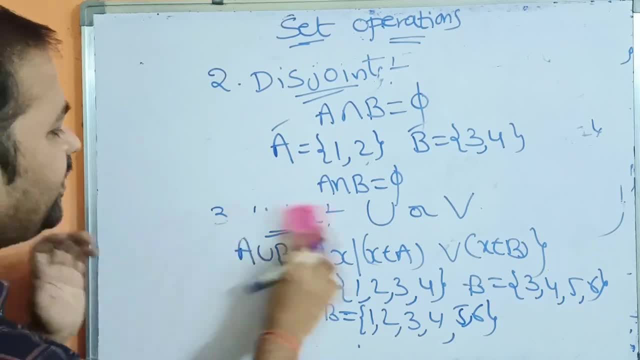 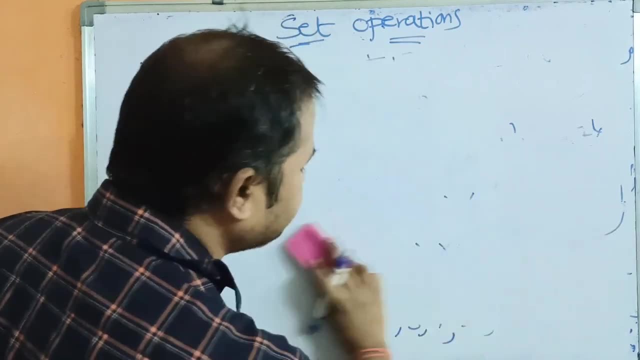 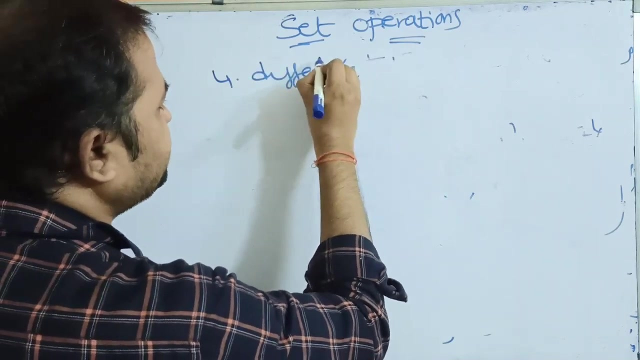 So 5,, 6.. So this is about disjoint and union operation. So three operations are over. Now let us see the remaining four operations. The next operation is difference operation. So the next operation is difference operation, So difference. If we have two sets, such as 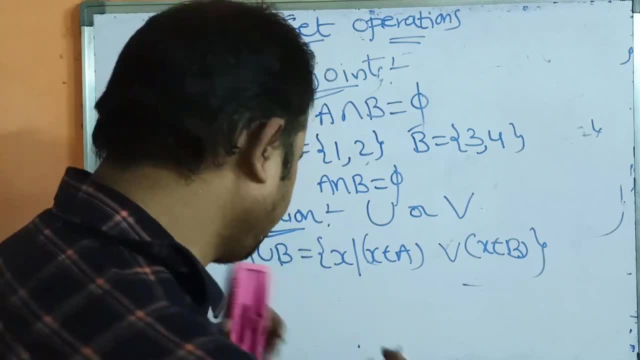 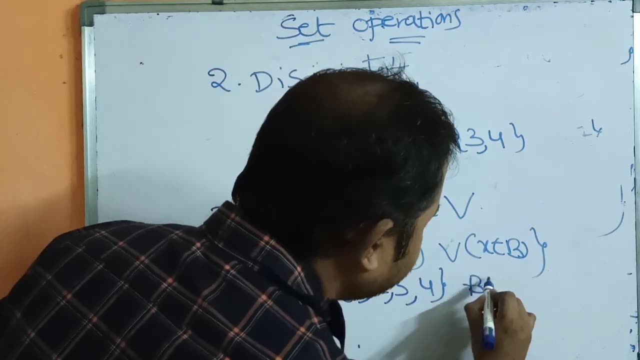 If duplicate elements are there, then we have to write only once. Okay, Let we have two sets, such as: A is equal to 1,, 2,, 3, 4.. B is equal to 3,, 4,, 5.. 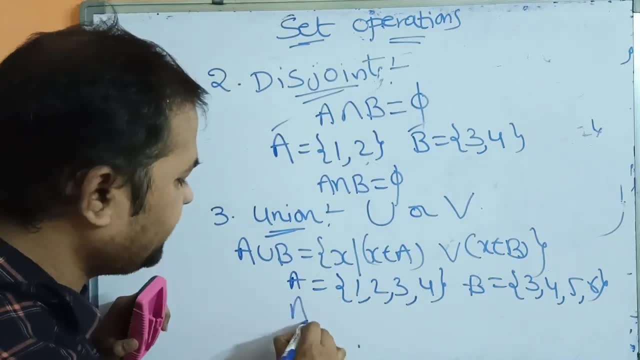 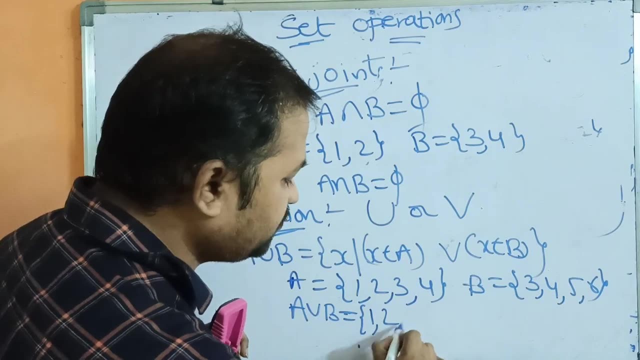 Okay, So then, what is A union B? A union B means what we have to write, both the set elements. So what are set A elements 1,, 2,, 3,, 4, comma? what are B elements 3,, 4,, 5,, 6.. 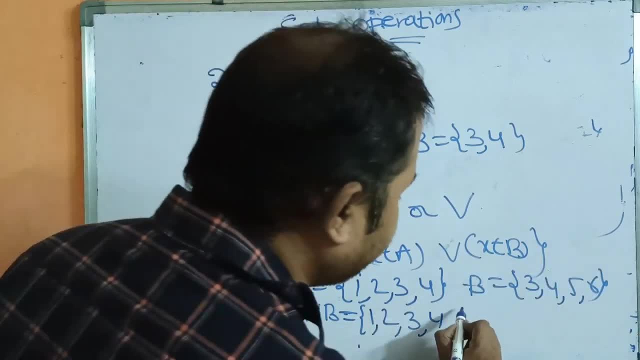 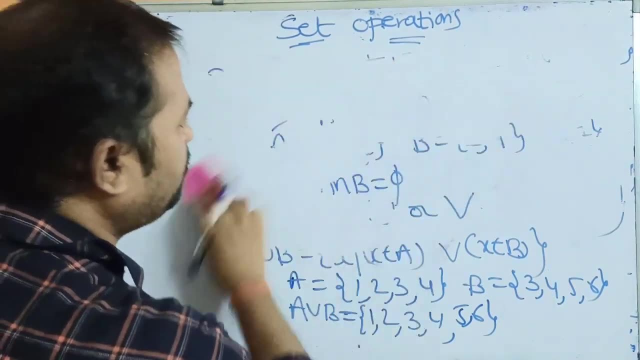 But 3, 4 is already present in A, So we have to write the remaining elements, So 5, 6.. Okay, So this is about disjoint and union operation. So three operations are over. Now let us see the remaining four operations. 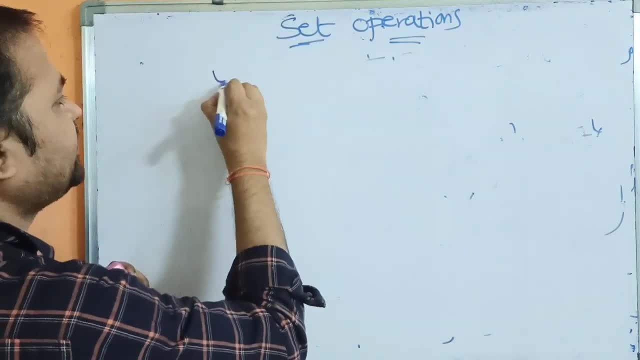 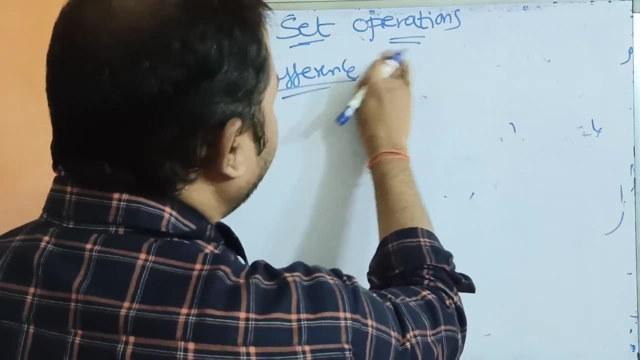 The next operation is difference operation. So the next operation is difference operation, So difference. If we have two sets, such as A and B, then the difference is denoted by minus symbol. So we can denote with the help of minus symbol. 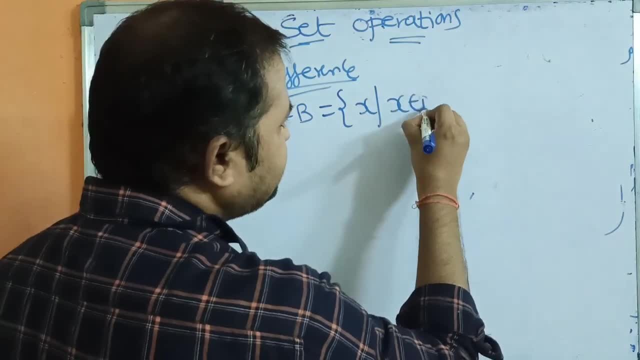 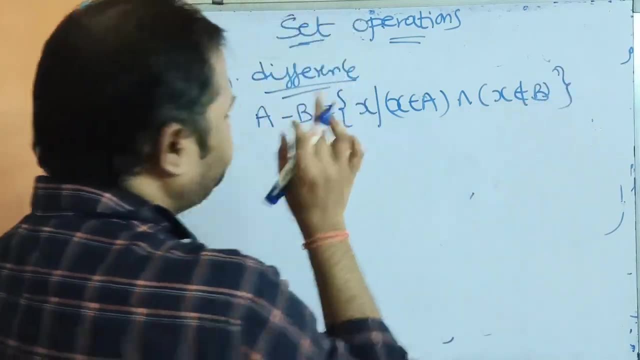 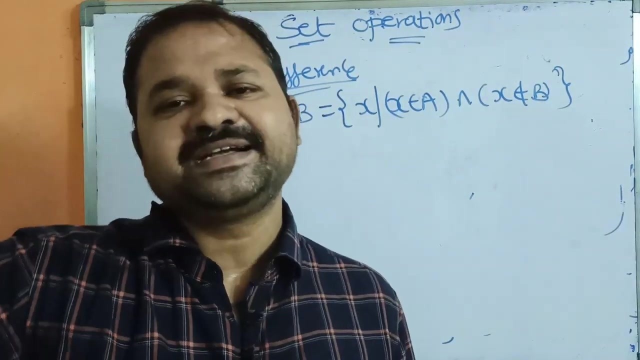 A minus B is equal to. Here the formula is like this: X is such that X belongs to A, and X does not belong to A. So here union means Here the set contains all the elements Of A, But those elements should not be present in B. 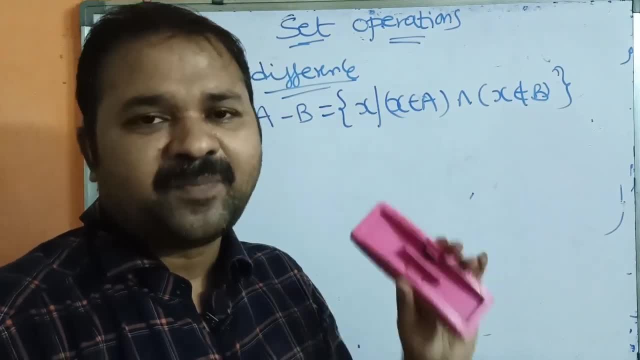 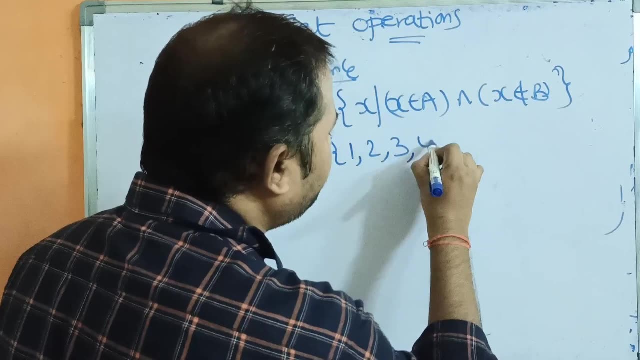 Okay, It contains all the elements of A, But they are not present in B. Let us take an example for this. Let A is equal to 1,, 2,, 3,, 4, 5.. B is equal to. 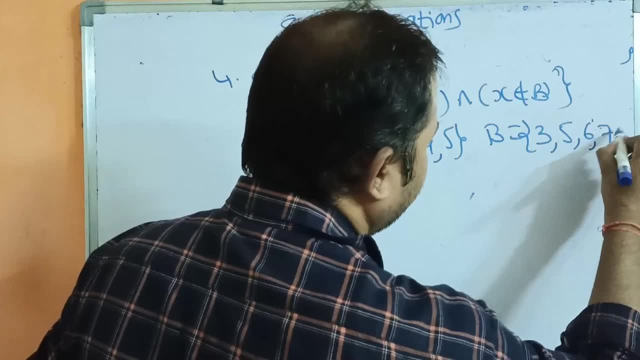 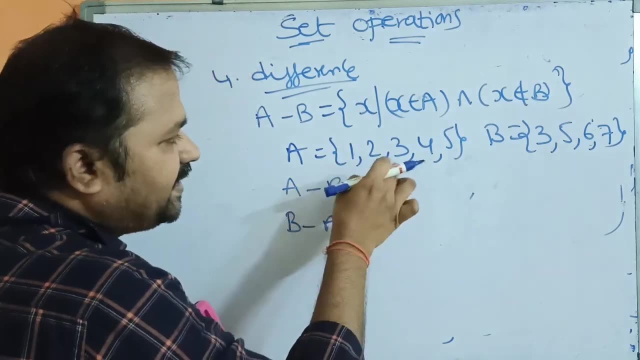 B is equal to 3,, 5,, 6,, 7.. Okay, Now let us calculate A minus B, B minus A. So what is A minus B? A means 1,, 2,, 3,, 4,, 5.. 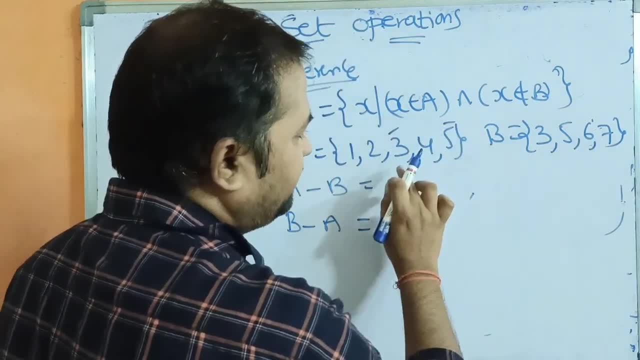 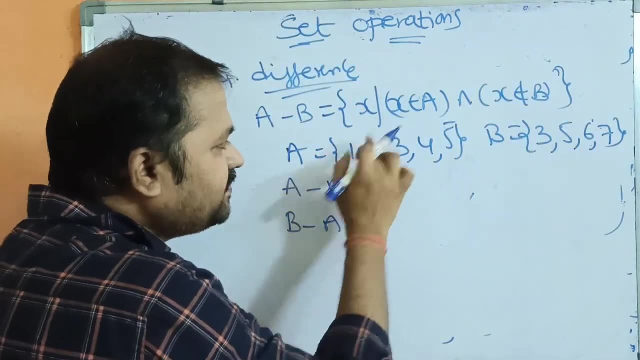 B means 3,, 5,, 6, 7.. So we can cancel 3, 5.. So we can cancel 3, 5.. Why? Because here 3, 5 are present in B, So we have to take the remaining elements of A. 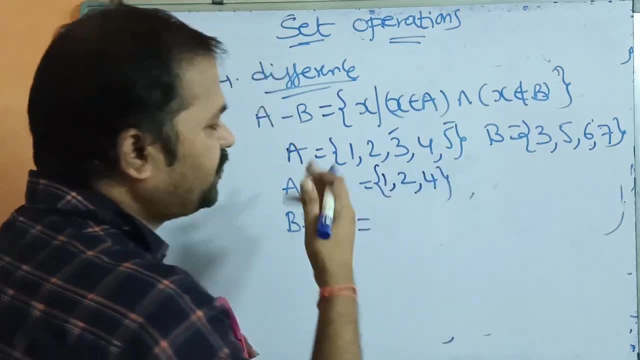 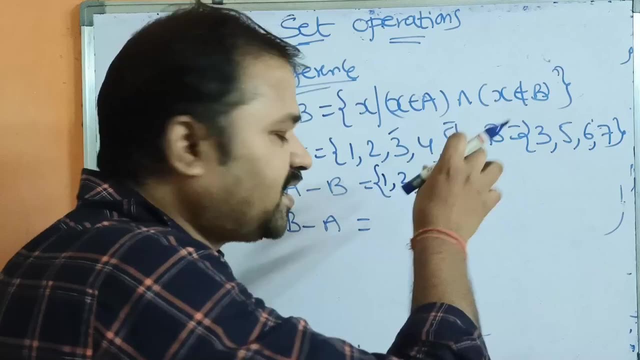 So the remaining elements of A are what? 1,, 2, 4.. Okay, So what is minus operation? It contains all the elements of A And those elements, But they are not present in B, But here, if you consider here: 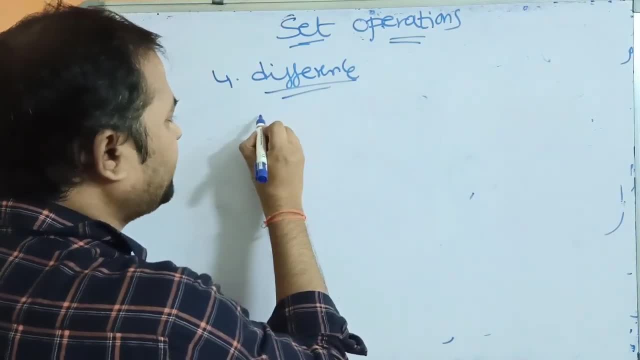 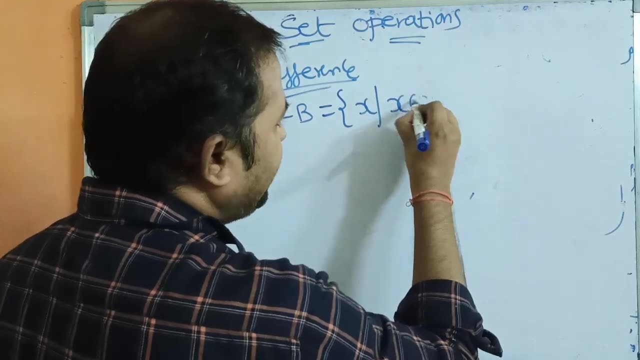 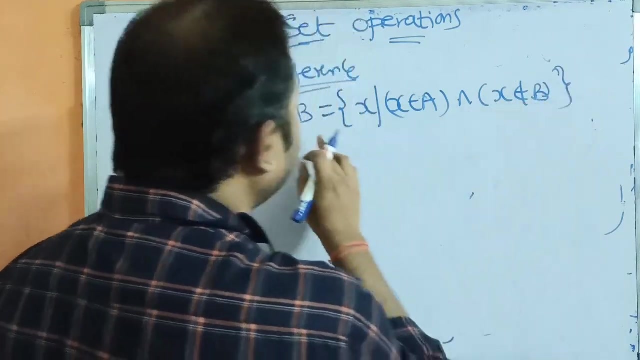 A and B, then the difference is denoted by minus symbol. So we can denote with the help of minus symbol: A minus B is equal to. yet the formula is like this: X is such that X belongs to A, and X does not belong to A. So here union means, yet the set. 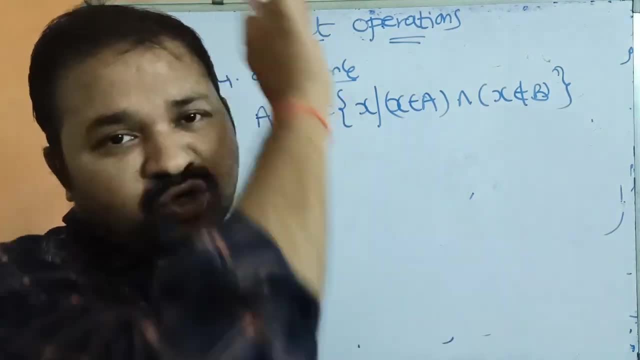 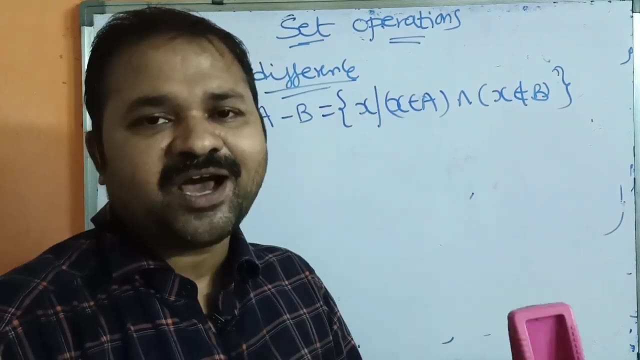 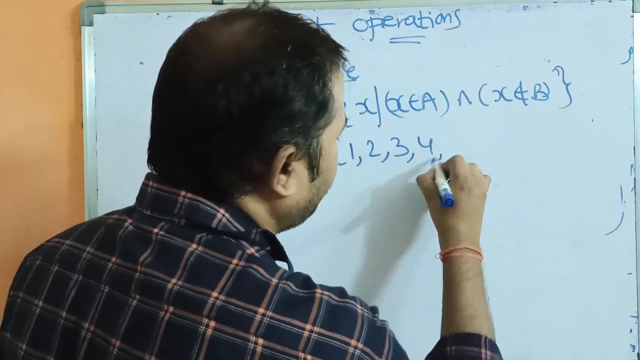 contains all the elements of A, but those elements should not be present in B. It contains all the elements of A, but they are not present in B. Let us take an example for this. Let A is equal to 1,, 2,, 3,, 4, 5.. B is equal to. 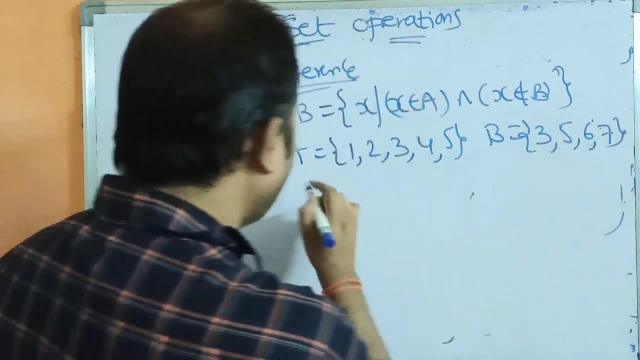 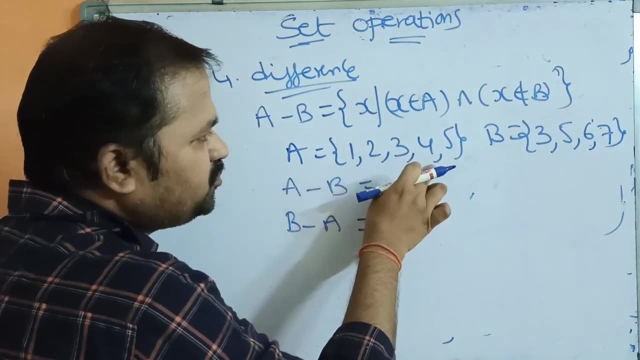 3,, 5,, 6, 7.. Now let us calculate A minus B, B minus A. So what is A minus B? A means 1,, 2,, 3,, 4, 5.. B means 3,, 5,, 6,, 7.. So we can cancel 3, 5.. So we can cancel 3, 5.. Why? 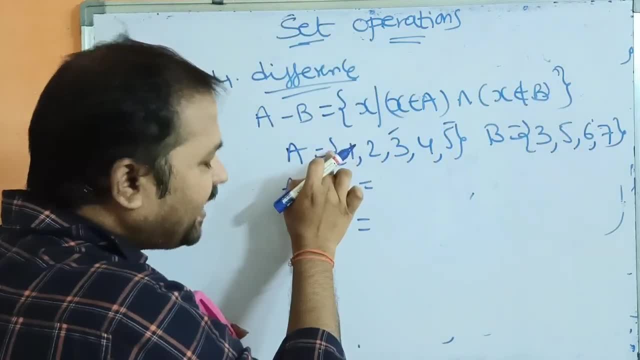 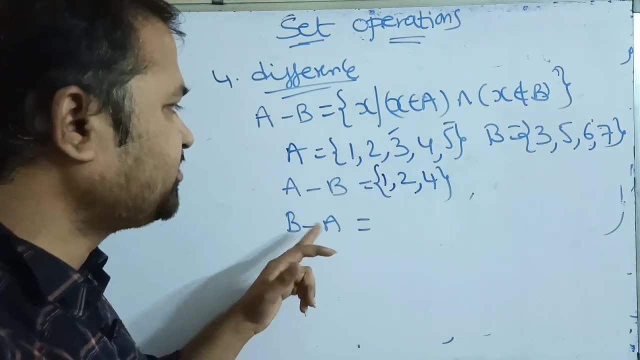 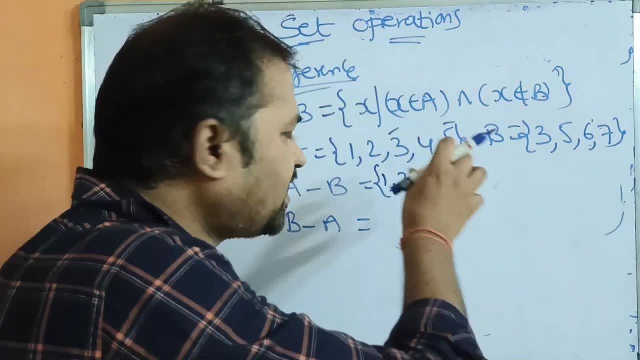 is minus operation? It contains all the elements of A. So what is minus operation? It contains all the elements of A. So what is minus operation? It contains all the elements of A And those elements. but they are not present in B. But here, if you consider here, 3, 5 are present in B. So 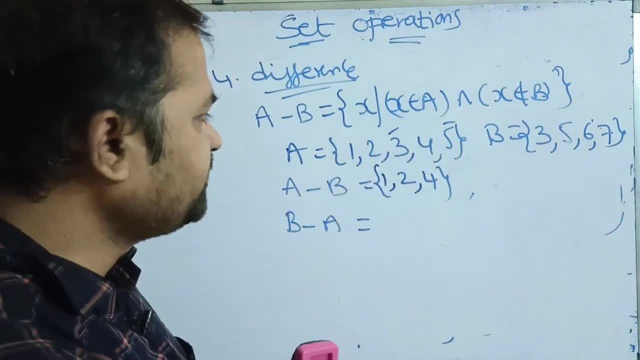 we should not consider them. So the remaining elements are 1,, 2, 4.. Or simply, let us do the subtraction So we can cancel 3, 5.. So the remaining elements are 1,, 2, 4.. Now what is B? 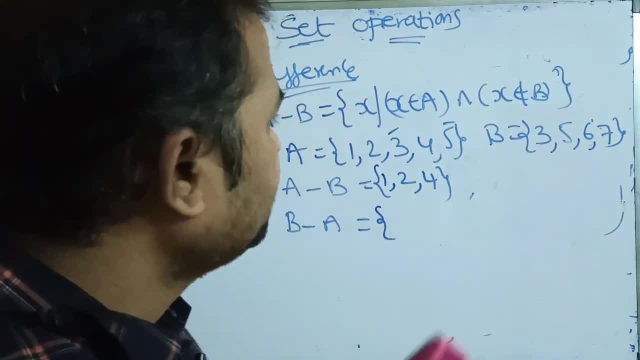 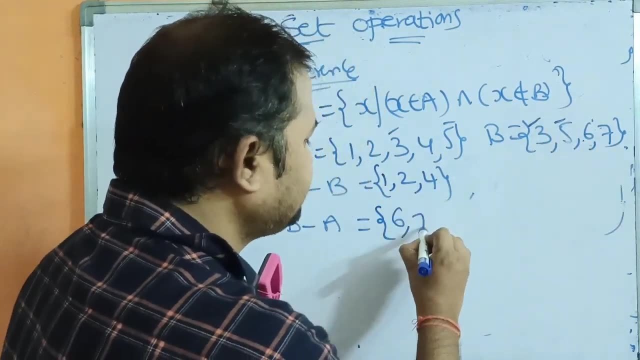 minus A. What is B minus A? Let us calculate this. So 3, 5,, 6, 7 means we can cancel 3, 5.. we can cancel 3, 5. so the remaining elements of b are what? 6, 7. okay, the remaining elements of b are. 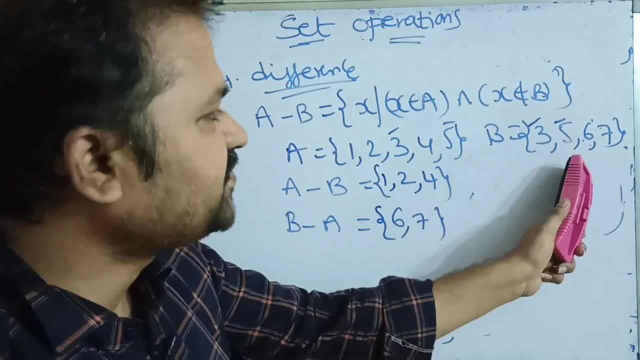 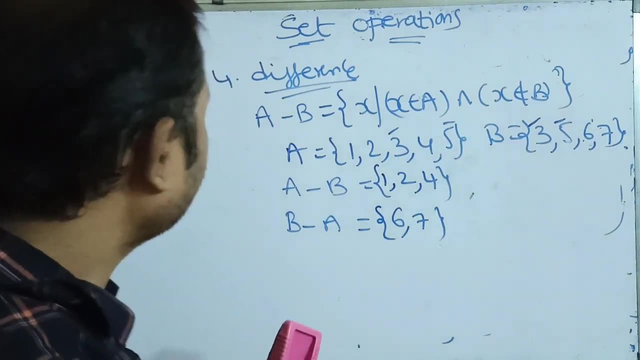 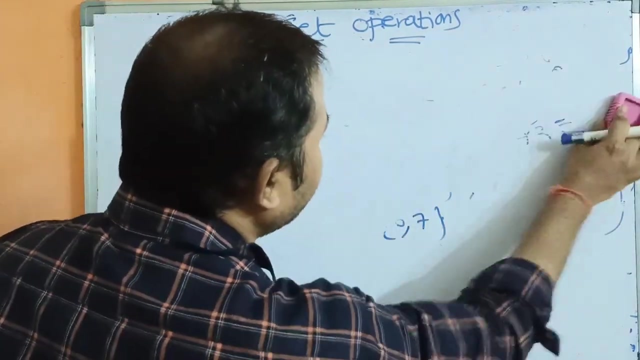 so b minus a means it consists of all the elements of b, but they are not present in a. but here 3, 5 are present in a, so we need to write the remaining one. so this is about difference. now let us now let us see the next operation. the next operation is: difference is fourth operation, so the next. 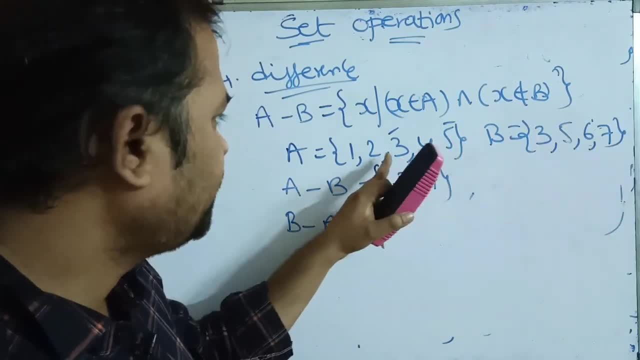 3, 5 are present in B, So we should not consider them. So the remaining elements are 1,, 2, 4.. Or simply, let us do the subtraction So we can cancel 3, 5.. 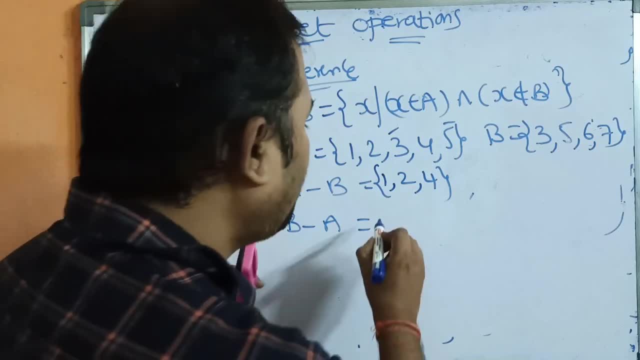 So the remaining elements are 1,, 2, 4.. Now, what is B minus A? What is B minus A? Let us calculate this. So 3, 5, 6, 7 means we can cancel 3, 5.. 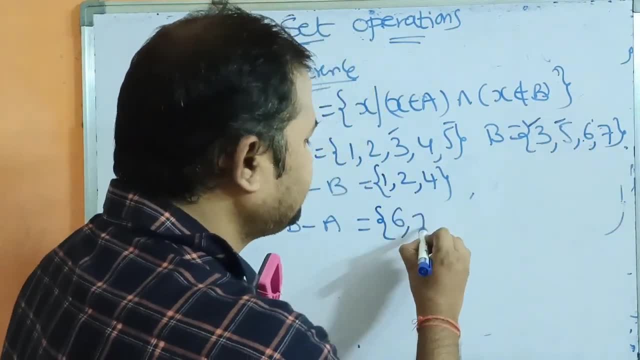 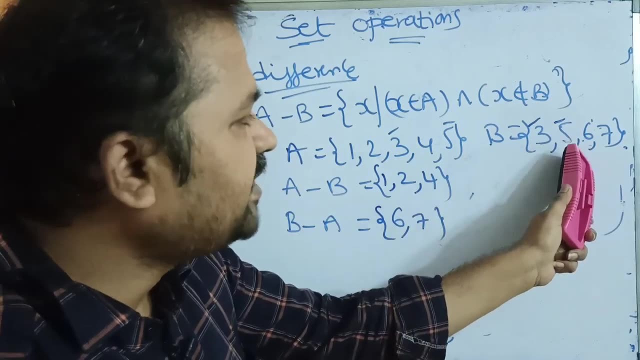 We can cancel 3, 5.. So the remaining elements of B are what? 6, 7.. Okay, The remaining elements of B are So: B minus A means it consists of all the elements of B, But they are not present in A. 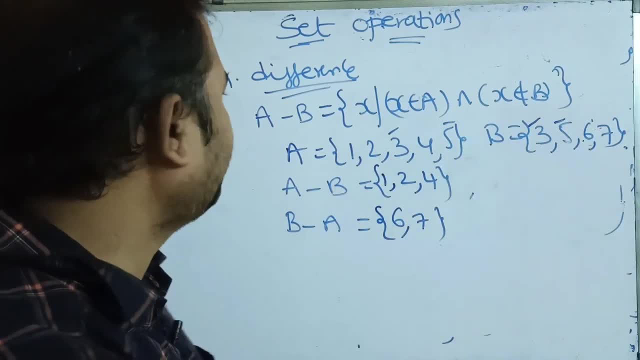 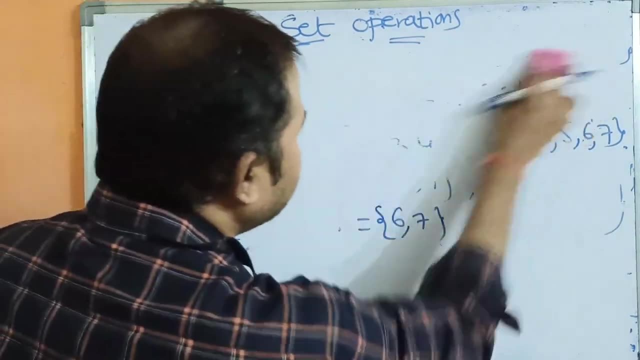 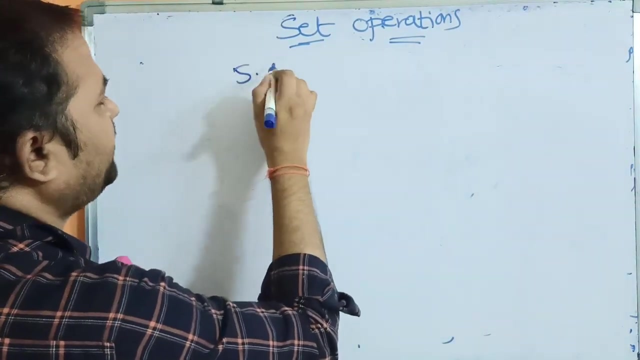 But here 3,, 5 are present in A, Okay, So we need to write the remaining one. So this is about difference. Now let us see the next operation. The next operation is: difference is fourth operation. So the next operation is complement operation. 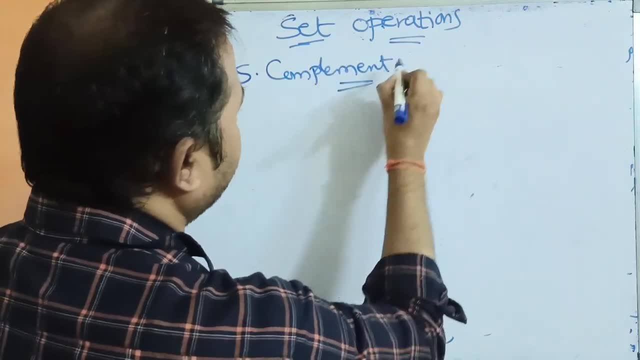 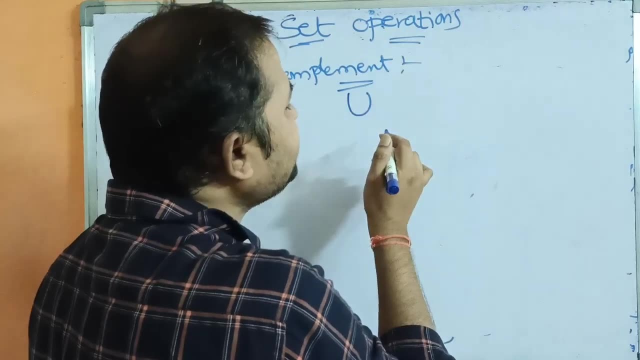 Complement operation. So what is complement operation Here? in order to perform the complement, We must need two sets. The first set is U- U means universal set- And the second set is A set. It may be A or B or any set. 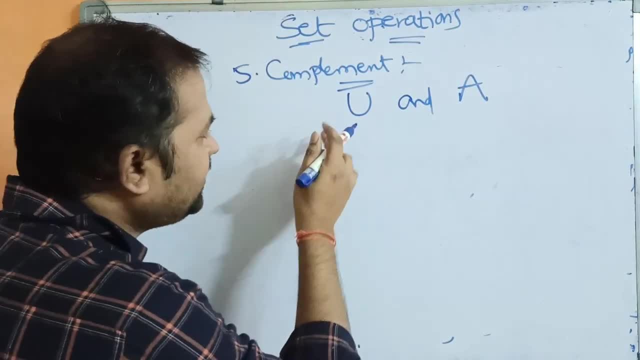 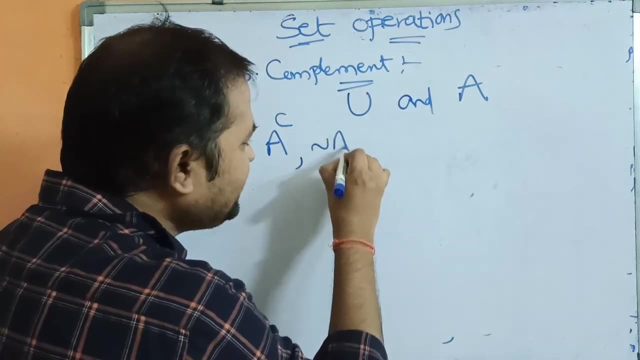 Then we can calculate the complement. Here, in order to denote the complement, We can use either A power C A complement, or we can use tilde A symbol, Or we can use A bar symbol. So a complement is denoted with the help of these three symbols. 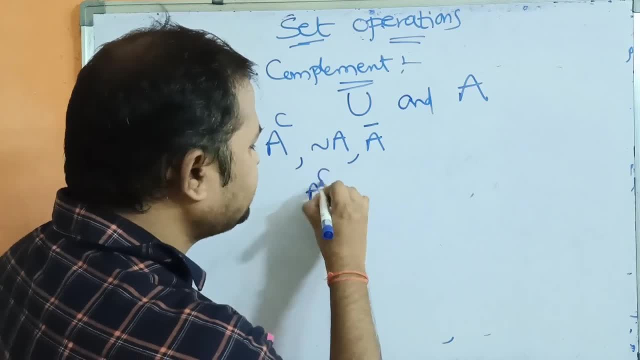 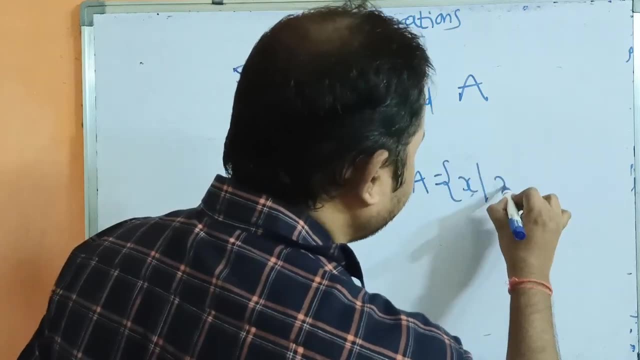 And we can write as any symbol: Okay, A power C is equal to. Here the formula is very simple: U minus A. U minus A is equal to X, is such that X belongs to U And X doesn't belongs to A. 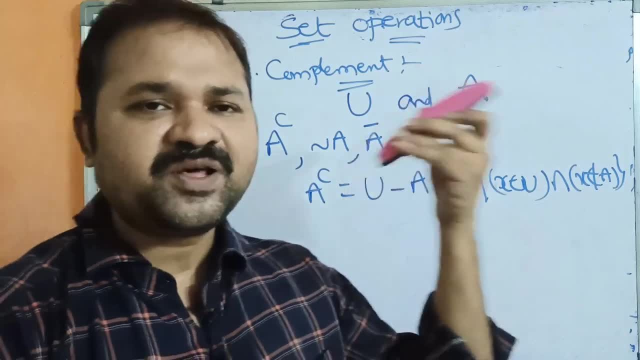 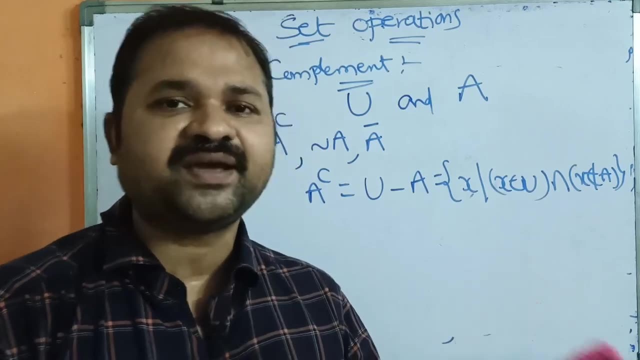 Okay, So how to calculate U minus A? It is similar to A minus B, only Already we discussed about A minus B. What is A minus B? It contains all the elements of A, But they are not present in B. Okay, 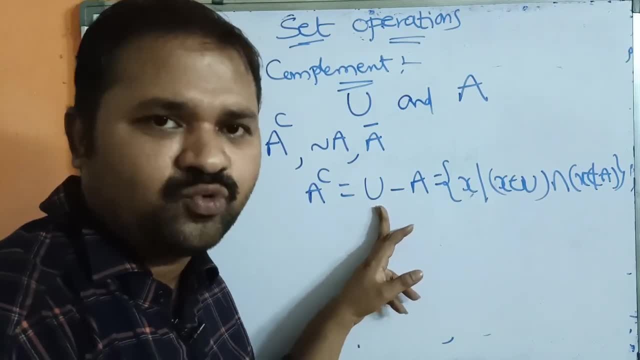 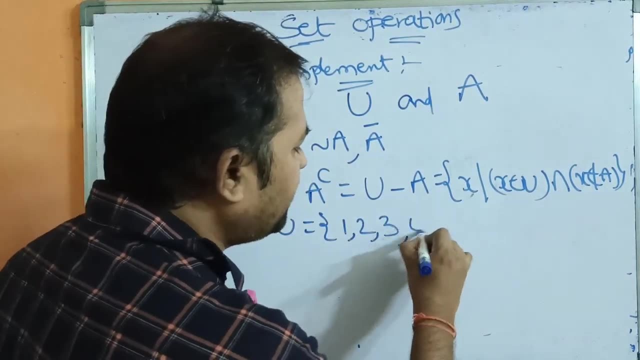 So what is U minus A? It contains all the elements of U, But they are not present in A. Okay, Let us take an example for this. A is U is equal to 1 comma, 2 comma, 3 comma. 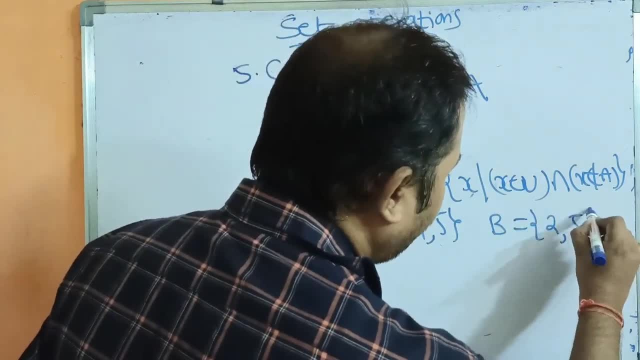 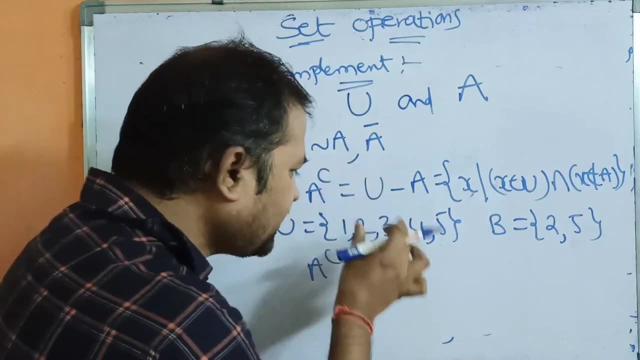 4 comma 5.. So B is equal to 2 comma 5.. Okay Now, A complement is equal to A complement Complement is equal to: So it contains all the elements of A, But they are not present in B. 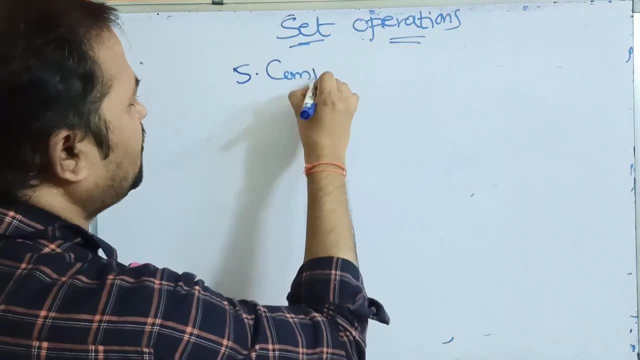 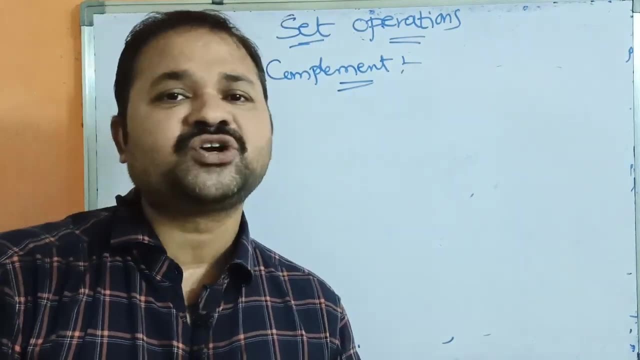 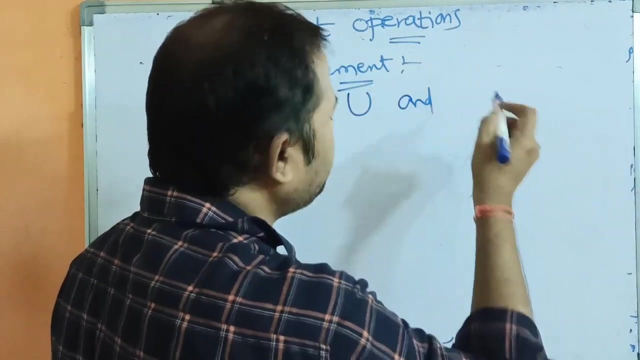 operation is complement operation, complement operation. so what is complement operation here? in order to perform the complement, we must need two sets. the first set is u- u means universal set- and the second set is a set- it may be a or b or any set. then we can calculate the complement. 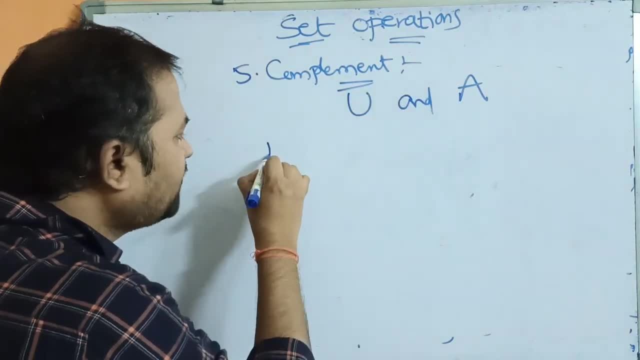 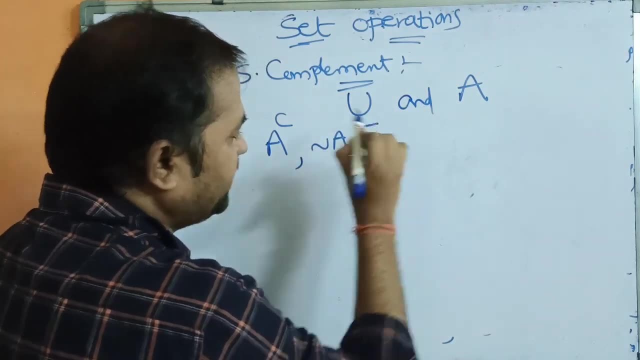 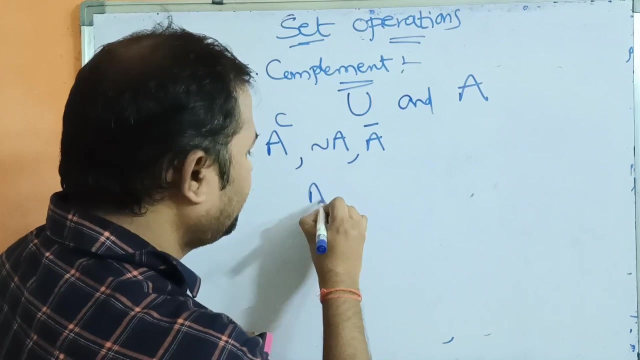 here, in order to denote the complement, we can use either a power c a complement, or we can use tilde, a symbol, or we can use a bar symbol. so a complement is denoted with the help of these three symbols and and we can write as any symbol: okay, a power c is equal to. here the formula is: 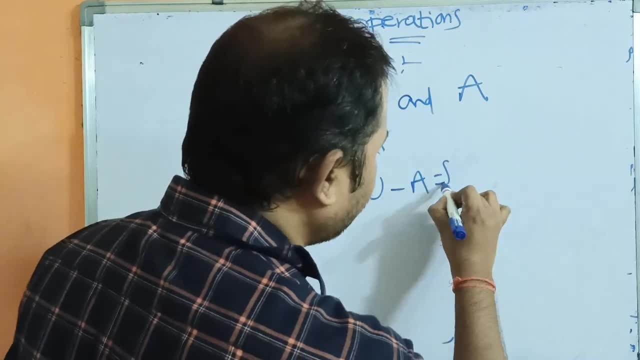 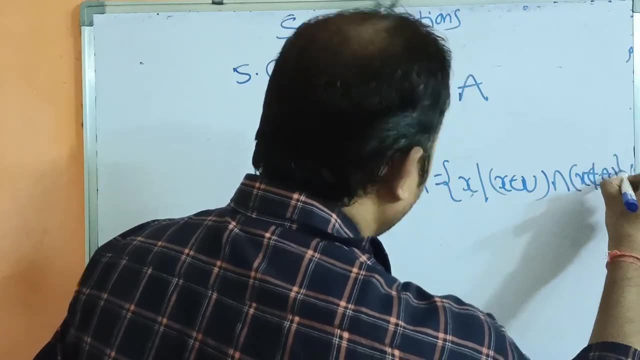 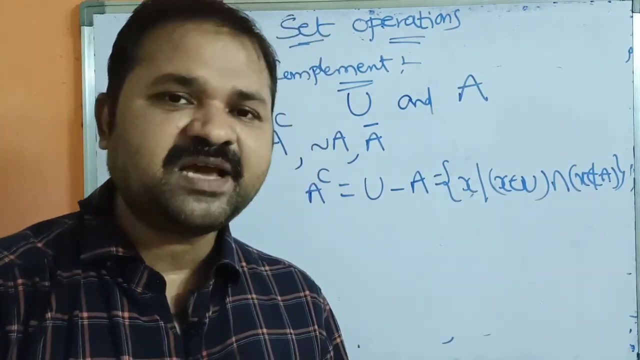 very simple: u minus a. u minus a is equal to x, such that x belongs to u and x doesn't belongs to a. okay, so how to calculate u minus a? it is similar to a minus b, only already we discussed about a. what is a minus b? it contains all the elements of a, but they are not present in b. okay, so what is u? 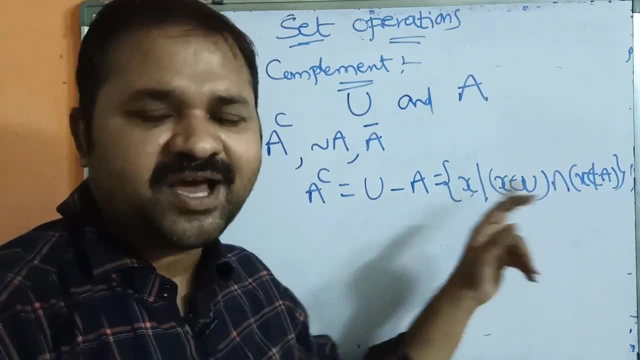 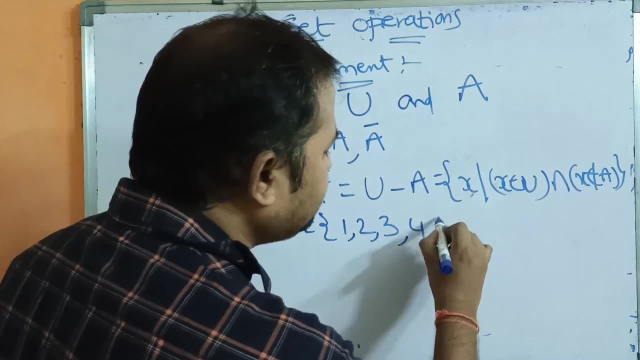 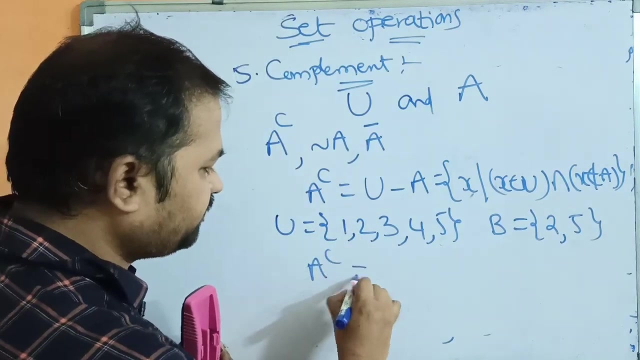 minus a, it contains all the elements of u, but they are not present in a. okay, let us take an example for this. a is u, v is equal to one comma, two comma three comma, four comma five, so b is equal to two comma five. okay now, a complement is equal to a complement. complement is equal to, so it contains: 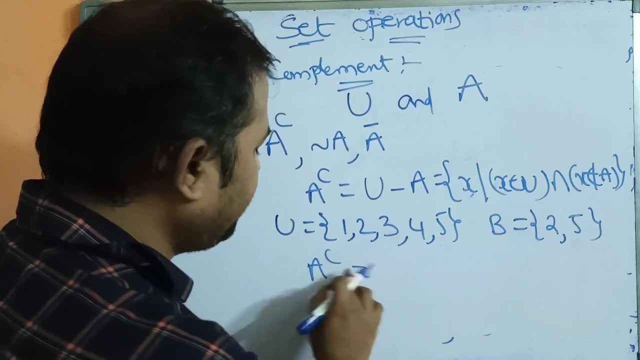 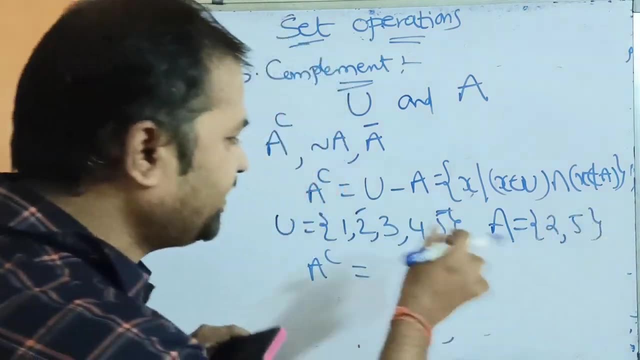 all the elements of a, but they are not present in b. but they are not here. we have taken what- let us assume this as b, or we can take b power complement. okay, here two and five are present in a, so we should not consider them. why? because these two elements are present in a, so the 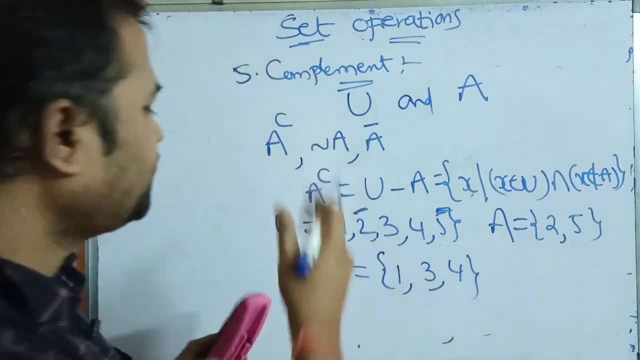 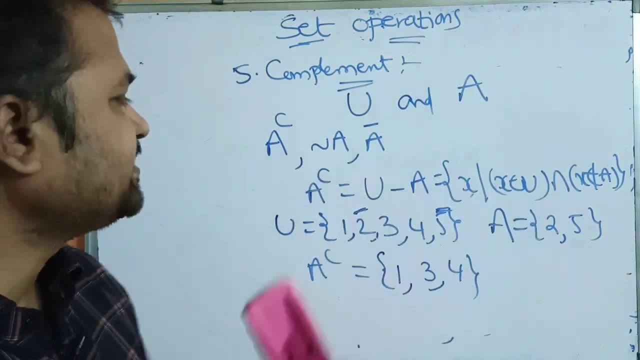 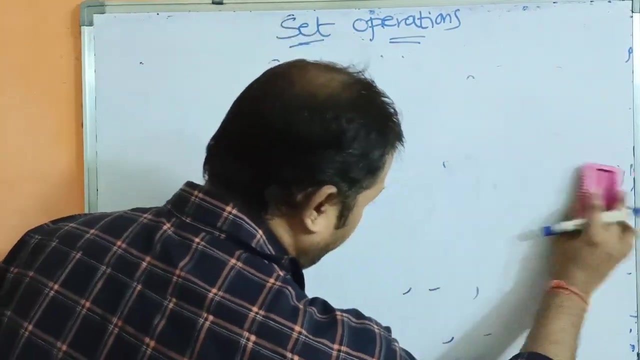 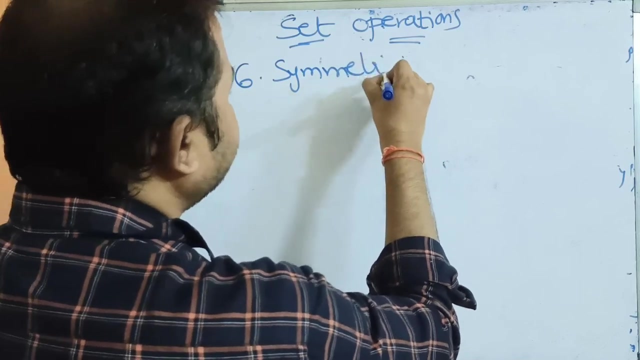 remaining elements are one, three, four. so one three, four. so this is nothing but complement. okay, complement means we must need universal set and another set. the formula is u minus a. the last two operations, symmetric difference, as well as cartesian product. let us see about symmetric difference. let us see about symmetric difference. so what is symmetric difference? 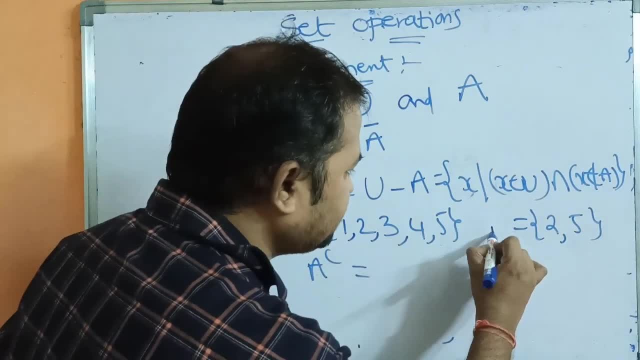 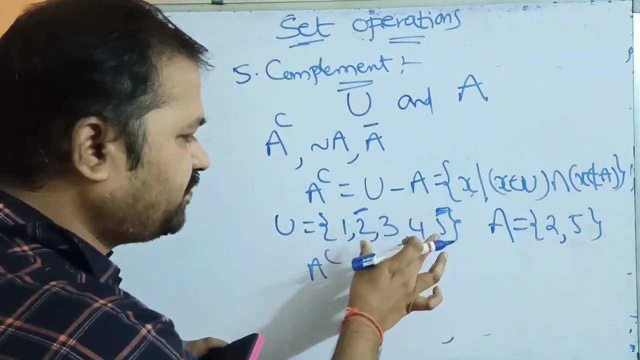 But they are not Here. we have taken what? Let us assume this as B, Or we can take B power complement. Okay, Here 2 and 5 are present in A, So we should not consider them. Why? Because these two elements are present in A. 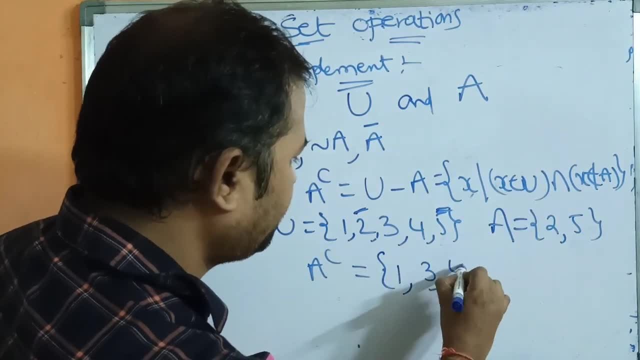 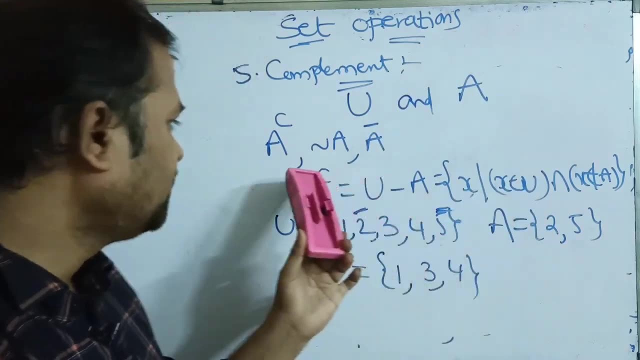 So the remaining elements Are 1, 3, 4.. So 1, 3, 4.. So this is nothing but complement. Okay, Complement means we must need universal set And another set. The formula is U minus A. 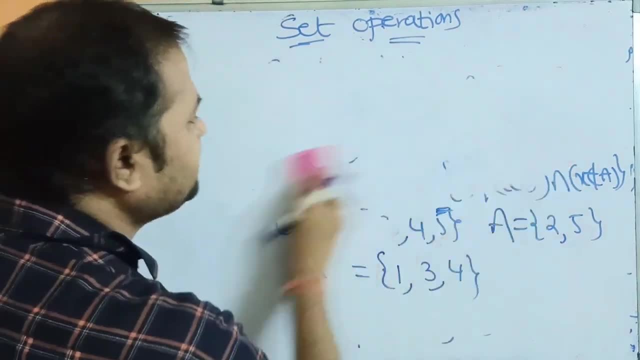 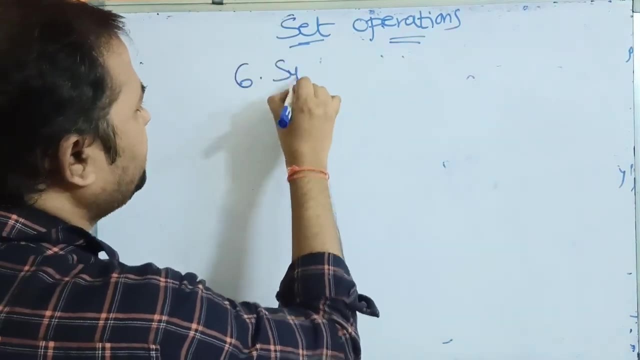 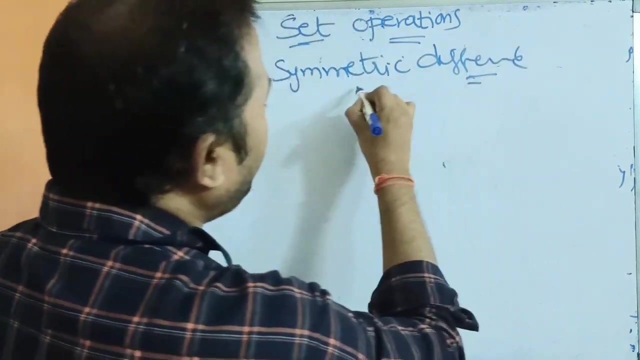 Now let us see the last two operations: Symmetric difference as well as Cartesian product. Let us see about symmetric difference. Let us see about symmetric difference. So what is symmetric difference Here If we have two sets Such as A and B? 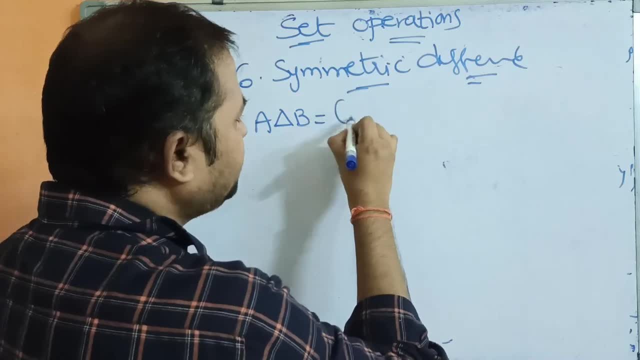 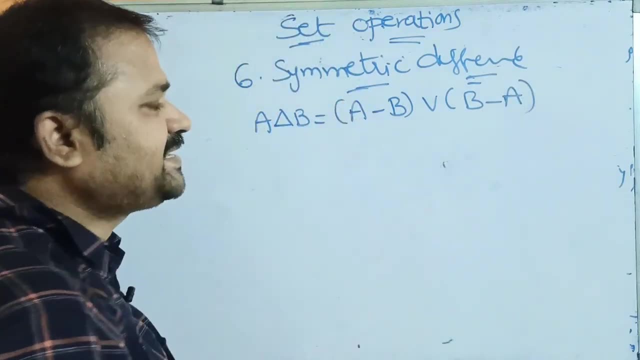 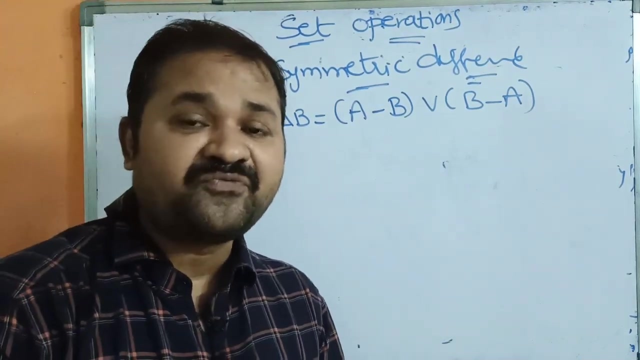 Then the symmetric difference is denoted by A delta B. Here the formula for A delta B is A minus B, union B minus A. So symmetric difference means It contains the elements of A or B, But not both the sets. It contains the elements of A or B. 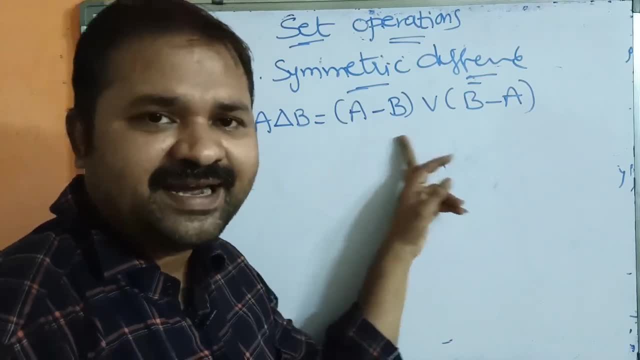 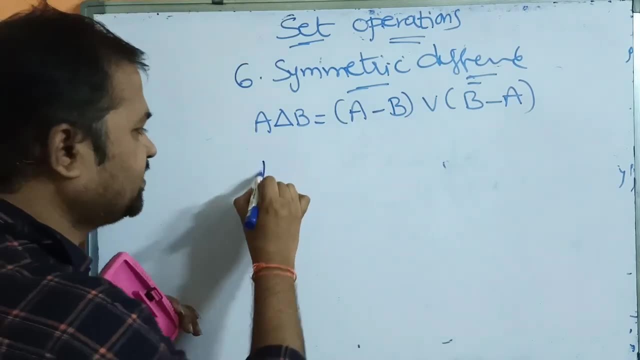 But not both the sets. So if we take A minus B, It contains the elements of A. Okay, If we take B minus A, It contains the elements of B, But not the both, But not both the sets. Let us take an example. 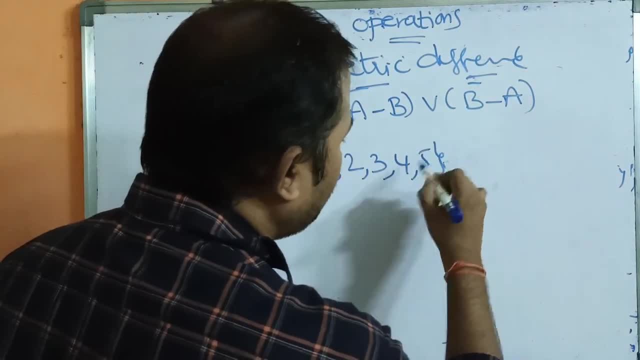 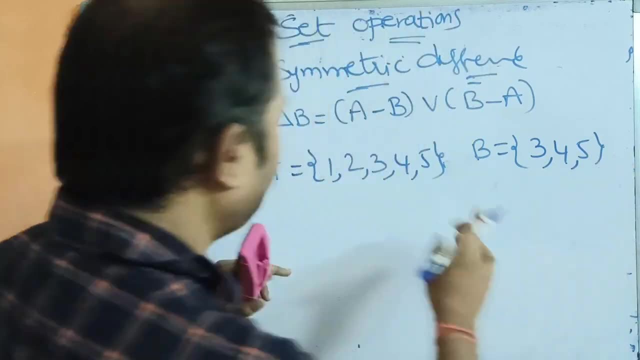 A is equal to 1 comma, 2 comma, 3 comma, 4 comma, 5.. So B is equal to, B is equal to. Let us take an example: So 3, 4, 5.. 3, 4, 5.. 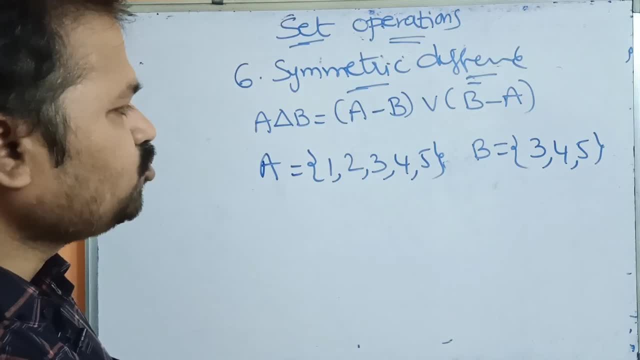 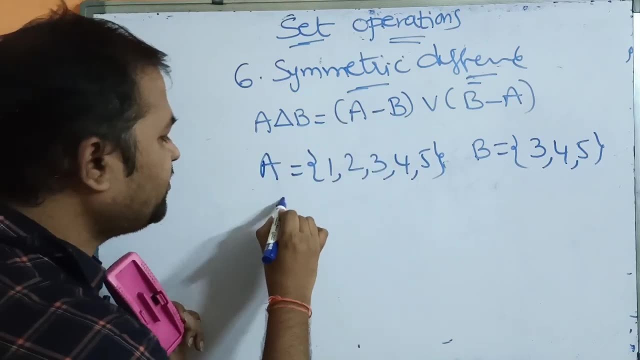 So what is the example here? A is equal to 1 comma 2 comma, 3 comma, 4 comma 5.. B is equal to 3 comma 4 comma 5.. So next, First we need to calculate A minus B. 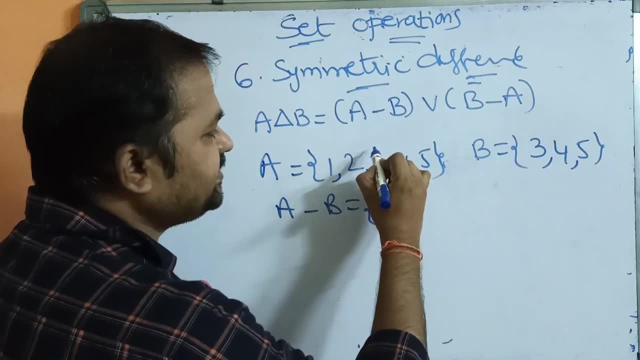 So what is A minus B? So 1, 2, 3, 4, 5. 3, 4 5 means These 3 elements are present in B, So we have to take the remaining 2 elements, 1 comma 2.. 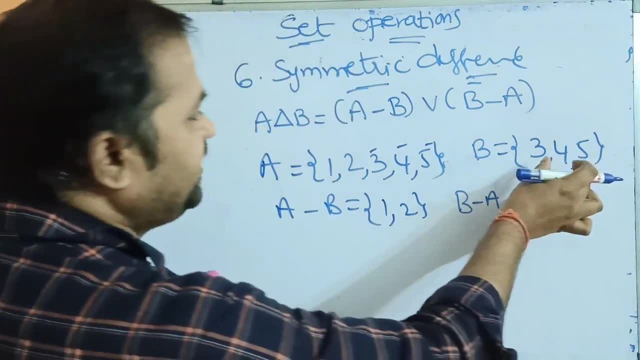 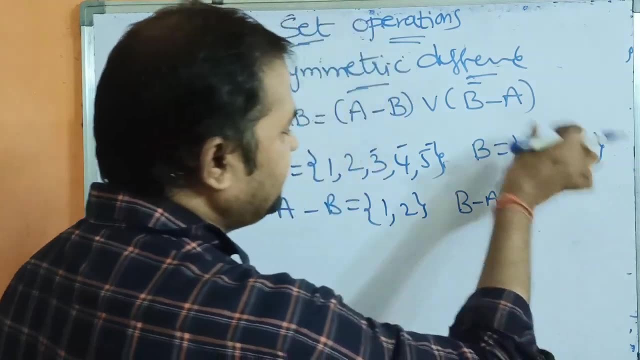 Now, what is B minus A? B minus A means Here 3, 4, 5 are present in A, So here no remaining elements are there? Okay, Here all these elements are present in A, So B minus A means pi. 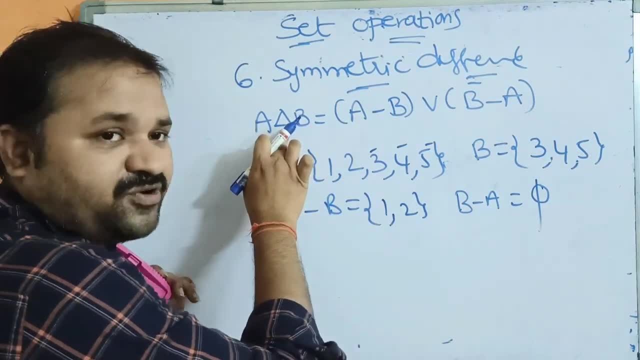 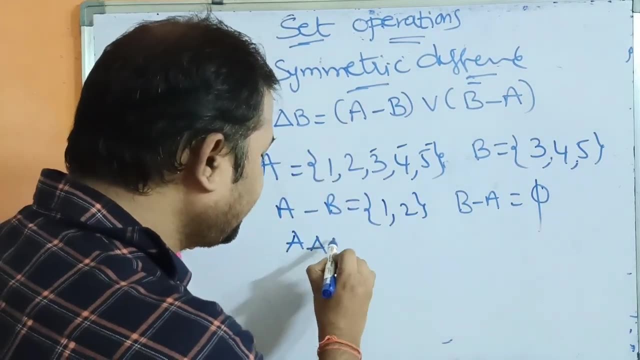 Okay, So what is So this symmetry difference is denoted by this triangle. This is pronounced as delta A, delta B. So what is A delta B? It contains the elements Of A or B, but not both. So what is A minus B? 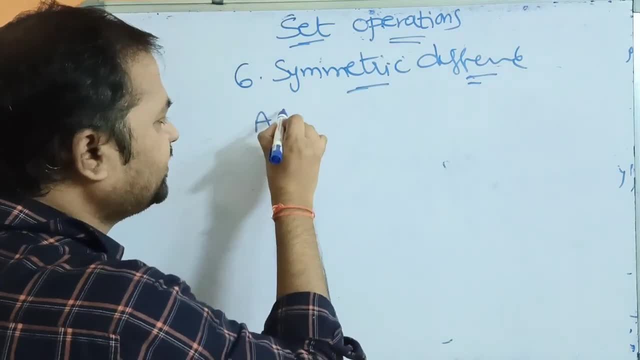 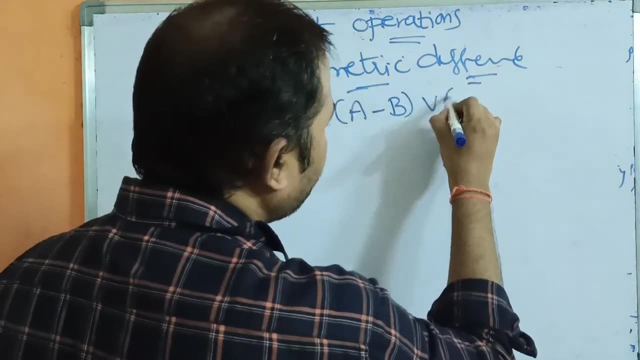 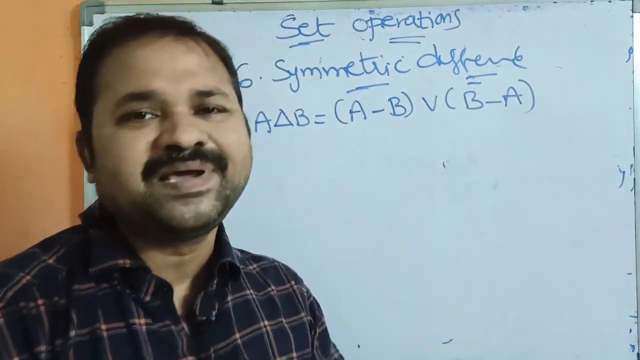 here, if we have two sets such as a and b, then the symmetric difference is denoted by a delta b. if the formula for a delta b is a minus b, union b minus a, so symmetric difference means it contains elements of a or b, but not both the sets. it contains the elements of a or b, but not both the. 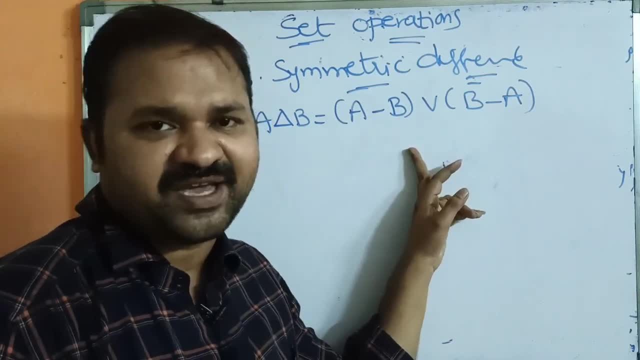 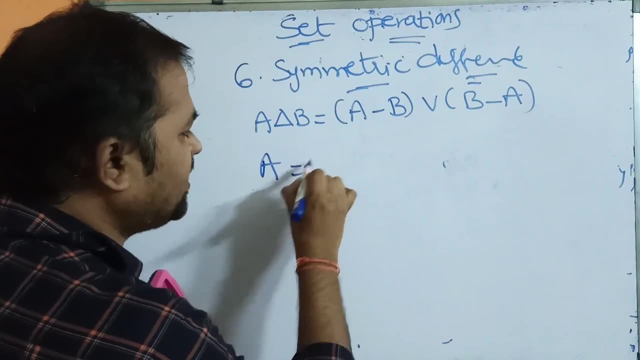 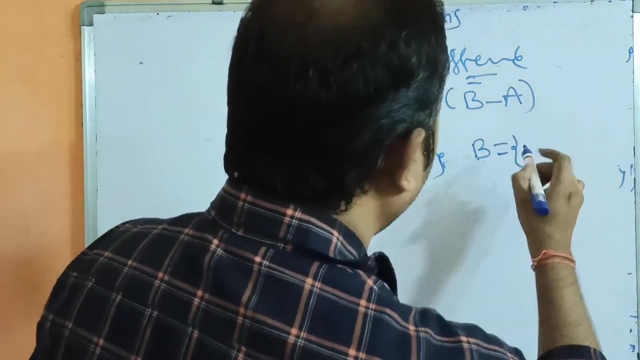 sets. so if you take a minus b, it contains the elements of a. okay, if you take b minus a, it contains the elements of b, but not the both, but not both the sets. let us take an example: a is equal to 1 comma, 2 comma, 3 comma, 4 comma 5.. so b is equal to, b is equal to. let us take an example so. 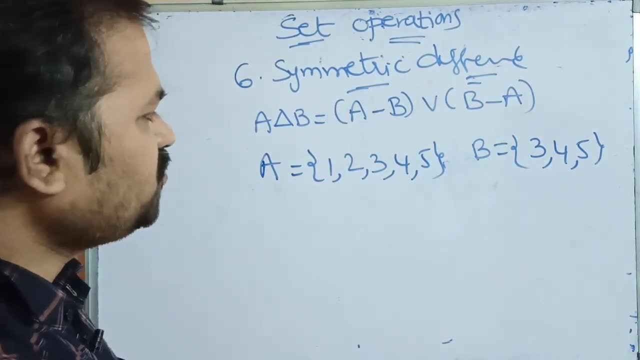 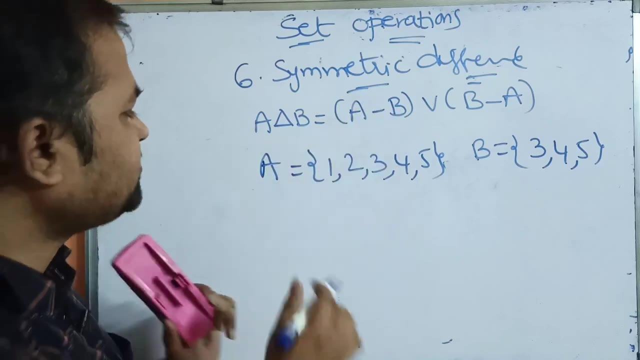 5.. So what is the example here? a is equal to 1 comma 2 comma, 3 comma, 4 comma 5, b is equal to 3 comma 4 comma 5.. So next, first we need to calculate a minus b. So what is a minus b? 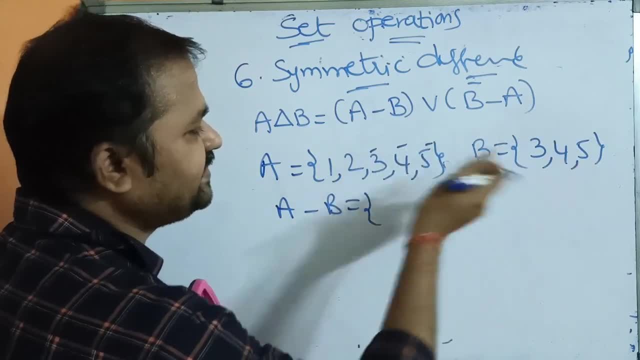 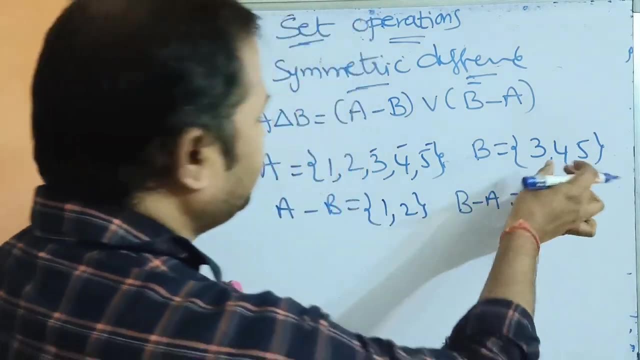 So 1,, 2,, 3, 4, 5, 3,, 4, 5 means these three elements are present in b, So we have to take the remaining two elements, 1 comma 2.. Now what is b minus a? b minus a means here 3,, 4, 5 are. 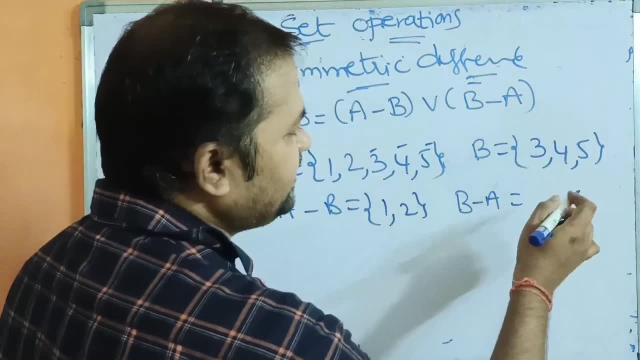 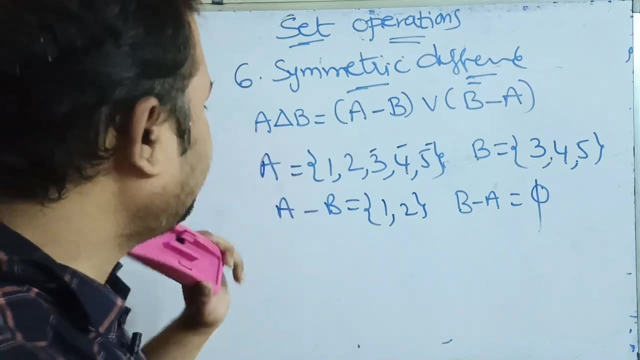 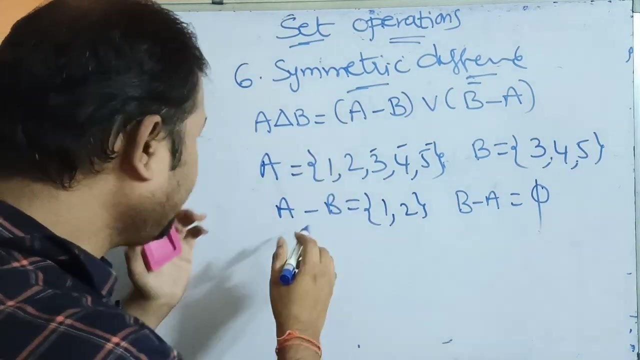 present in a, So here no remaining elements are there Here. all these elements are present in a, So b minus a means pi. So what is this symmetry difference is denoted by this triangle. This is pronounced as delta a, delta b. So what is a, delta b? It contains the elements of a or b, but 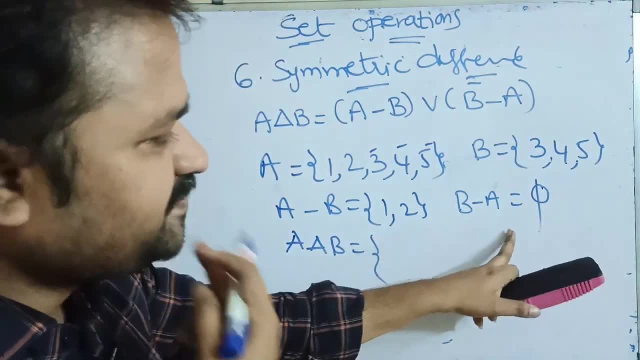 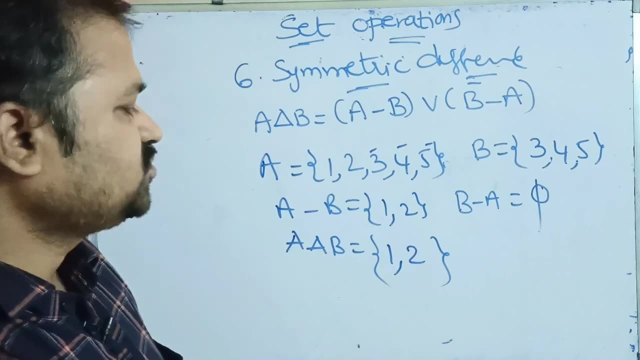 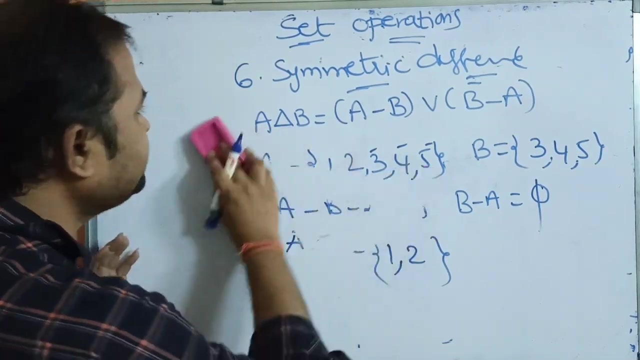 not both. So what is a minus b? 1 comma 2.. What is b minus a pi? So 1 comma 2. union pi means what 1 comma 2.. 1 comma 2.. So this is the. in this way we can calculate the symmetric difference. Now let us. 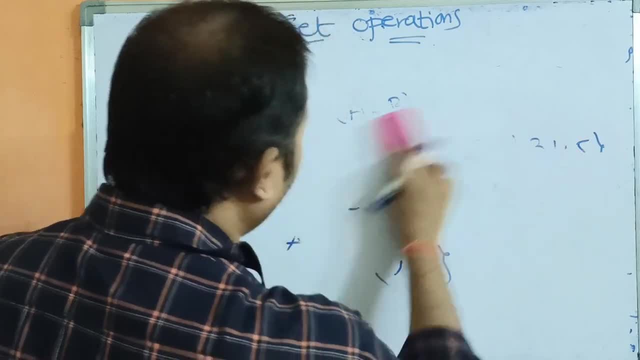 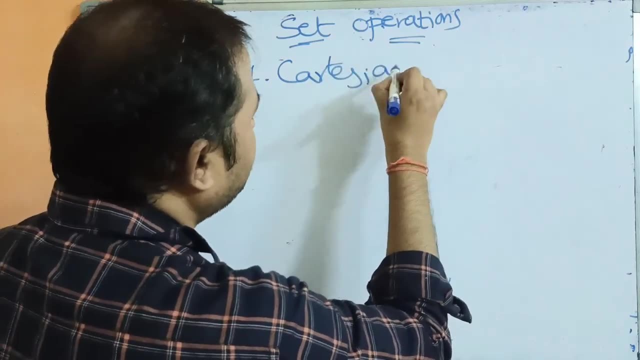 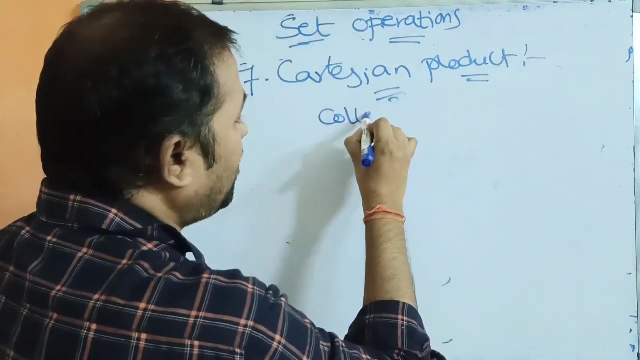 see the last operation. The last operation is Cartesian product. So the seventh operation is Cartesian product. So this is the last operation. So Cartesian product. So what is a Cartesian product? Cartesian product means it contains a set of ordered pairs, a collection of ordered pair. 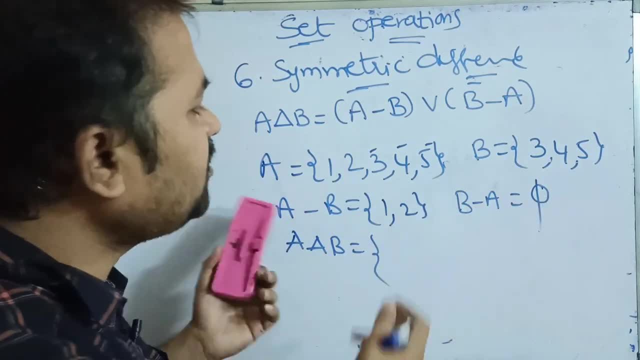 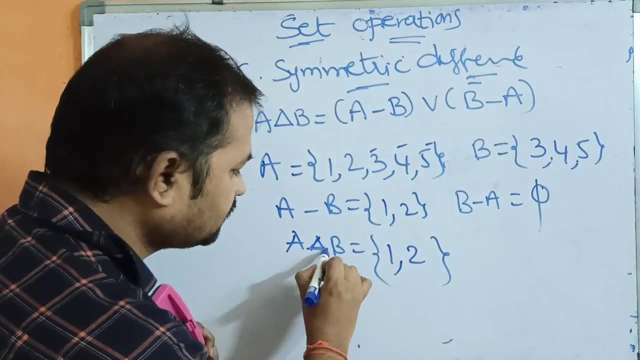 1 comma 2.. What is B minus A Pi? So 1 comma 2. union Pi means what? 1 comma 2.. 1 comma 2.. So this is the. In this way we can calculate the symmetric difference. 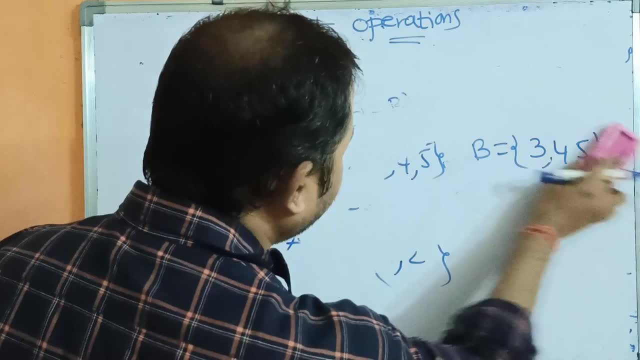 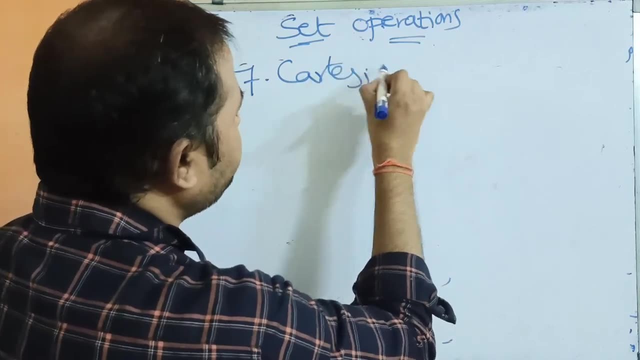 Now let us see the last operation. The last operation is Cartesian product. So the 7th operation is Cartesian product. So this is the last operation. So Cartesian product. So what is A Cartesian product? Cartesian product means it contains a set of ordered pairs. 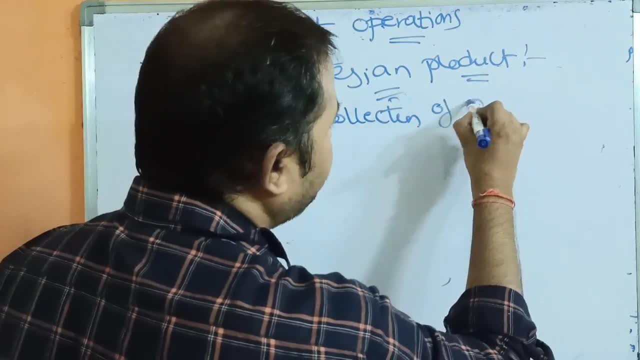 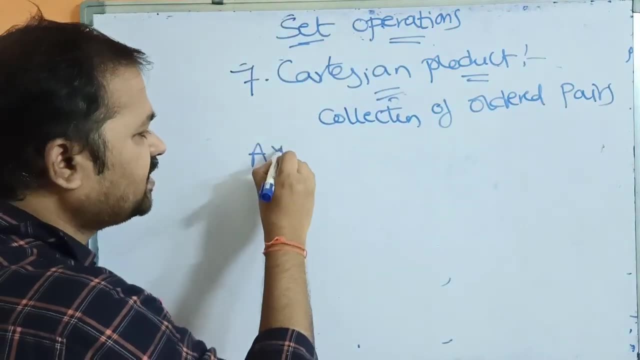 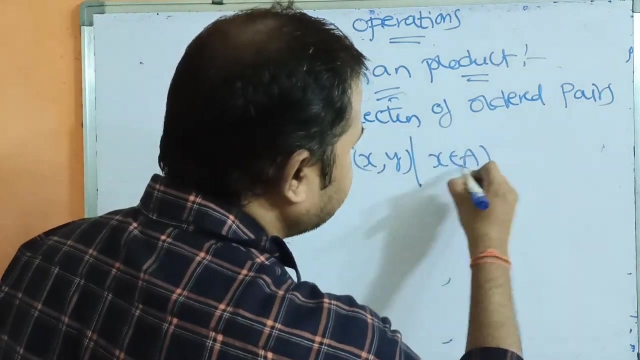 A collection of ordered pair. Collection of ordered pair. Ordered pairs- Pairs. Here Cartesian product is represented with the help of this cross mark, symbol A. cross B is equal to X, comma Y, such that X belongs to the first set and Y belongs to the second set. 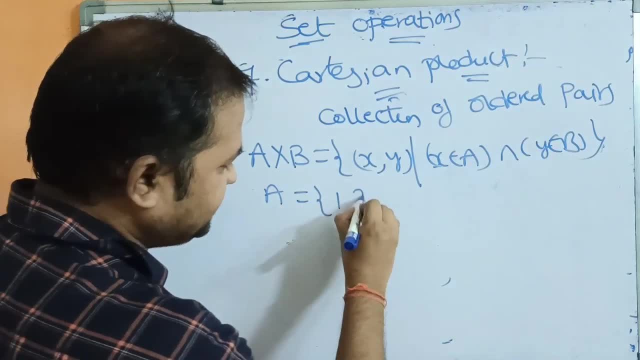 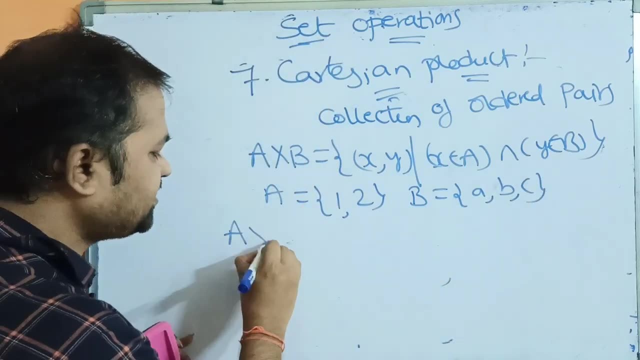 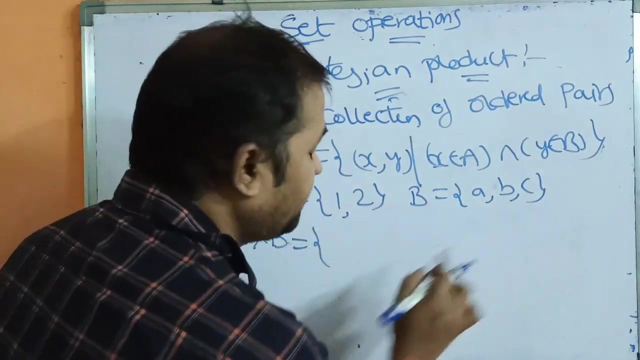 Okay, Let we have 2.. 2 sets like this: A is equal to 1 comma, 2.. B is equal to A comma B comma C. Then how to calculate Cartesian product A cross B. A cross B means we have to take every element from the A and form the ordered pair with every element of B. 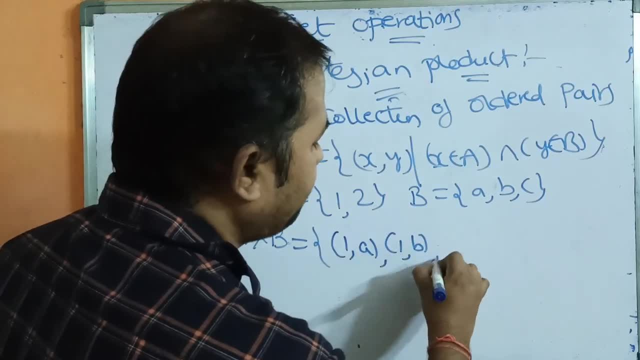 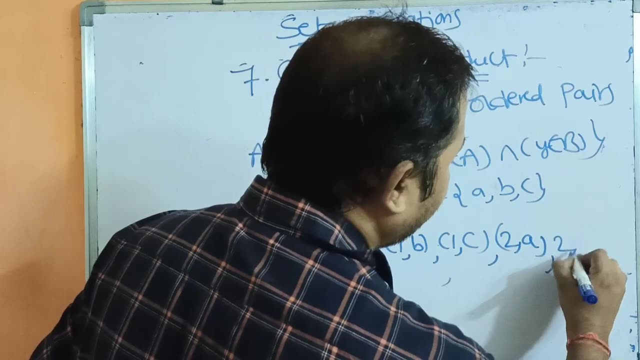 So we can write here as: 1 comma A, 1 comma B, 1 comma C. Now let us take the second element from the B and form the pair with every element of B, 2 comma C. So likewise we can calculate. 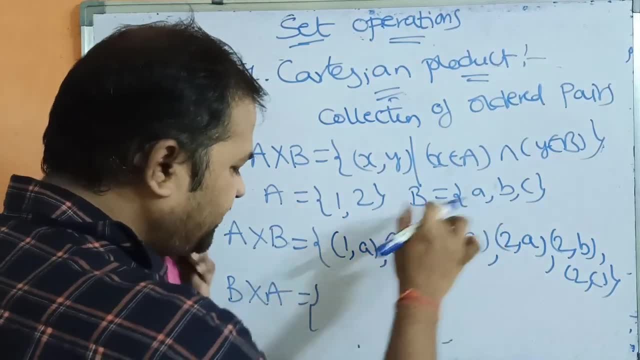 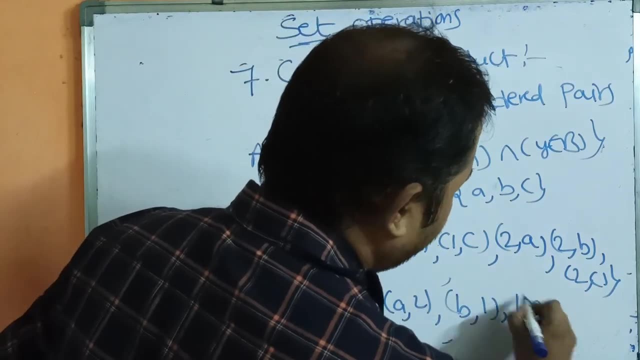 B cross A. B cross A means we can take the first element of A. So A comma 1,, A comma 2.. Next B comma: 1, comma, B comma 2.. Next C comma: 1, comma C comma 2.. 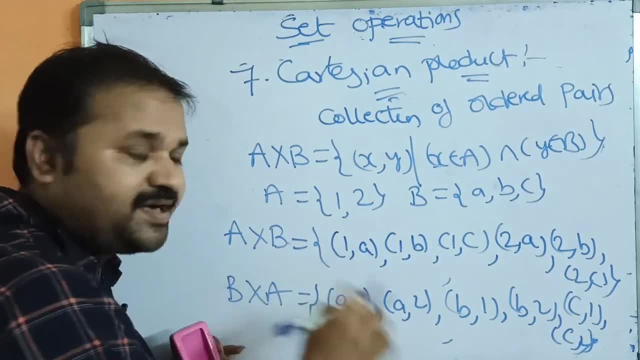 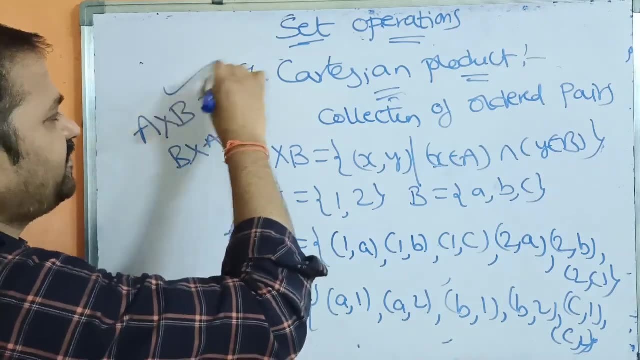 Here 1 comma A is entirely different from A comma 1. So we can say that A cross B is not equal to B cross A. So A cross B never equals to B cross A. So this is about various important 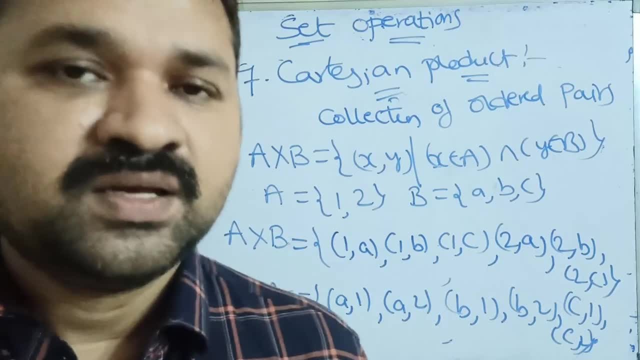 Important points regarding the set. So this is about sets.